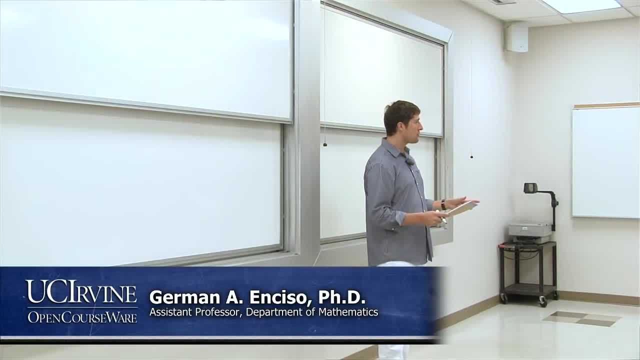 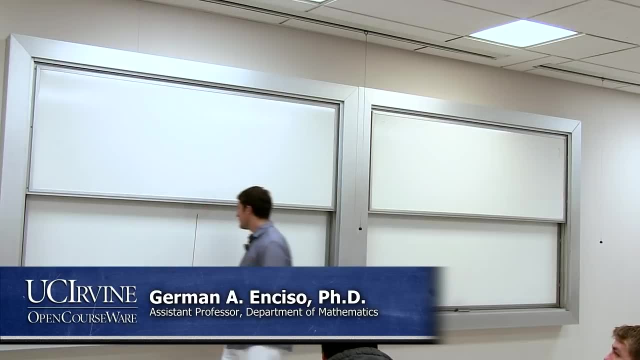 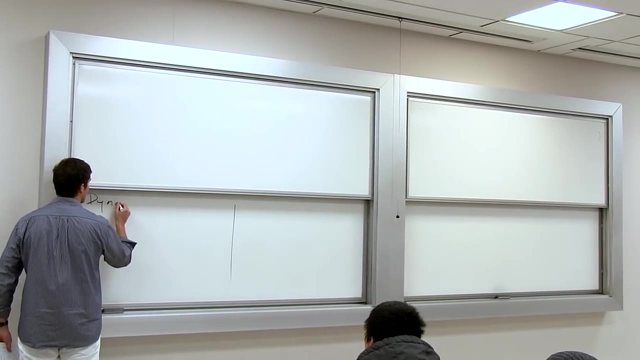 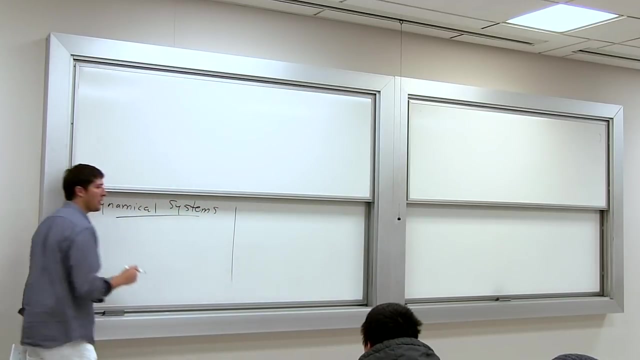 This is a mathematical modeling in biology course. We're going to talk about the main ideas for modeling problems in biology using mathematical systems, mathematical tools, and the main idea is the use of dynamical systems. Okay, and the basic idea of dynamical systems is to model concentrations, populations, etc. 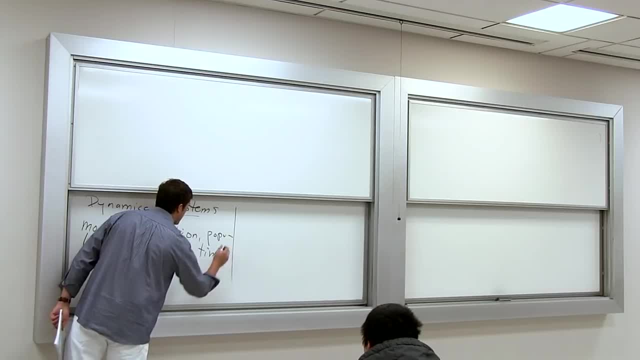 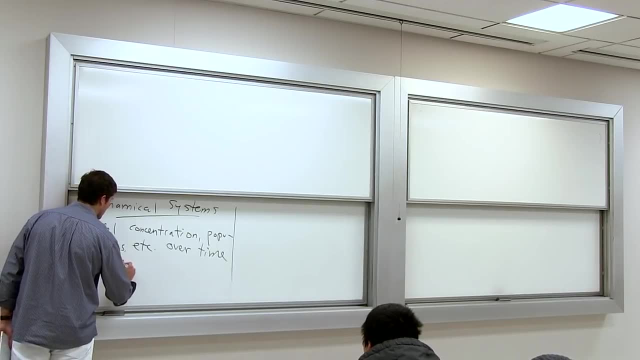 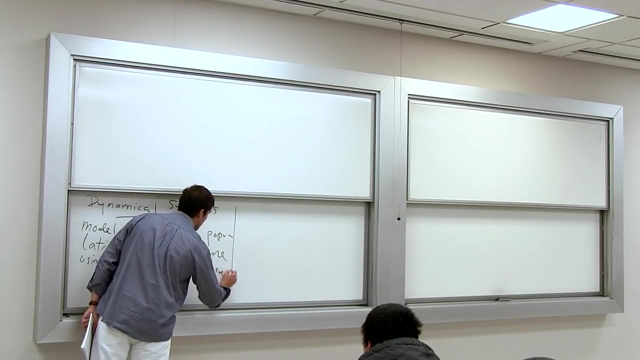 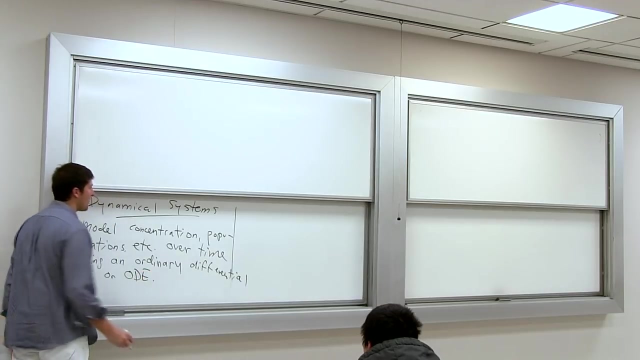 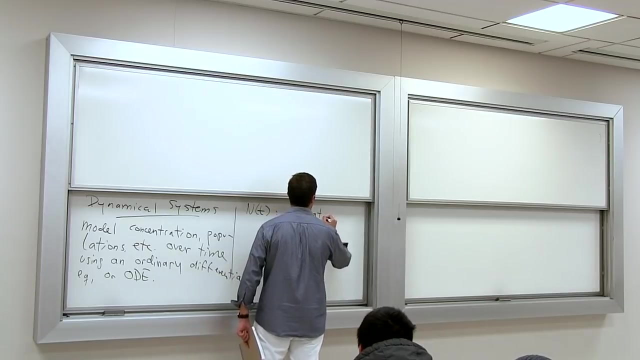 over time. okay, using a differential equation, ordinary differential equation or ODE. Okay, so the most simple ODE I can think of is the model of population. So suppose that N of t is the population of bacteria over time. 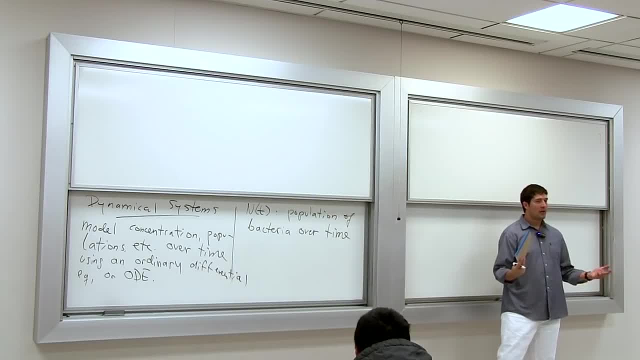 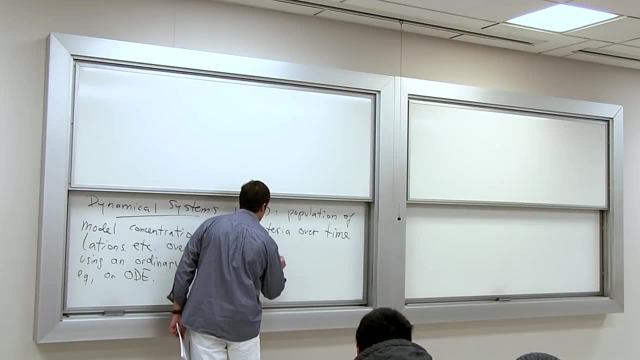 So you grab a bottle of bacteria- actually a bottle of sugar- and you put a bunch of bacteria in it and you let the whole thing evolve over time. 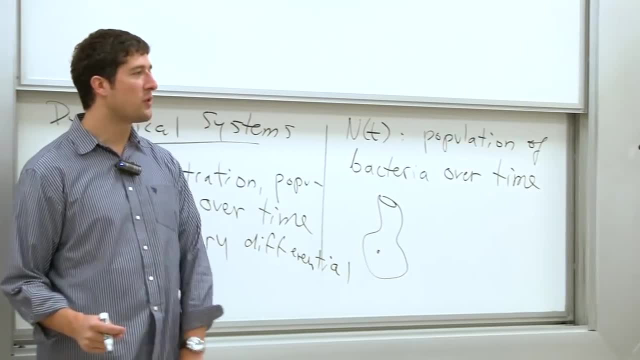 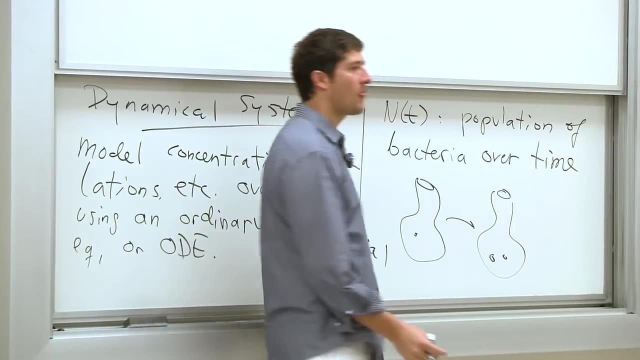 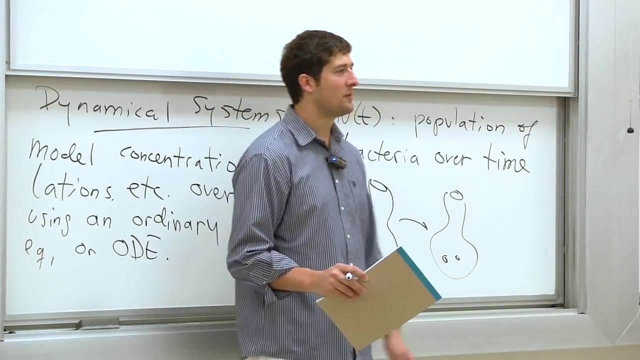 So here's a bottle. Let's say that you start with just one bacterium And after a while you wait and you get two bacteria. Now let's say that this time was I don't know two hours. So what happens after two hours? 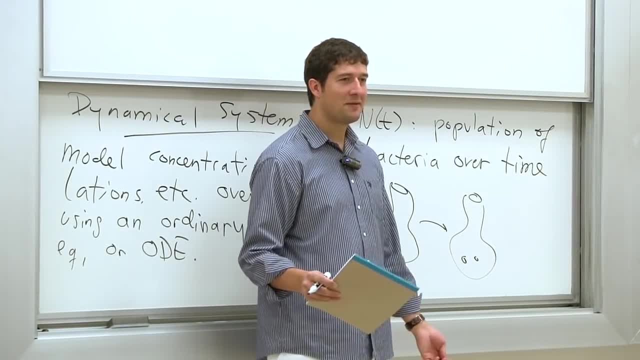 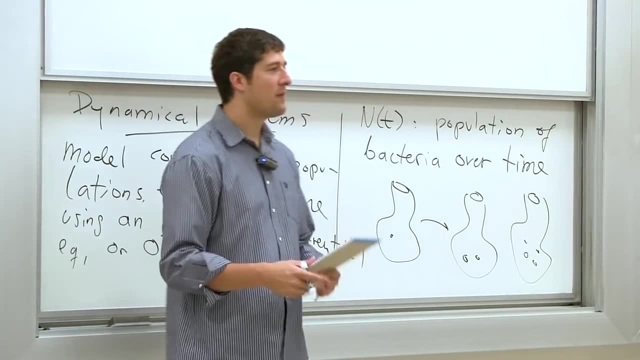 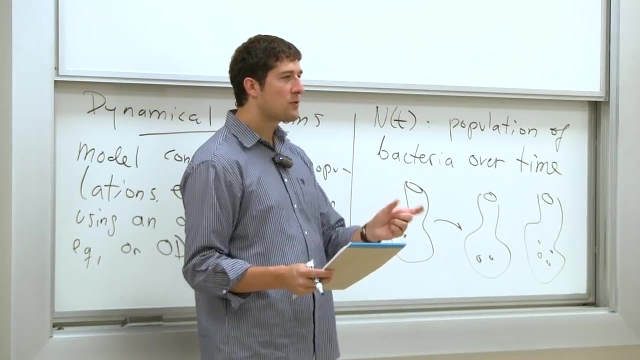 You get three, Or how many? Four, right, Okay, fine. So you get four bacteria after the same amount of time And the same thing over and over. So this growth is what we call exponential right. How do we capture this thing mathematically? 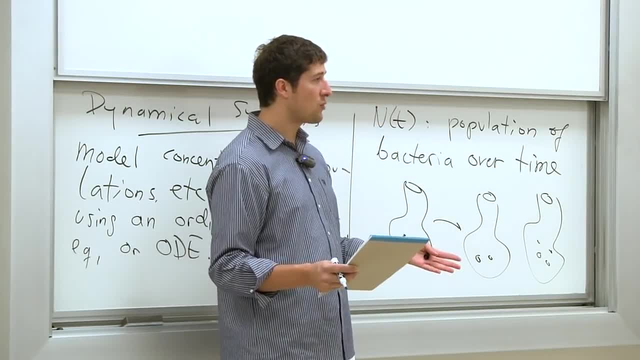 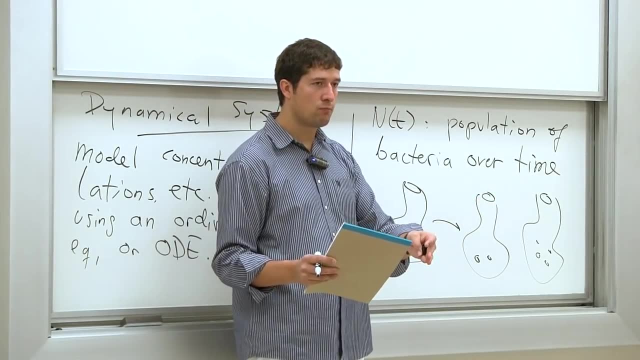 Well, one thing we could do is- and this is what's done in the whole course last quarter- is to assume that the number of bacteria is discrete And that there's also discrete amounts of time. After one amount of time, after two, three and four. 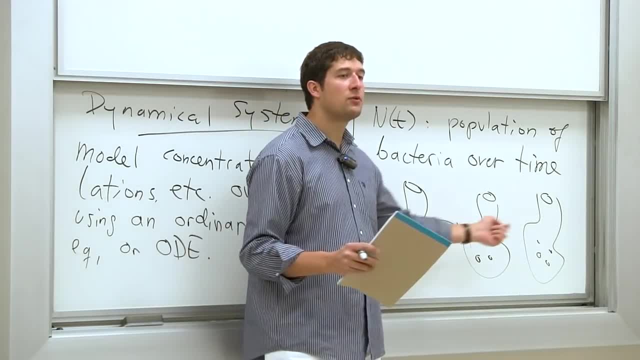 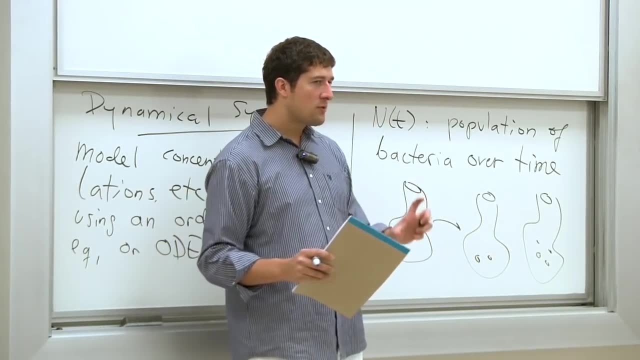 Now we're going to go one step beyond that. We're going to assume that the time is continuous. Time now is a continuous variable And the population is also a continuous variable. Mind you, that's already a simplification. We're assuming that the number of bacteria is a continuous variable. 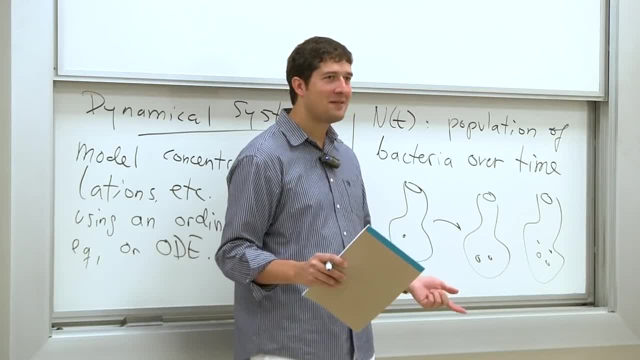 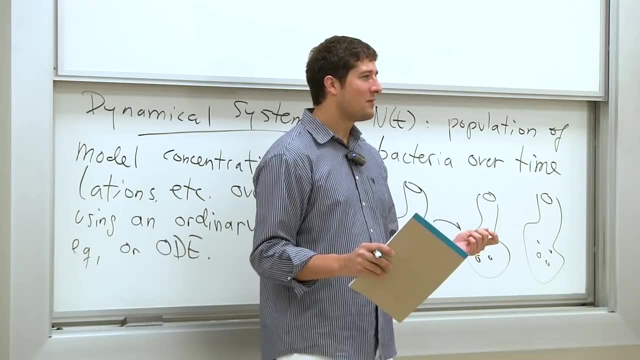 There's actually no such thing as 10.5 bacteria. right, You cannot talk about 10.5 bacteria, But we're assuming that the number of bacteria is a continuous number. Why do we do that? Why do we think we can get away with that? 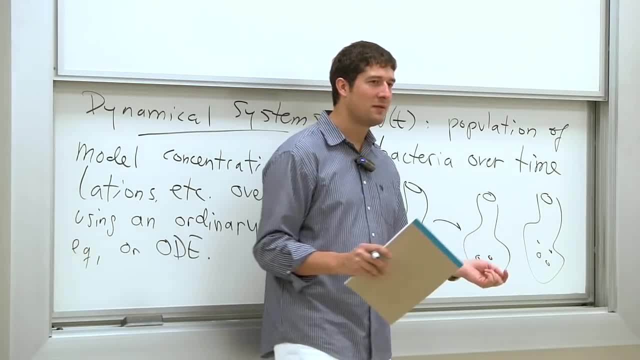 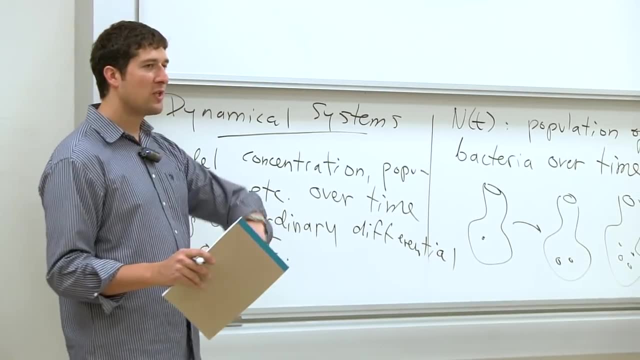 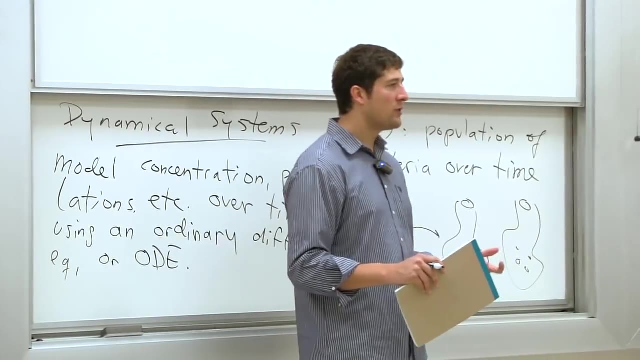 Sounds kind of a weird thing to assume that you can have 10.5 bacteria, right? Well, We do that, because otherwise we cannot write a differential equation. Differential equations usually involve continuous variables, First reason. Second reason is that the number of bacteria is usually so high- we're not talking 10 bacteria. 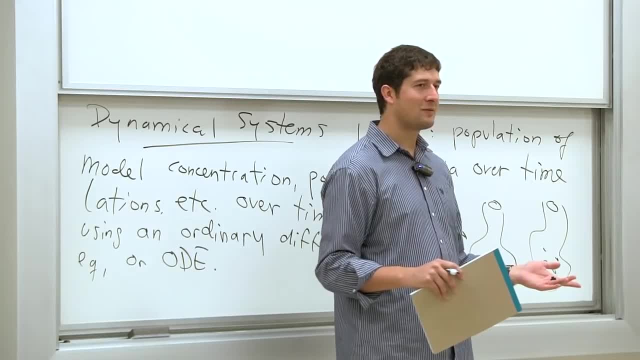 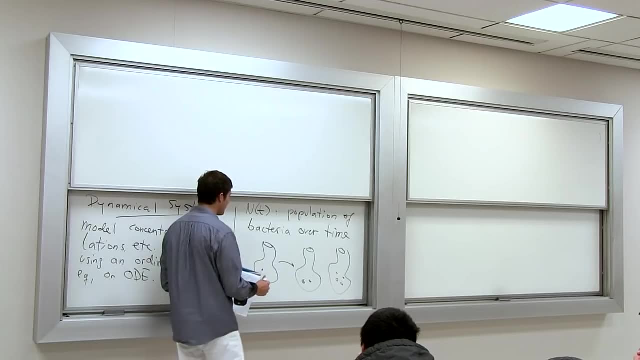 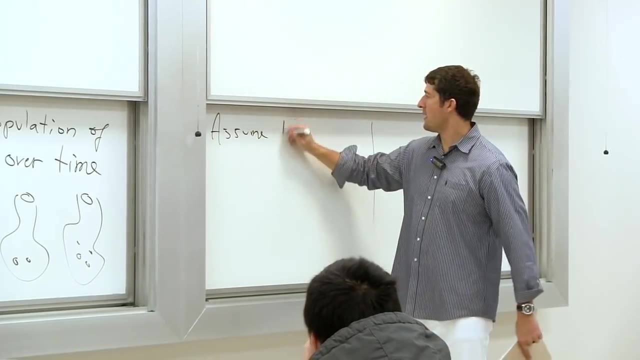 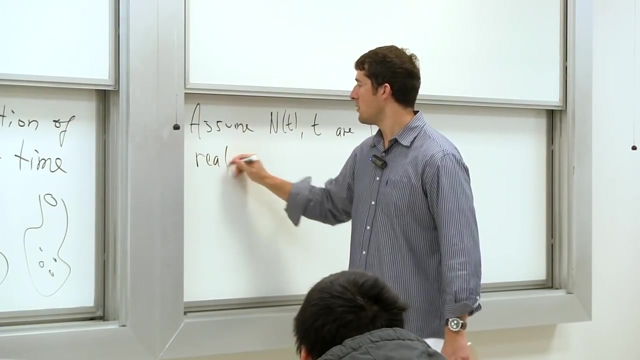 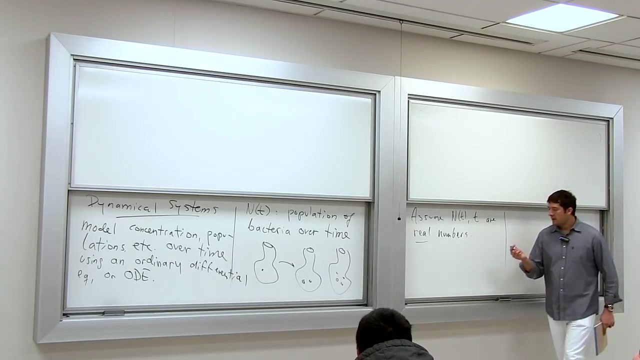 we're talking a million bacteria, that it doesn't really matter, right? So we're now going to assume that the population is continuous and time is continuous as well. So assume that N and time are real numbers. Okay, So now the differential equation I have in mind for this. maybe somebody can offer what. 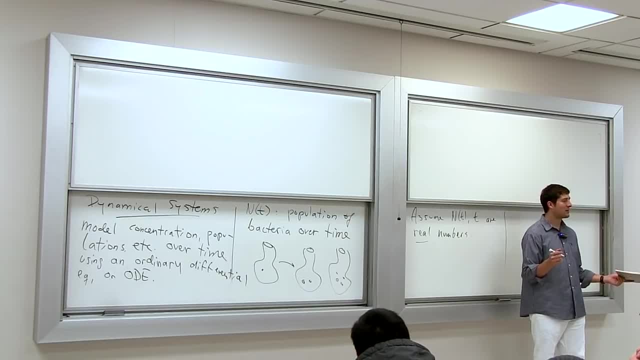 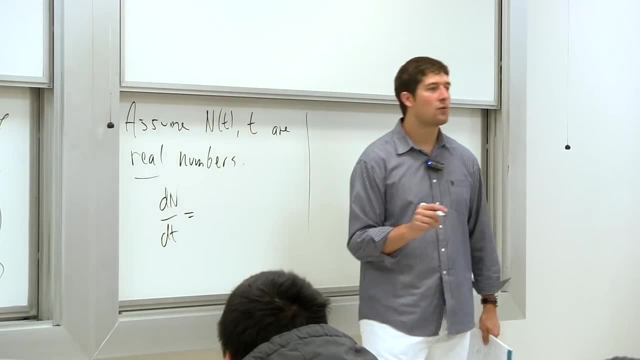 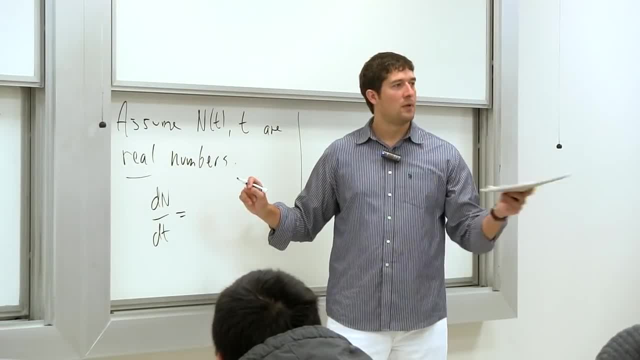 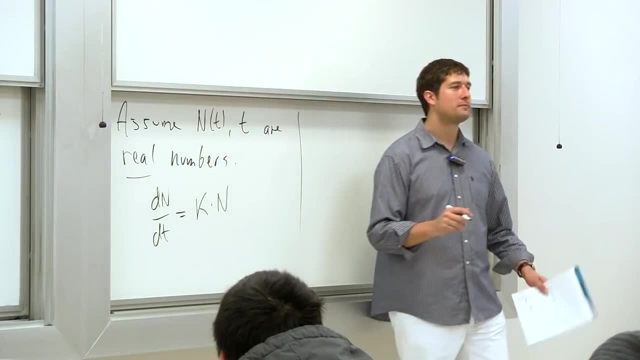 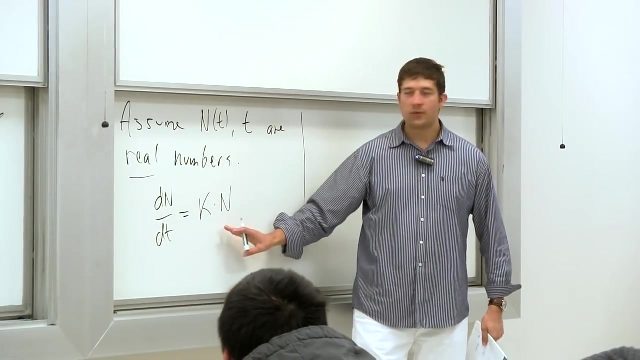 Lambda n or constant times n. We're going to call this constant k times n. Okay, What does this mean? Well, the rate of growth of bacteria is on the left hand side and on the right hand side we're saying constant times n. 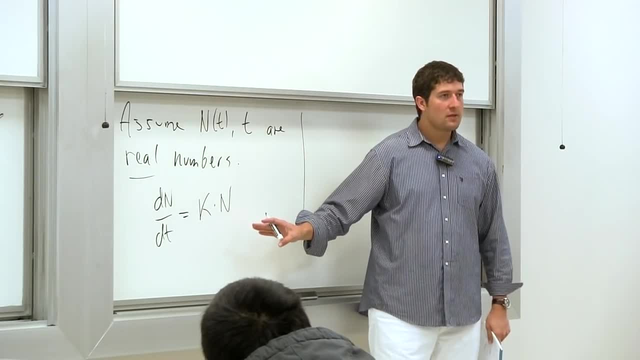 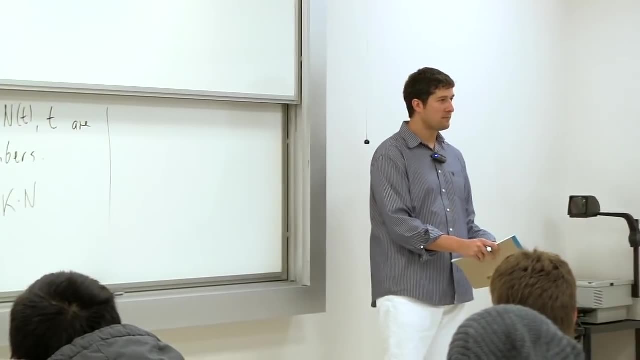 So, in particular, this means that if you start with, Let's say that you have a bottle with 1,000 bacteria over here, and over here you have a bottle with With 2,000 bacteria. So which of the two populations grows faster? 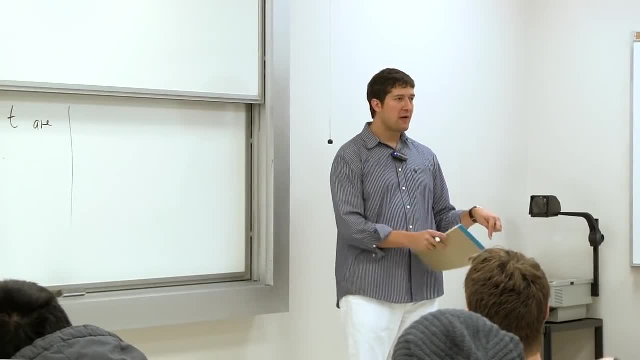 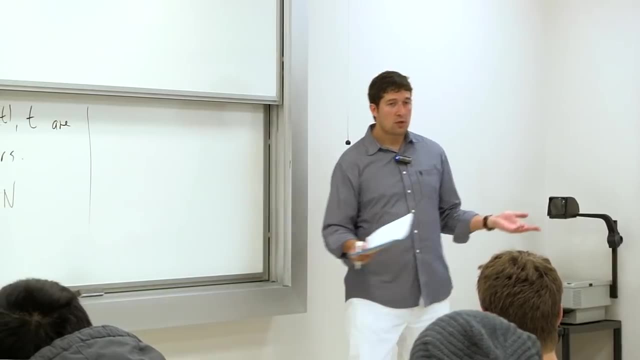 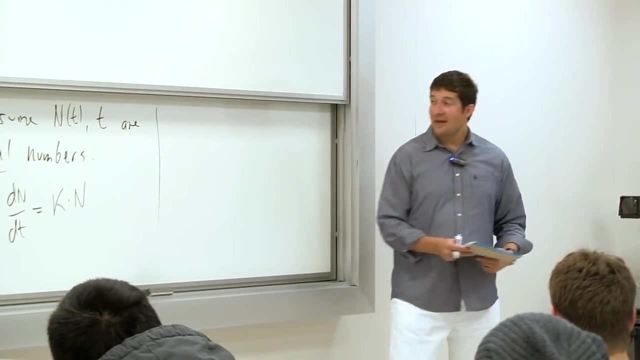 Of course this one right here. right? According to that equation, how much faster does this population grow than one with 2,000 bacteria? Two times faster, right? So if you start with 1,000 bacteria, you grow half as fast as if you start with 2,000 bacteria. 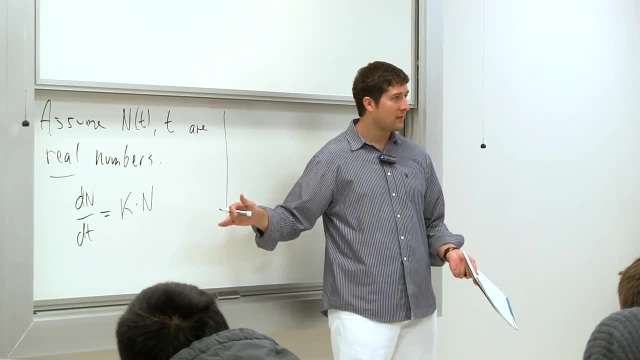 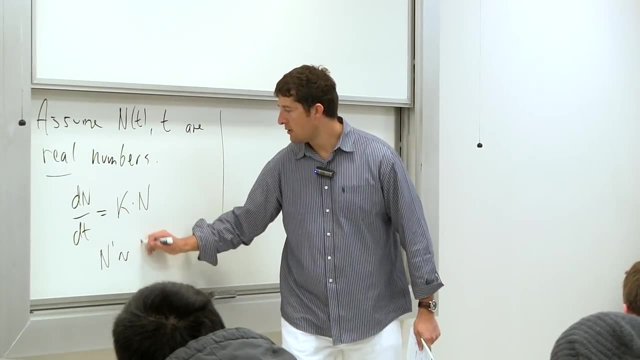 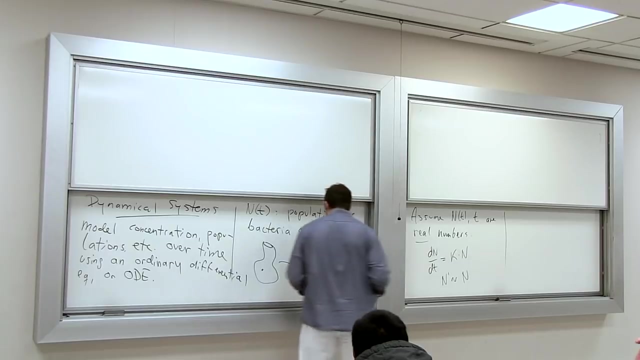 That is really what the equation says. It doesn't say anything other than that. It says that the, That, the, That, the, The rate of growth is proportional to the population. okay, That is this idea that if you start with two bacteria, you grow twice as fast than if you. 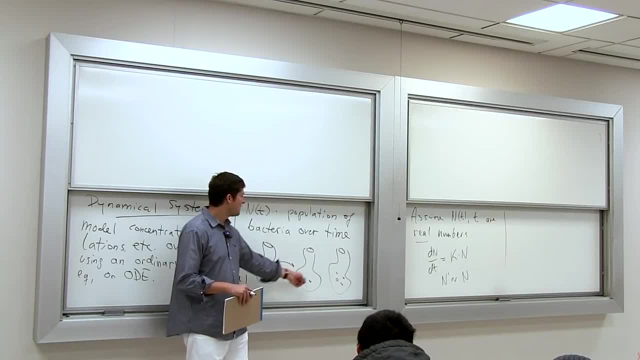 start with one. It's basically encoding this idea that you, That the bacteria, don't care how many other bacteria are around, as long as each of them has enough sugar to grow. you know they grow at the same rate on their own, you know, depending. 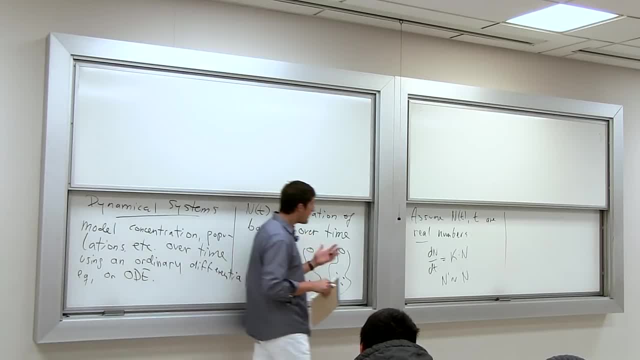 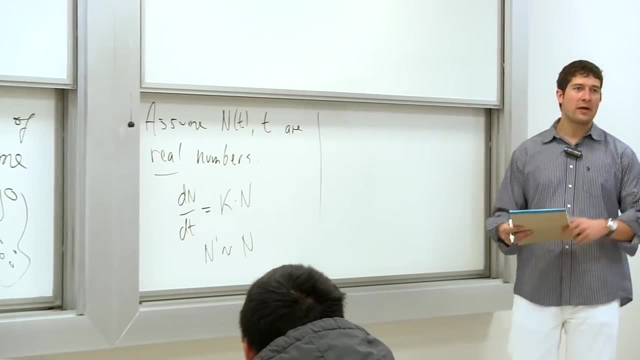 on how many other bacteria are in the same bottle. Okay, So that already is a big modeling assumption and it's all encoded in this equation. This is what we call an ordinary differential equation. I know you guys probably all know this, but let me just state it for 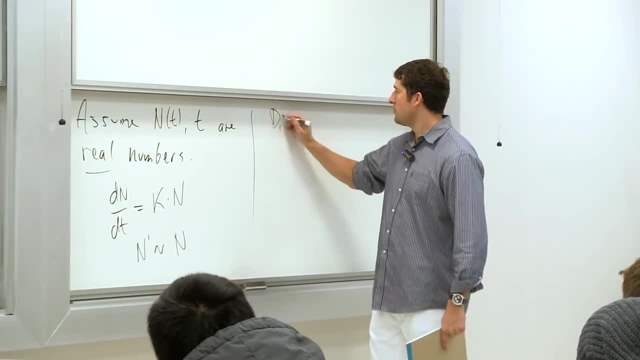 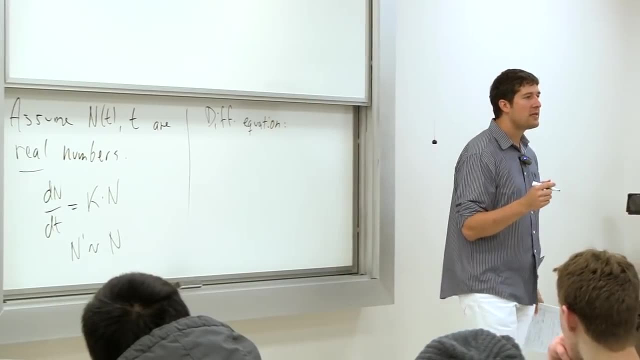 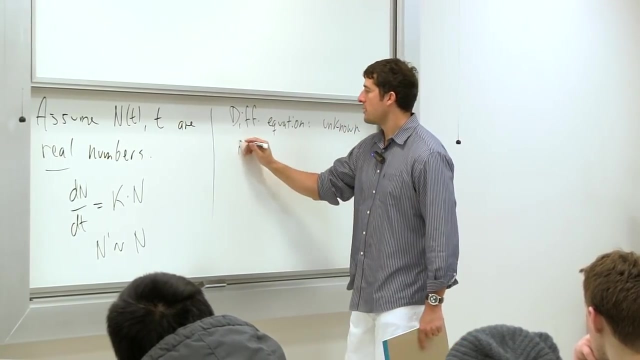 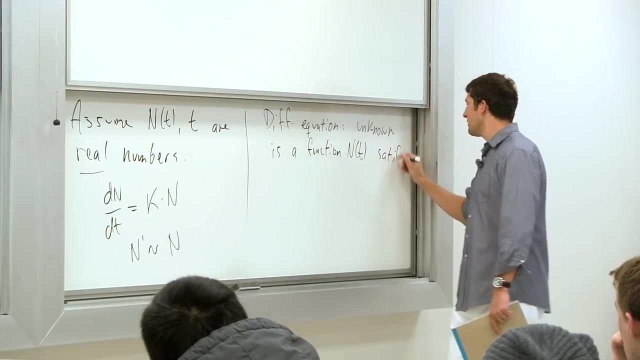 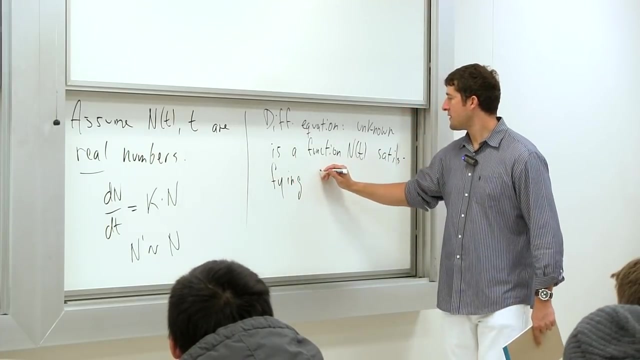 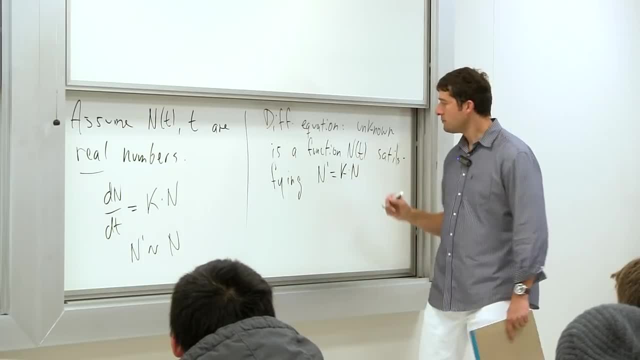 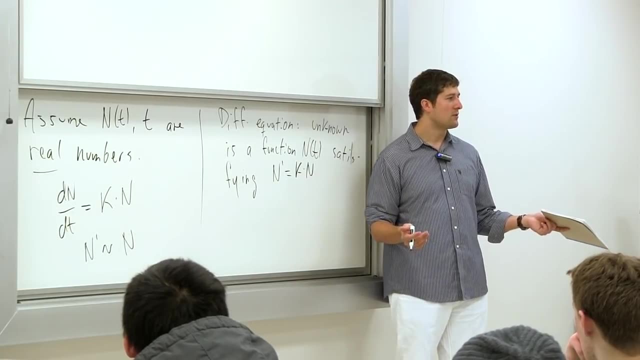 In this case, n prime equals k times n. Okay, So does anybody want to venture a function that satisfies this equation? Pretty easy, actually, right. So what do you think? Or what do you think Either the, Either the, Anything. 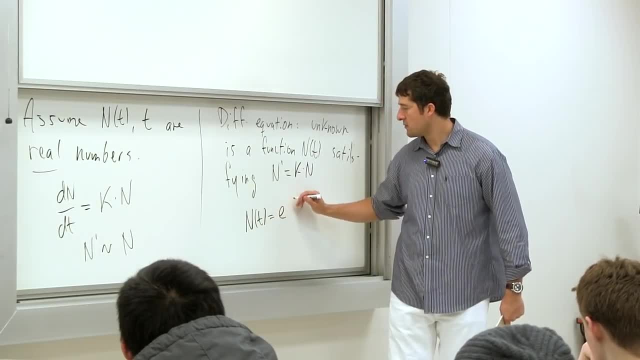 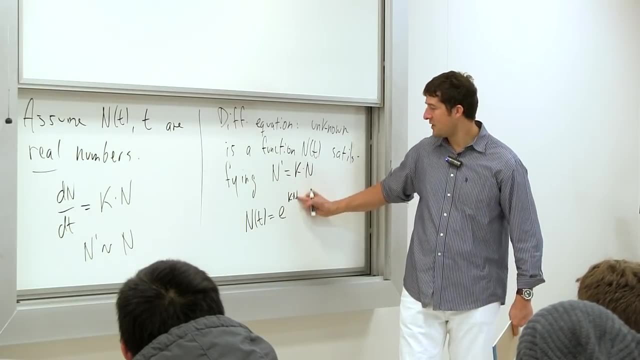 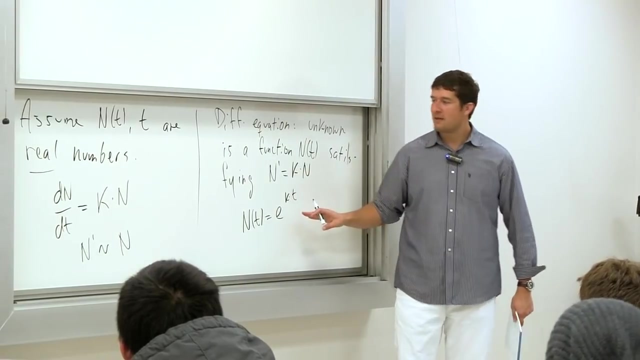 That's right, ernaft equals e to the k times. Well, times n, Times t, Times t right, Times t. Okay, So let's check that this function satisfies this equation. How do we, How do we do that? 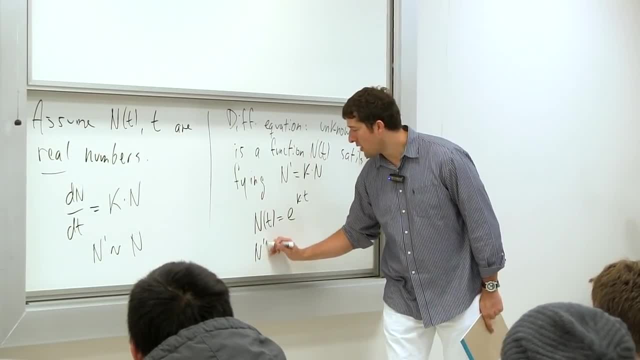 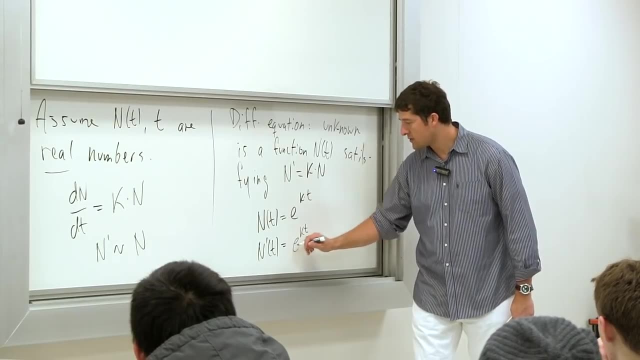 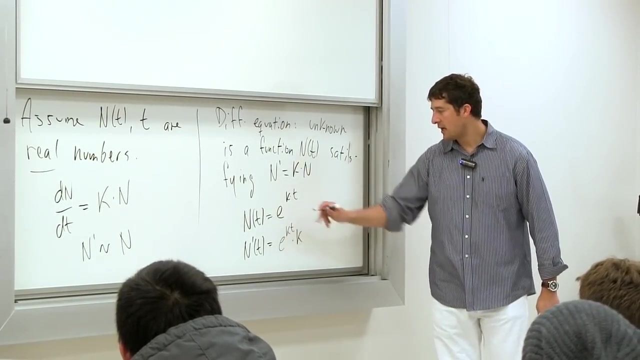 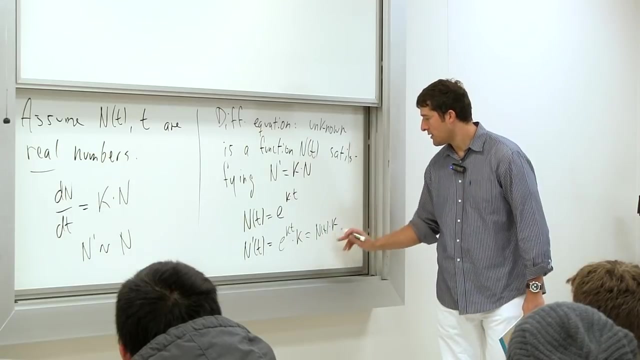 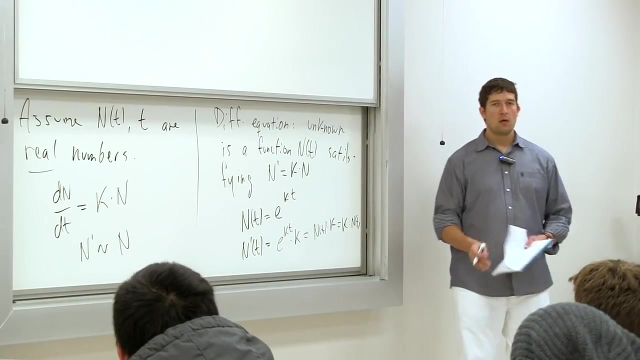 We just plug it in, right, Okay? So n prime of t is equal to equal to e to the kt times k, using the chain rule right, And because e to the kt is n, this is equal to n times k, which is just k times n. Okay, Is this the only function? 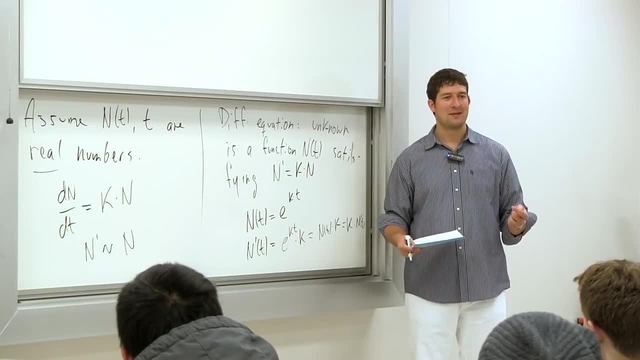 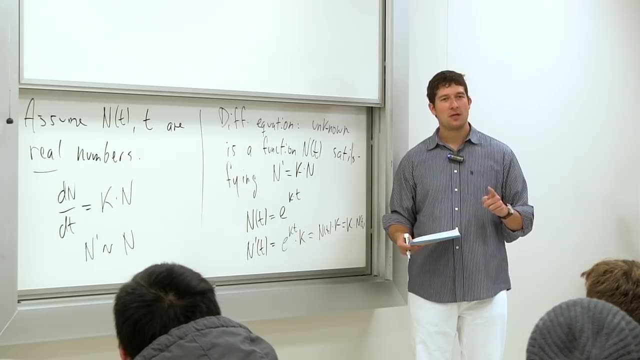 that satisfies that equation, or is there any other one? What do you think? Sine of kt? No, I don't think sine of kt works because the derivative is cosine right. Yes, Sine of a constant times e to the kt. 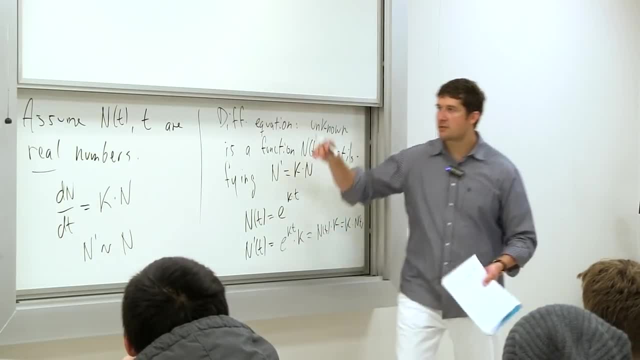 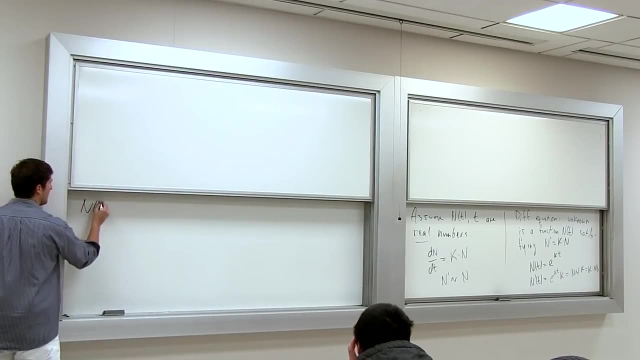 Yeah, exactly, You can actually multiply these by a constant right. So let's do this real quick. If n of t is a to the kt times k times n, what does that mean? So if n of t is a to the kt times e to the kt, what does that mean? 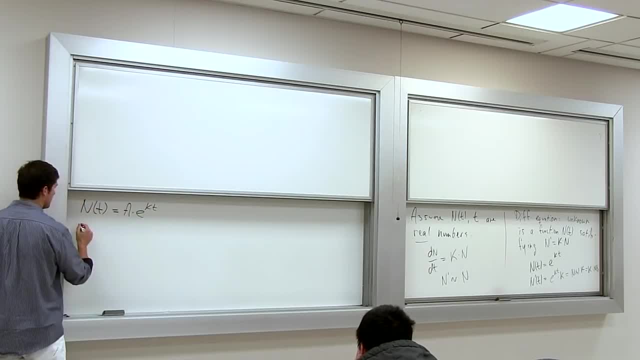 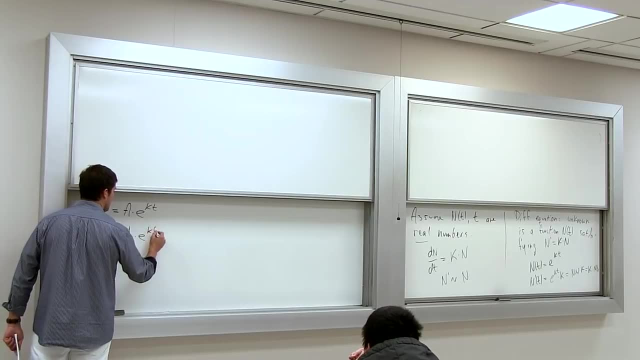 So if n of t is a to the kt, times e to the kt, what does that mean? So if n of t is a to the kt, times e to the kt, then n prime of t is equal to a times e to the kt times, the derivative, which is k. okay, 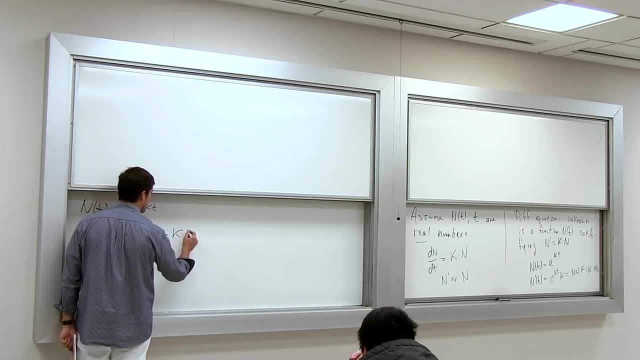 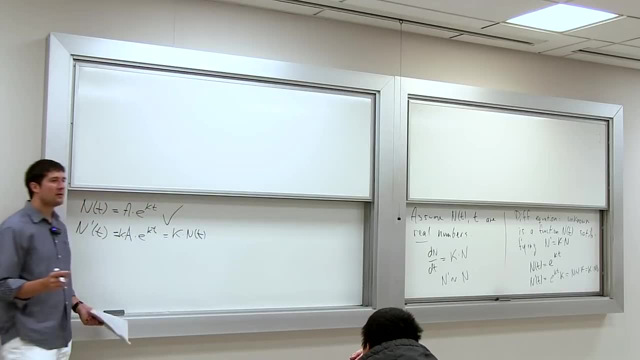 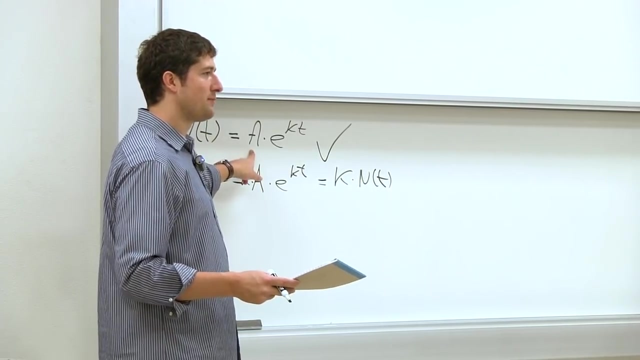 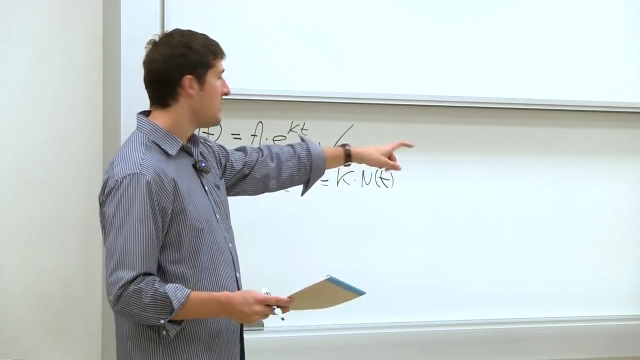 And this is n, of course, then this is equal to k times n of t. Okay, So it also satisfies the ODE In practice. there's actually a whole family of solutions, Okay, And you can also prove- but that's actually harder to prove- that every solution of the ODE is of this form. 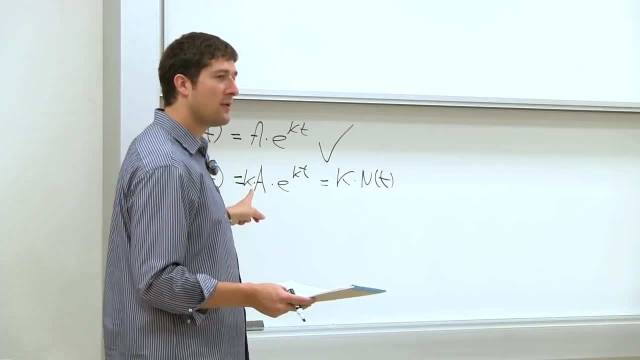 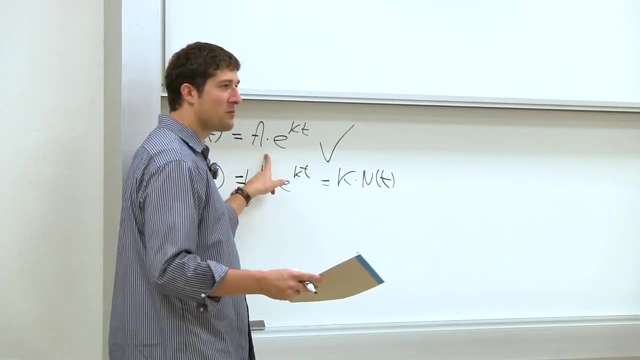 Okay, That's not so easy. We actually have not done that. We just proved that there's a whole family of solutions that satisfy the equation, But we didn't prove that. all solutions look like this: But you can also prove that, Okay, So the solutions: 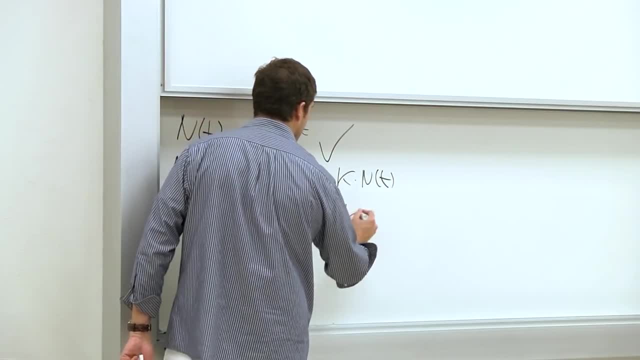 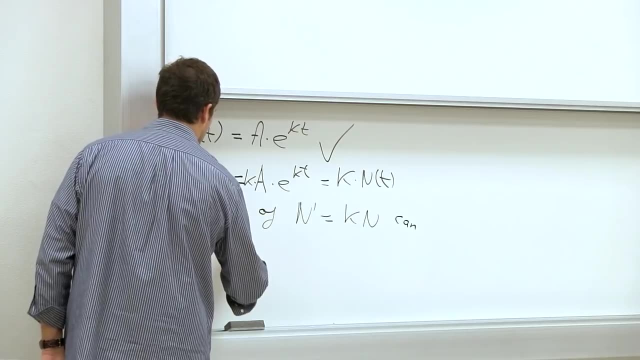 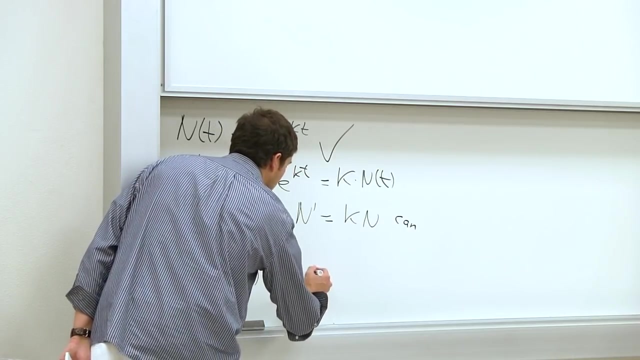 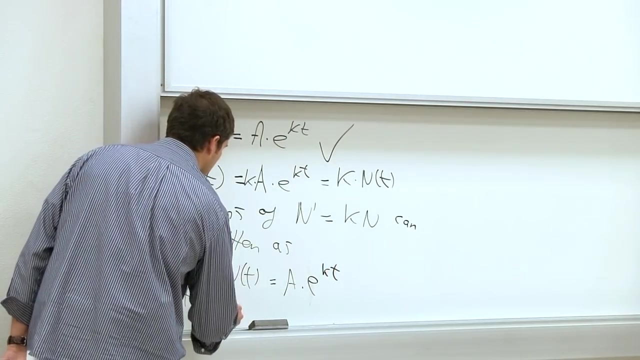 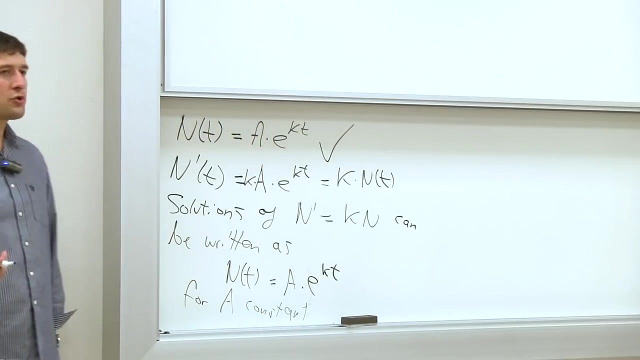 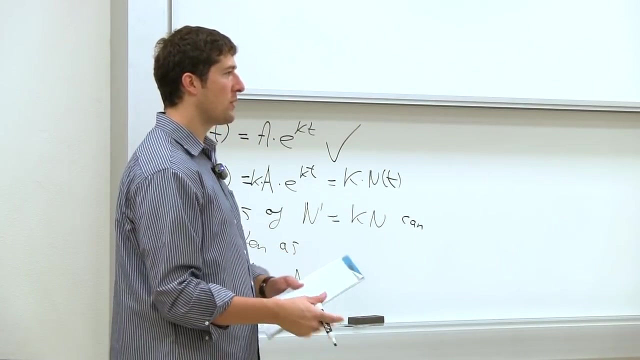 of the ODE n prime equals k times n can be written as as: n of t equals a times e to the kt for a constant. Okay, Now, usually we're we provide what's called an initial condition. Okay, The initial condition is the original population, with the population at time zero. 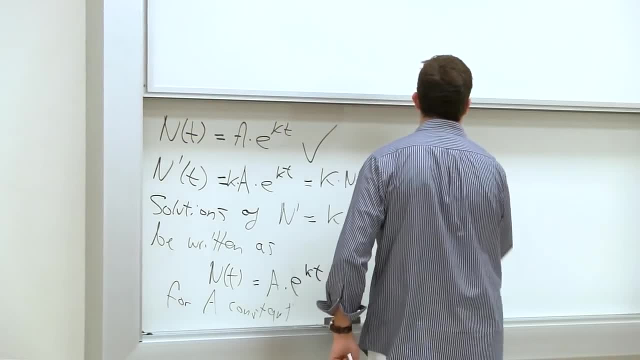 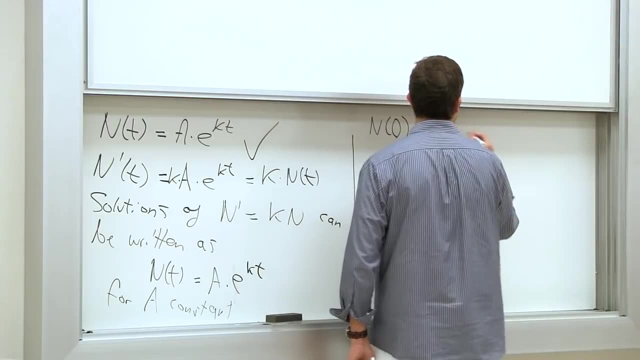 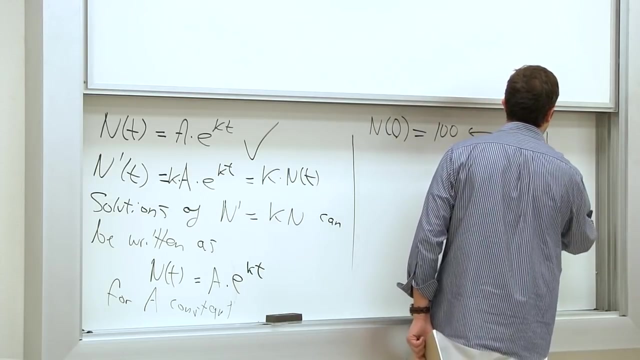 or the population at time, ten or whatever. So, for example, n of zero equals to a hundred. We call this the initial condition, And the initial condition can be used to figure out. 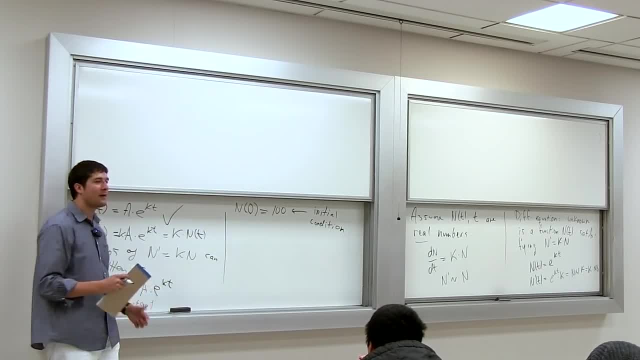 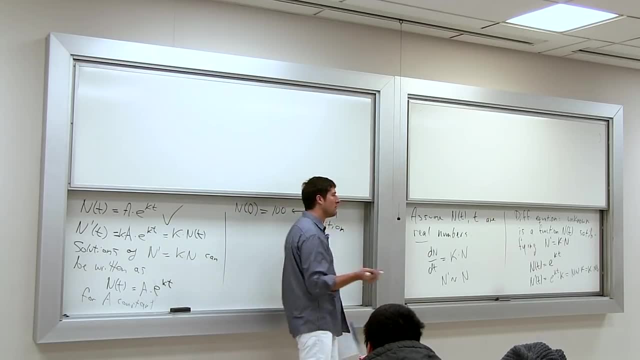 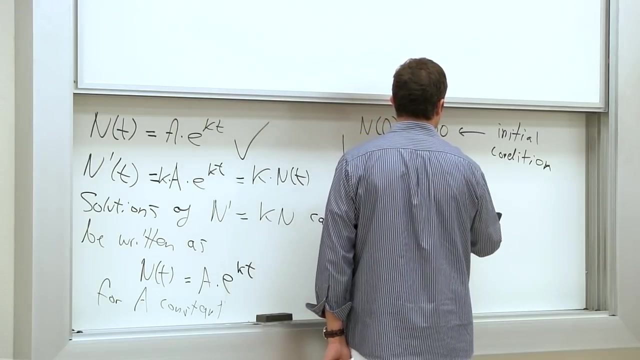 out the constant a. okay, So if we're given n of 0 is equal to 100,, then how can we figure out a? Well, we just plug it in right. So n of 0 is equal to a times e to the k times. 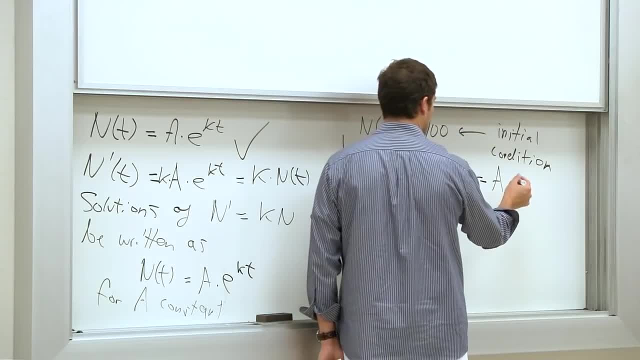 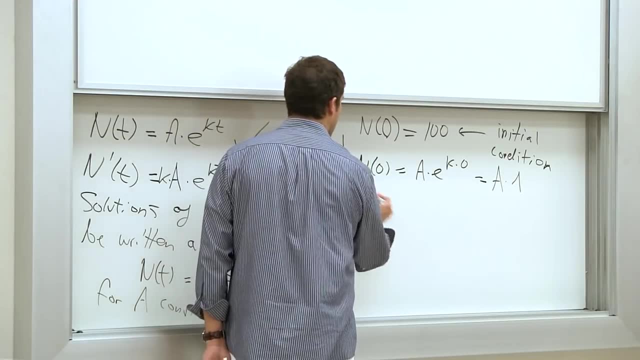 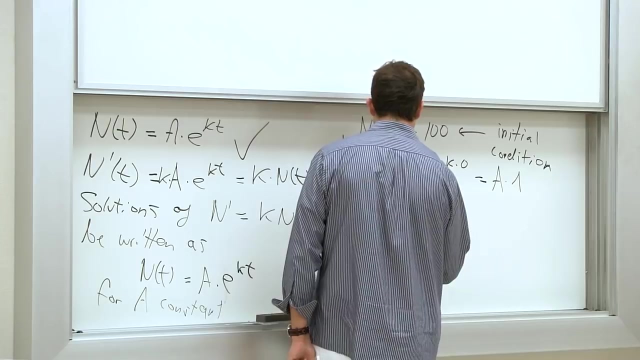 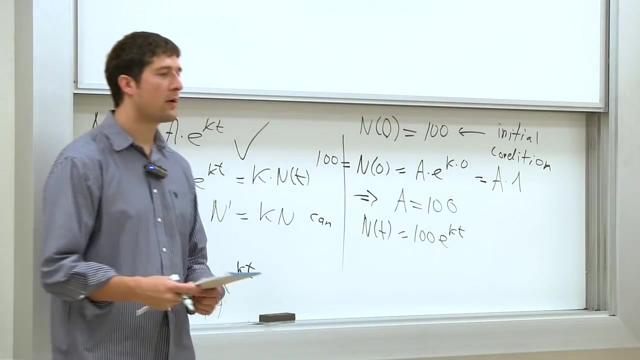 0,, which is equal to a times 1.. On the other hand, n of 0 is equal to 100,. okay, That means that a is equal to 100, and that n of t is equal to 100. e to the kt. Okay, I know for. 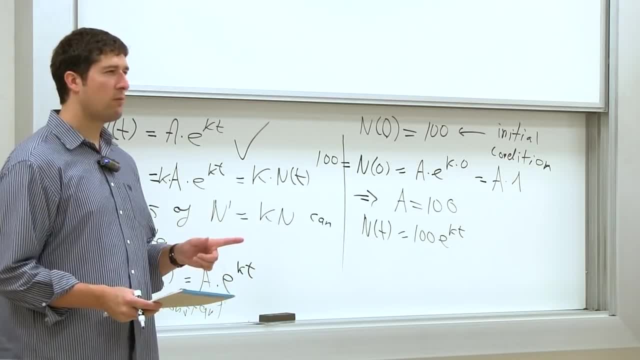 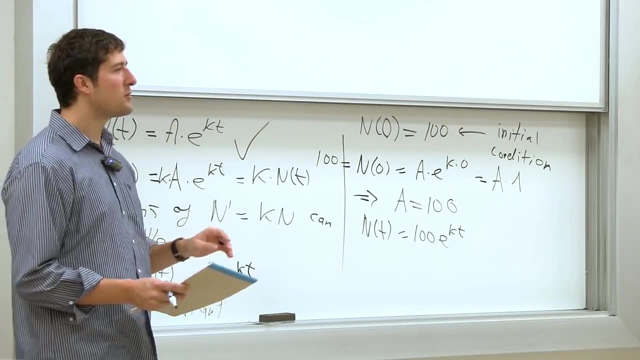 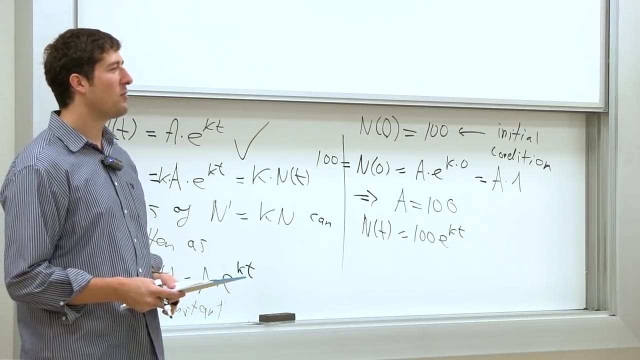 many of you guys. this is all very basic, although let me make sure you guys are all in second year. Third year, Third year: Okay, who's in second year? Second year is a sophomore right. Sophomore, No sophomores. Okay, what about juniors? Okay, what about seniors? What about? 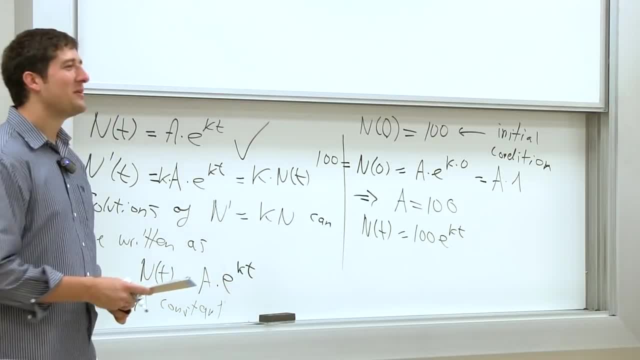 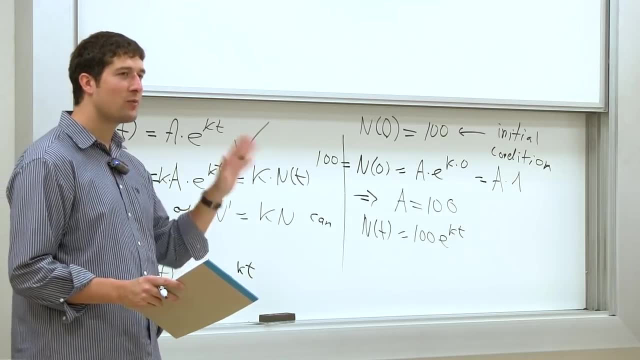 retired people One: okay, All right, okay, good. So all right, fine, Because you know, this course really has very basic prerequisites. so I want to make sure that people who are taking this course but did not take any more advanced course like Math 13 or something, 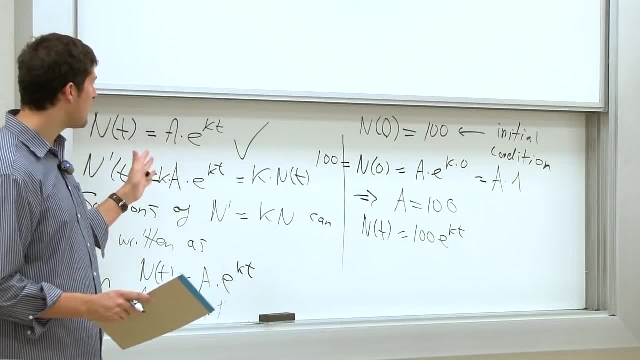 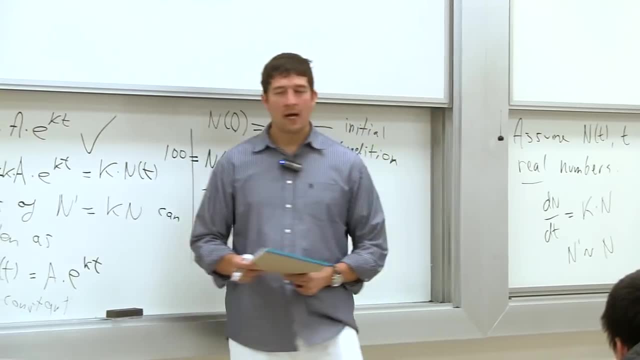 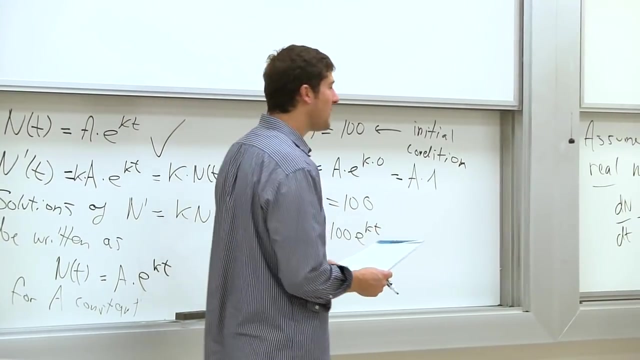 like that are missing out. So I want to make sure this is very basic stuff, but I wanted to say it. okay, We're going to make this a little more complicated now and assume the following: Actually, before I do that, let me ask you: what about the half-life? I'm sorry, not the half-life, The 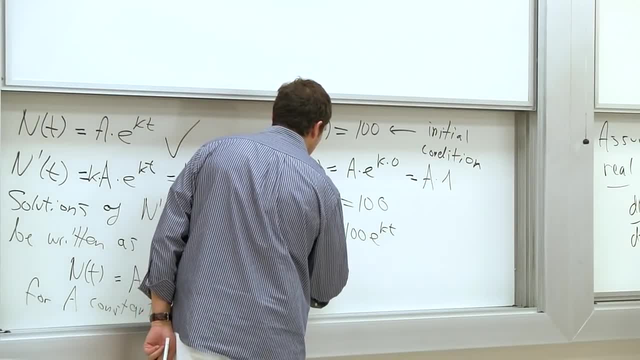 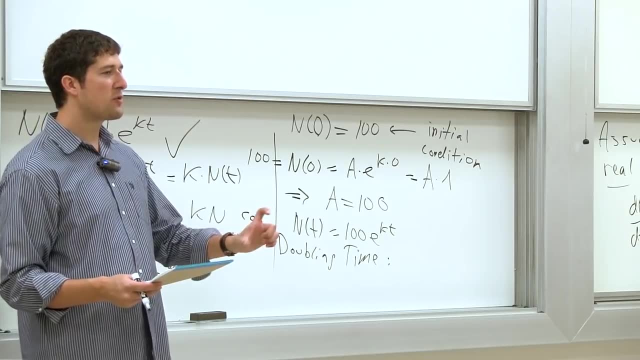 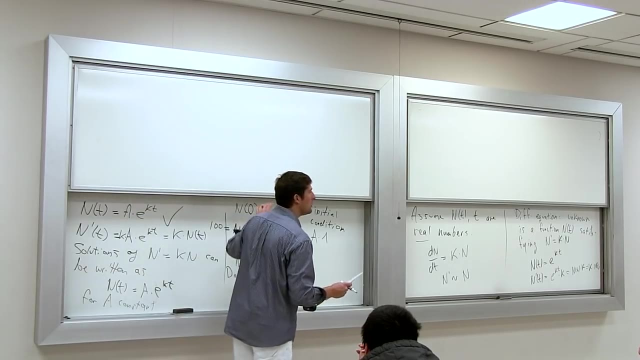 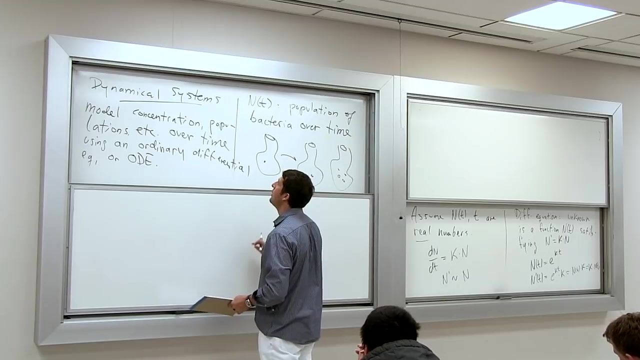 doubling time of the bacteria. If I have an equation like that, how do I know how long it takes for the bacteria to double in population? Fantastic, Right, Okay, That's just one more question. Yes, double the initial condition and find T. So let me write that here. 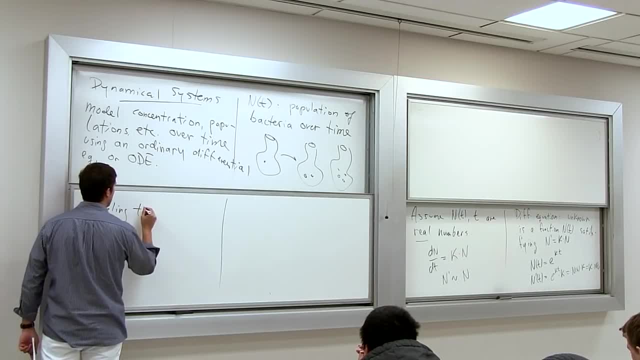 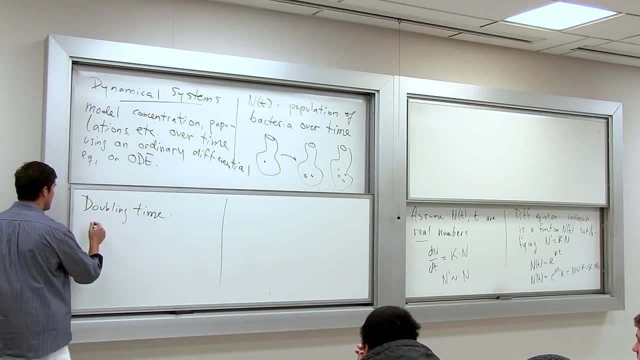 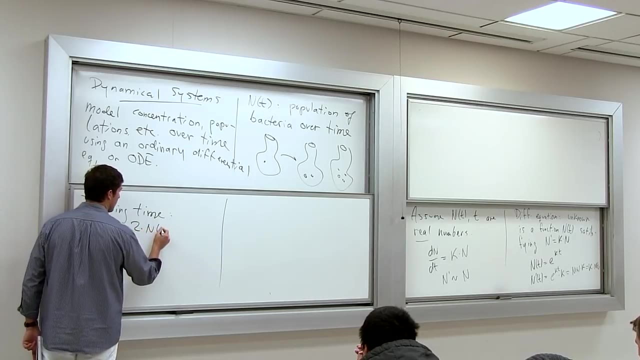 So doubling time. So this is the time that it takes for the bacteria to double, of course. So suppose that N of T zero is equal to two times N of zero. okay, We want to find T zero such that this condition is satisfied. 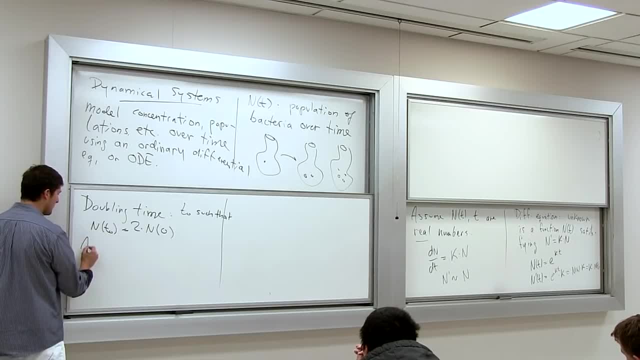 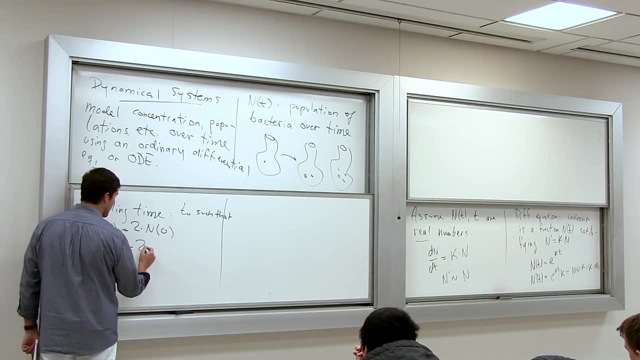 Well, we know the equation for N of T: right N of T is equal to A times E to the K T. in this case, K T zero is equal to two times N of T. right N of T is equal to A times E to the K times zero. 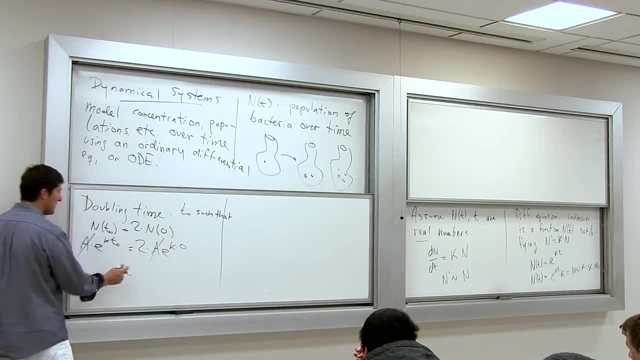 So that means that I can cancel out the A on both sides and this, of course, is equal to one, and I get E to the K, T zero is equal to two. okay, And I would like to solve for T zero. so I'm going to take the logarithm on both sides. 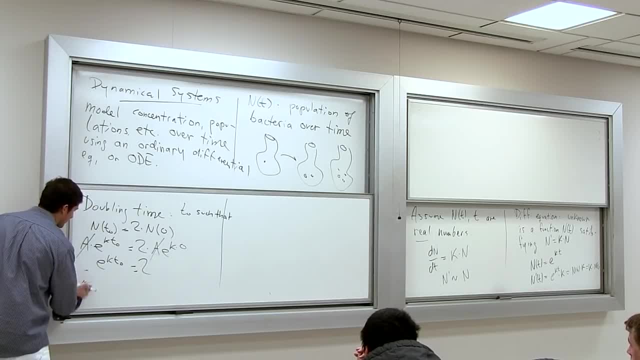 and I get. well, I take the logarithm on both sides. So on this side I get K times T zero is log two and that means that T zero is equal to log two over K. Okay, now back to the modeling. 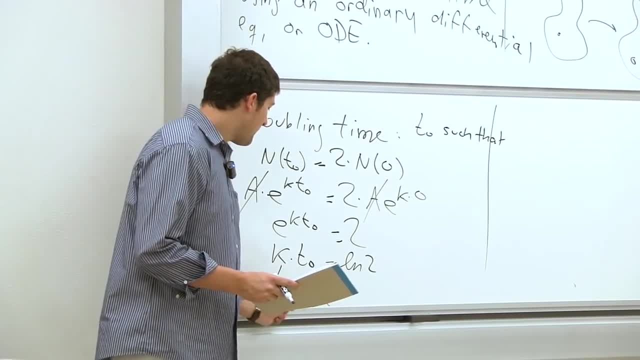 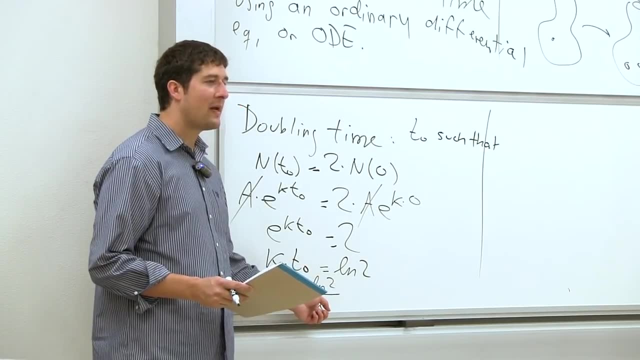 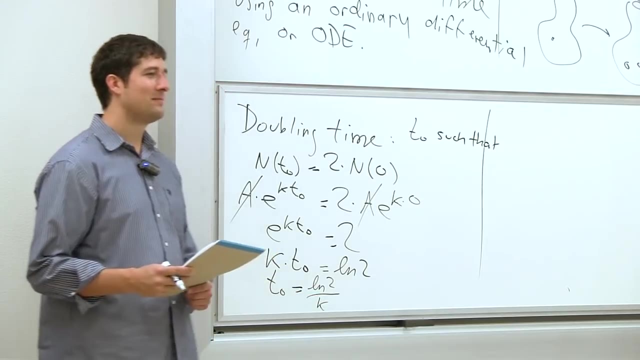 Remember we're now thinking about modeling problems. So the T zero has units of time, right, minutes, hours, whatever. So what would be the unit for K? Did you ever think about the units for this constant? It's one over seconds or one over minutes or whatever. 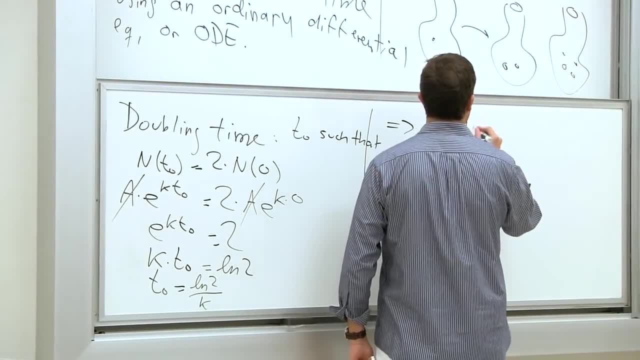 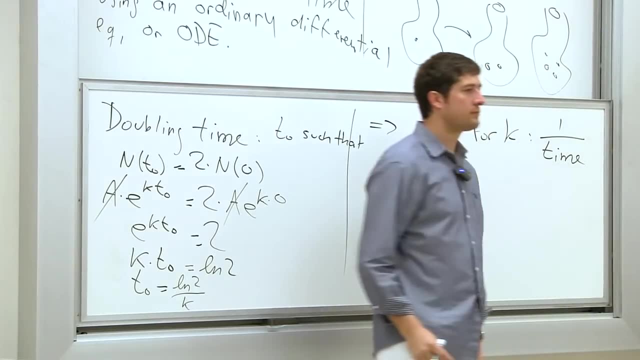 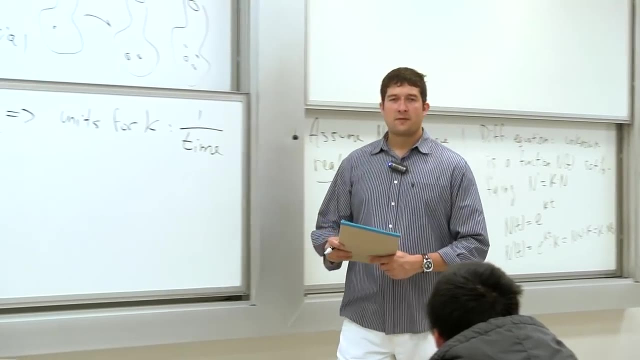 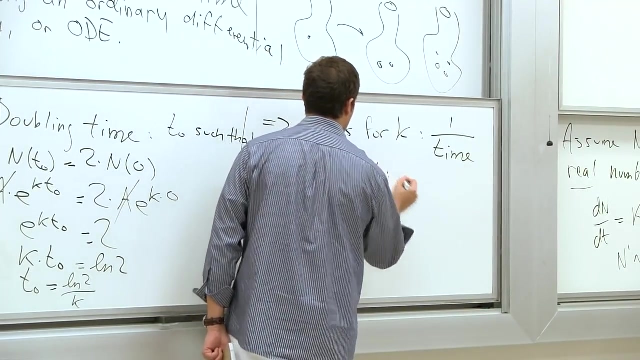 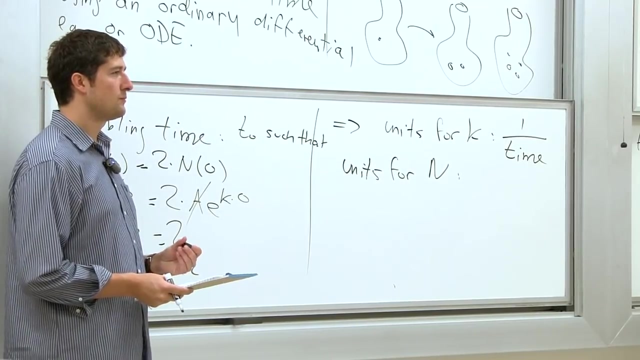 So that means that the units for K are one over time. okay, which is an interesting thing. What are the units for N? Now that we're talking about units, What do you think? N is the population right? Exactly Could be the number of bacteria. 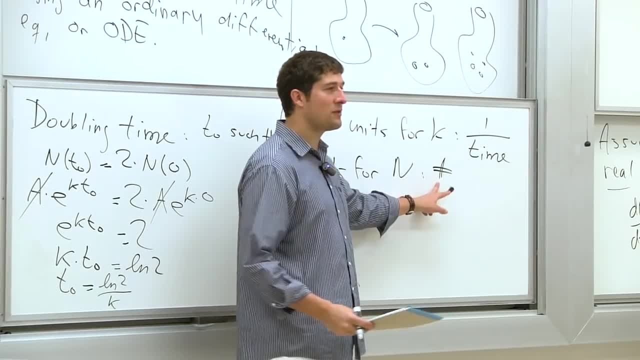 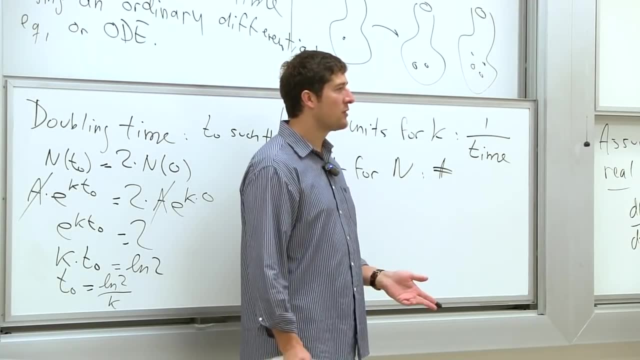 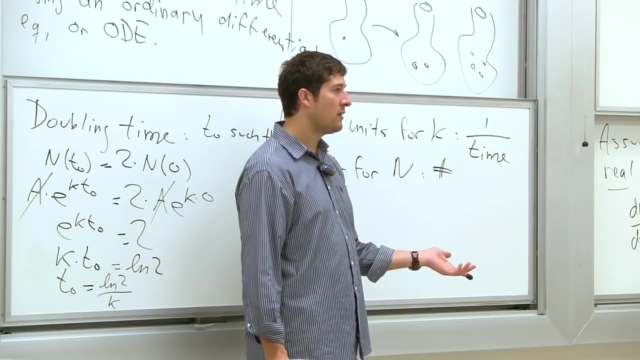 Believe it or not, that's a unit. It's kind of a weird unit, right? We're not used to thinking about number as a unit, But if you've taken a chemistry course, When you think about mole, a mole is a number of molecules, right? 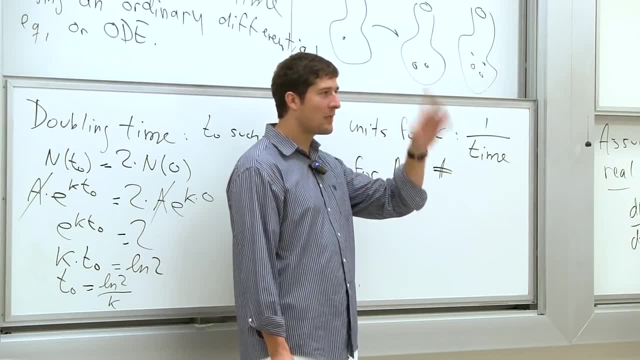 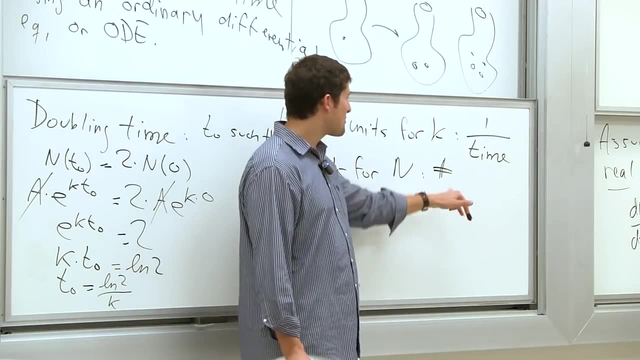 A mole is equal to- I don't know- 10 to the you know six point. something times 10 to the 24 molecules, right? So it's actually the same thing as bacteria, It's just that it's a larger number. 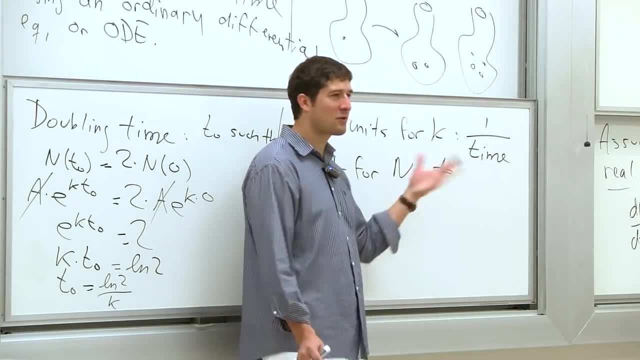 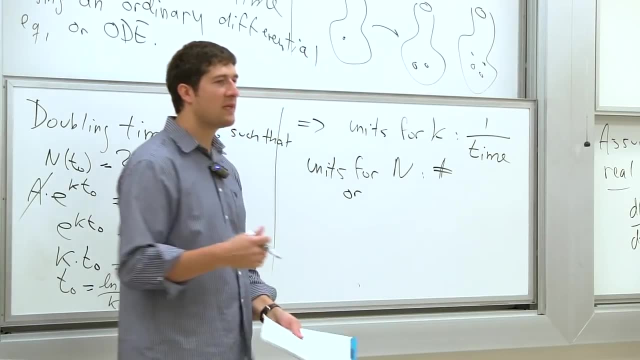 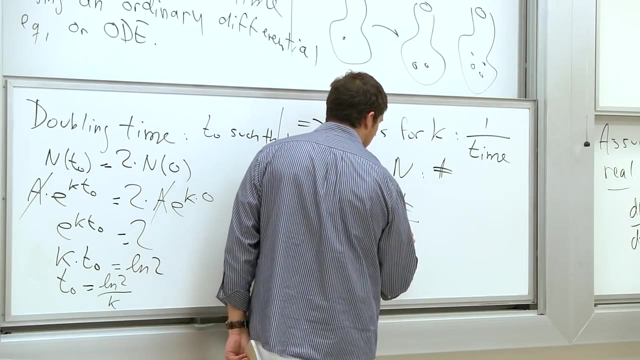 We can come up with a mole for bacteria, but you know who cares, right, We just call it number of bacteria. That's it, Or Or. Sometimes we're going to think about the density of bacteria. So it could be, for example, the number of bacteria divided by volume. 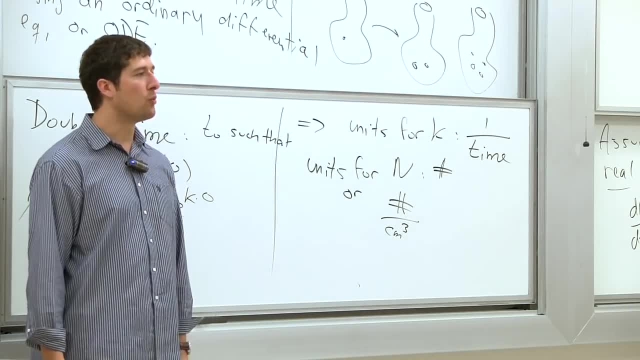 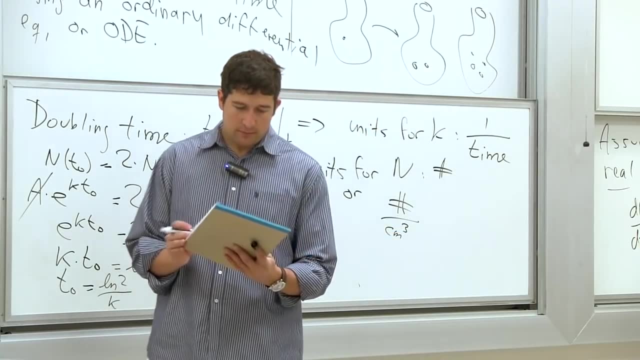 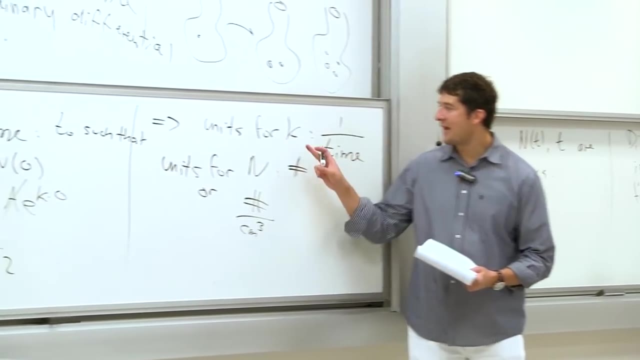 For example, number divided by centimeter cubed. Okay, Alright, So now let's make this a little more interesting. What if we have this constant K? So imagine that somebody you knowIF you're having this recherch, that color. 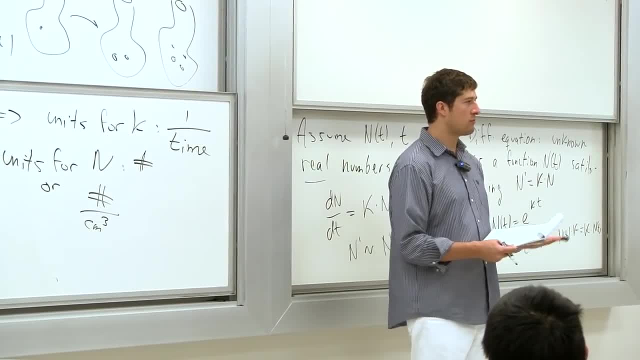 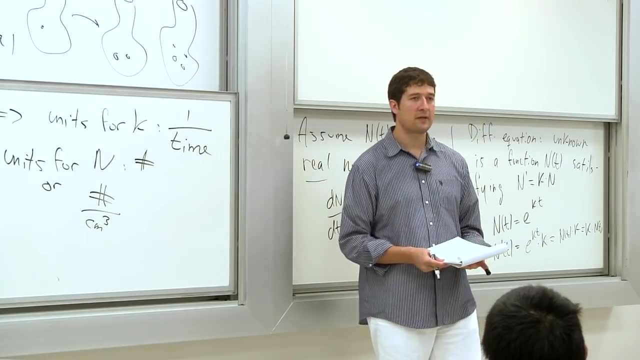 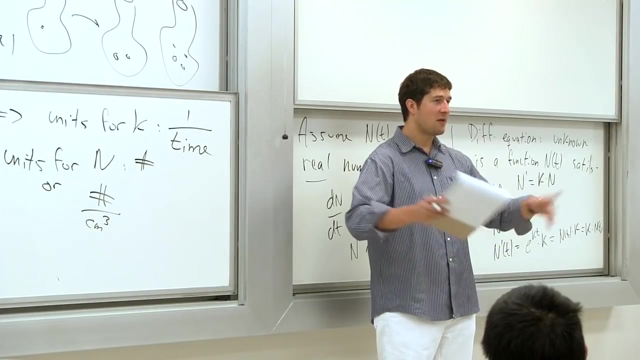 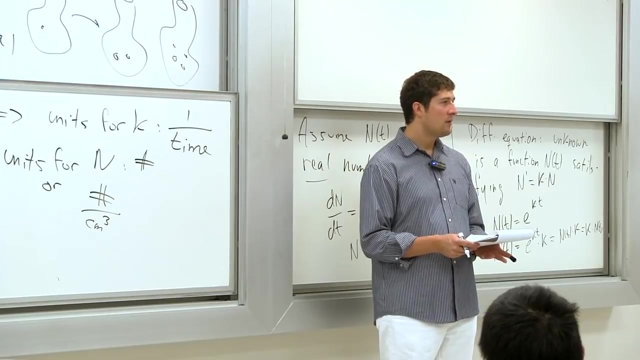 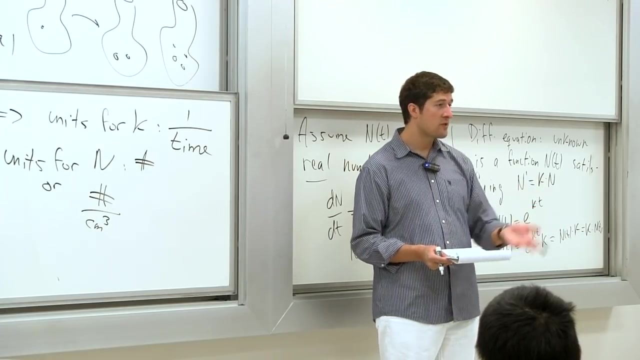 That person. I mean, that would be赤. Alright, Not 64, right, Never, You need Charles even more. Oh boy, Okay, do they do? they don't grow, or they don't grow as fast, or they may actually die. 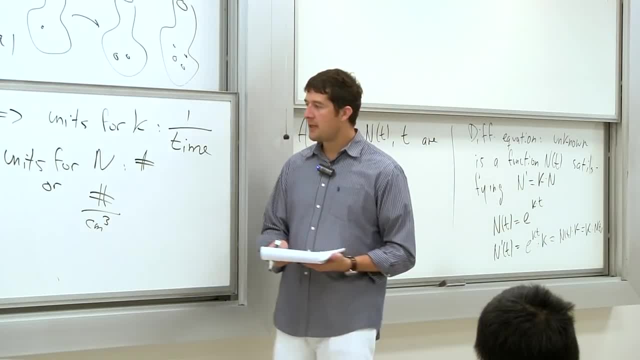 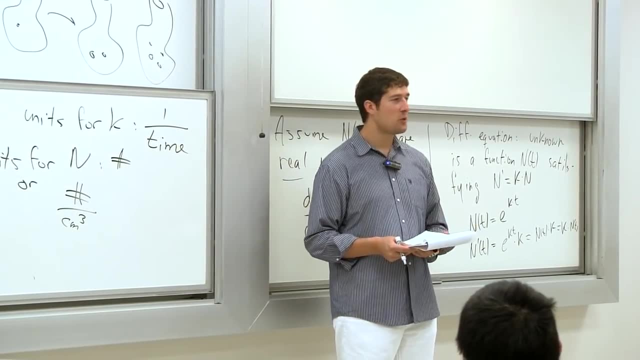 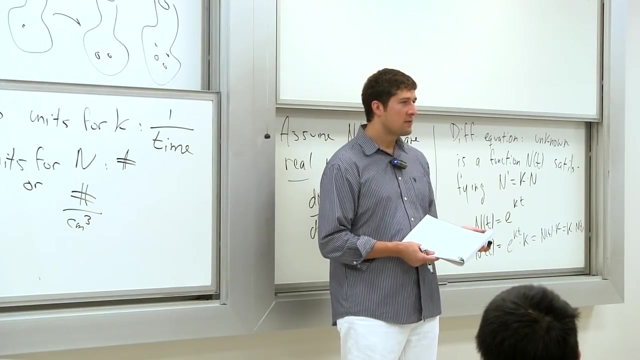 right, depending on the circumstances, right. so so this constant K, which essentially describes the happiness of the bacteria, right? I mean, the larger K, the faster they grow, right. so this constant K depends on a lot of things. it depends on them being, you know, have been, in the right environment, in particular, 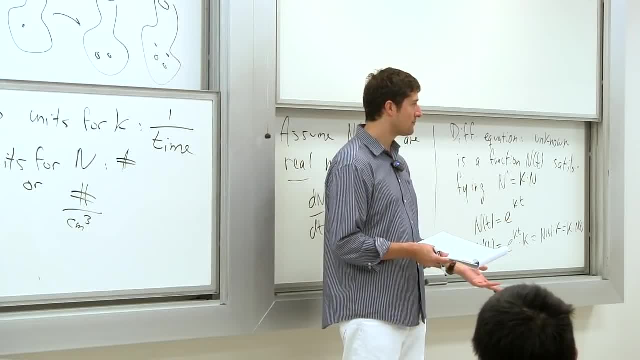 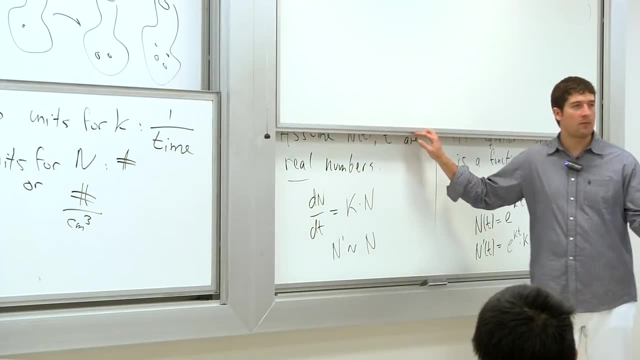 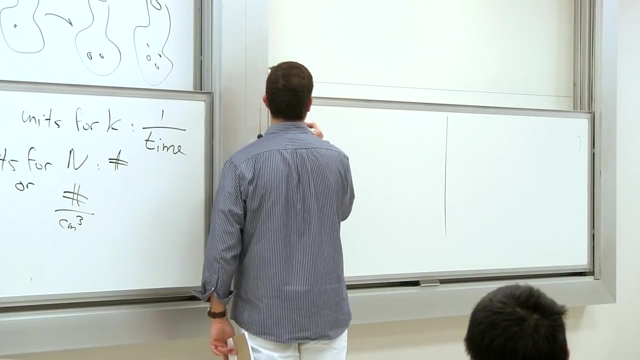 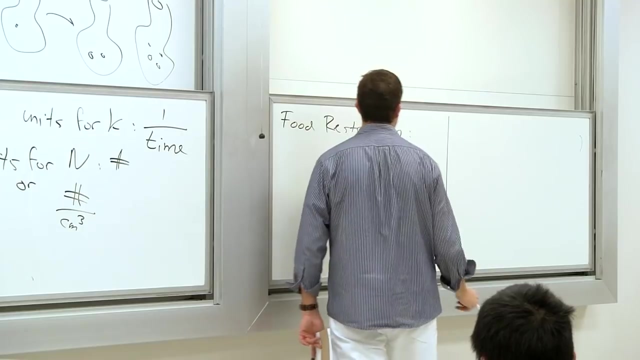 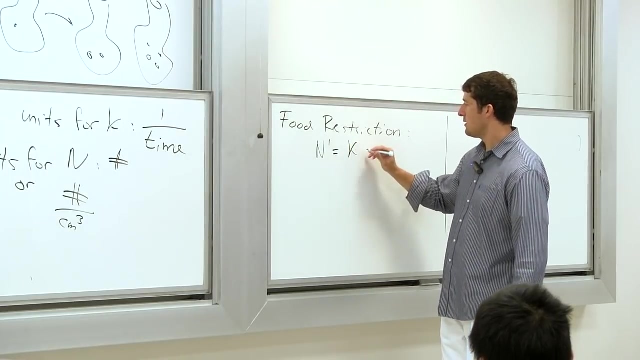 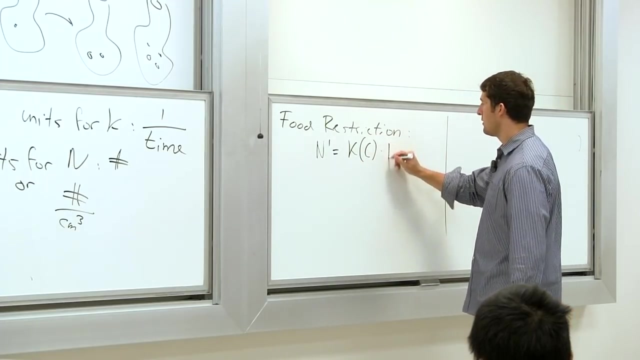 constant K should depend on how much food they have, right? so let's suppose that K depends on this variable food, which is how much food is available in the bottle. so food restrictions, okay. so now you let's suppose that K is dependent on a constant, on a variable C. so this: 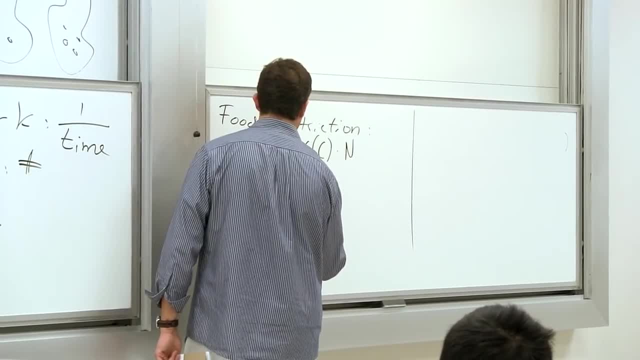 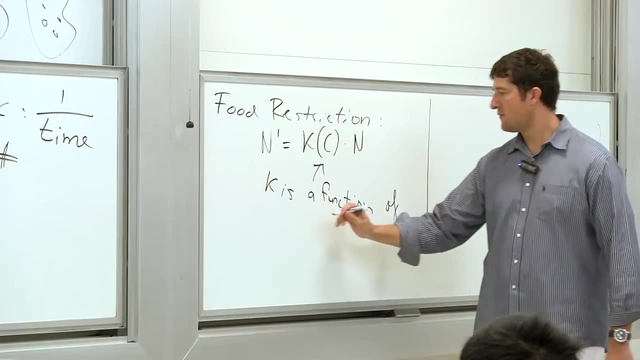 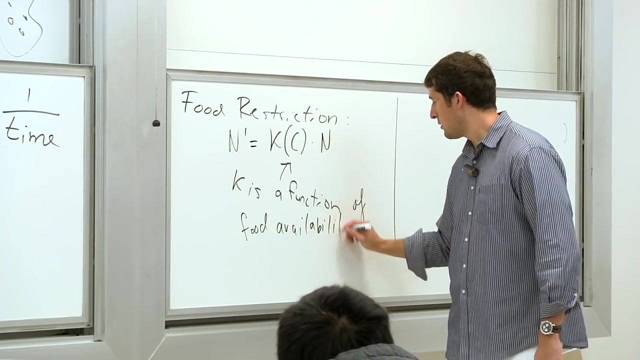 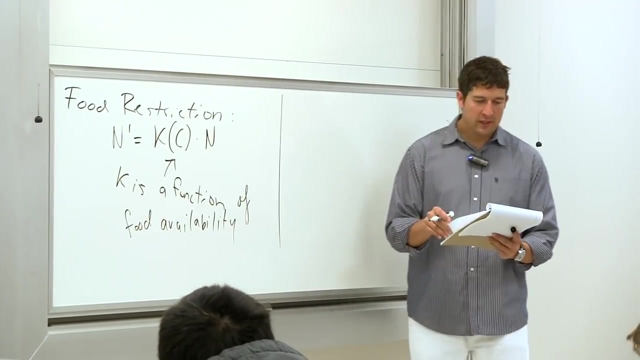 constant. K is not constant anymore. it's a function of food food availability. it's not constant anymore. it's a function of food food availability. okay, and we're going to make an assumption about the food. how do you? okay, and we're going to make an assumption about the food. how do you? 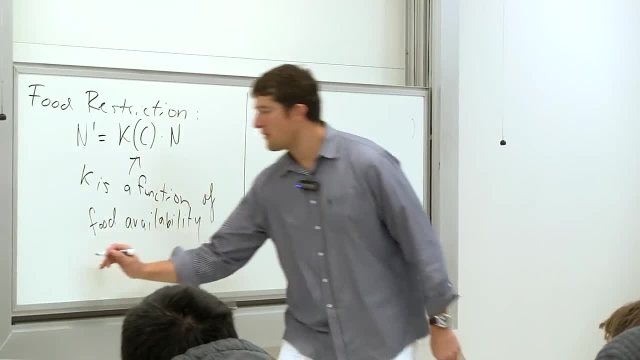 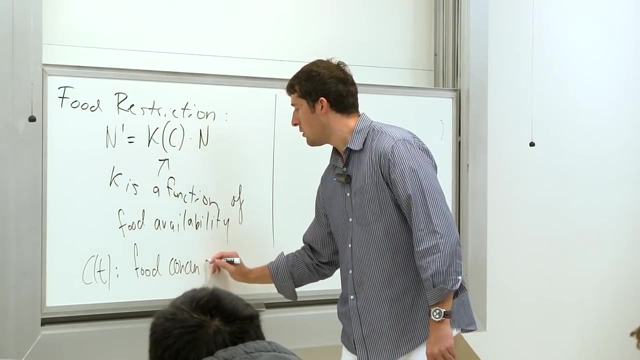 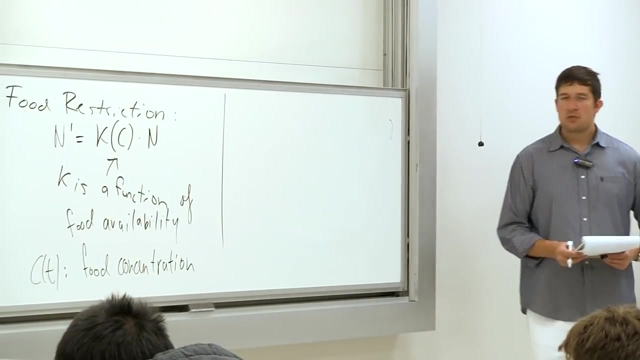 think that the food is consumed, so C of T is the food concentration. does anybody think that the food is consumed? so C of T is the food concentration. does anybody want to suggest a? think that the food is consumed, so C of T is the food concentration. does anybody want to suggest a? 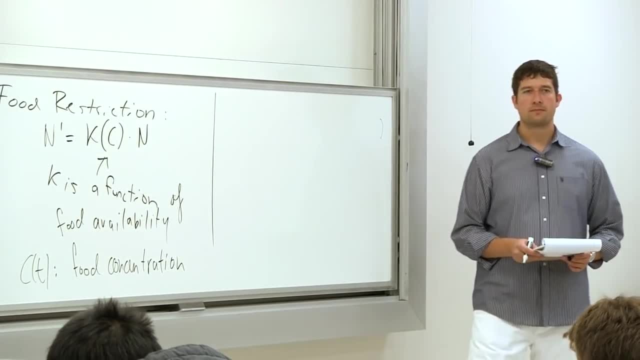 equation for C over time. so for, as a first approximation, we're gonna start equation for C over time. so for, as a first approximation, we're gonna start equation for C over time. so for, as a first approximation, we're gonna start with a bottle of food. we throw in the food in. 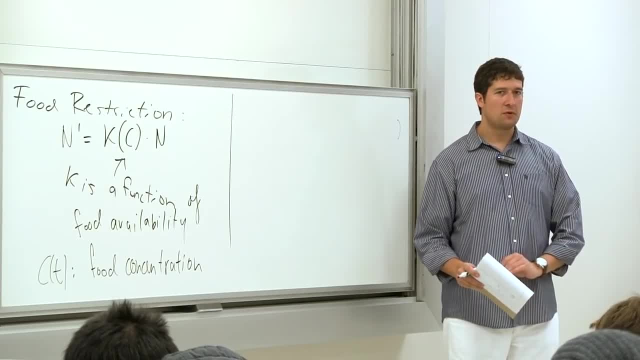 with a bottle of food, we throw in the food in. with a bottle of food, we throw in the food in the beginning. we're not throwing any the beginning. we're not throwing any the beginning. we're not throwing any more food afterwards and the food is you. 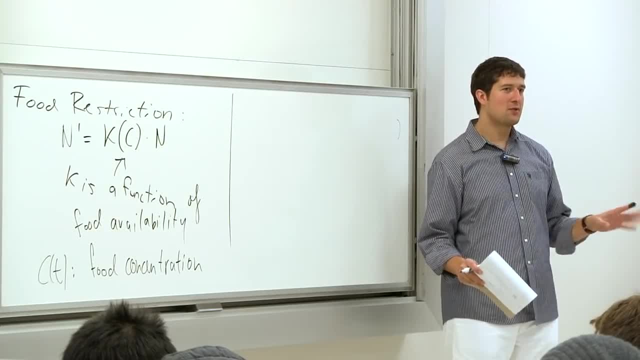 more food afterwards, and the food is you? more food afterwards, and the food is: you know the bacteria consume the food. they know the bacteria consume the food. they know the bacteria consume the food. they probably poop the food in some way. we're probably poop the food in some way. we're. 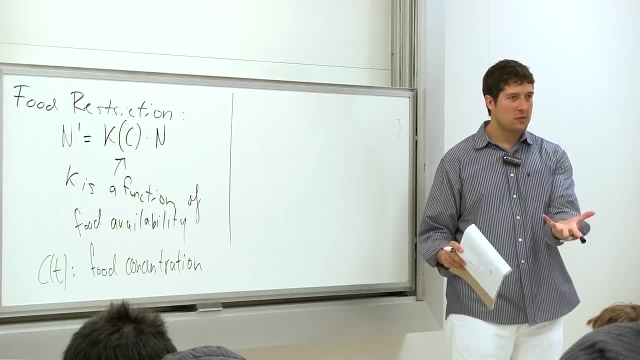 probably poop the food in some way. we're not gonna worry about how the food is, not gonna worry about how the food is not gonna worry about how the food is destroyed, but let the bacteria consume destroyed, but let the bacteria consume destroyed, but let the bacteria consume the food. right, so will be an equation. 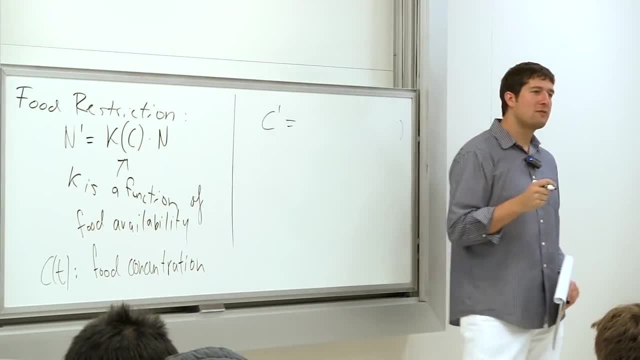 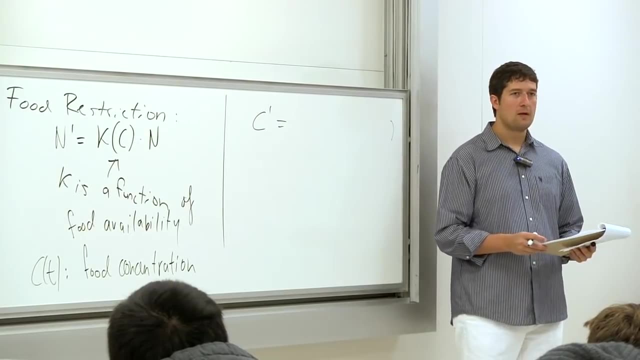 the food right, so will be an equation. the food right, so will be an equation for, for the rate of food destruction, for, for the rate of food destruction, for, for the rate of food destruction. what do you think, so let's see if. what do you think, so let's see if. 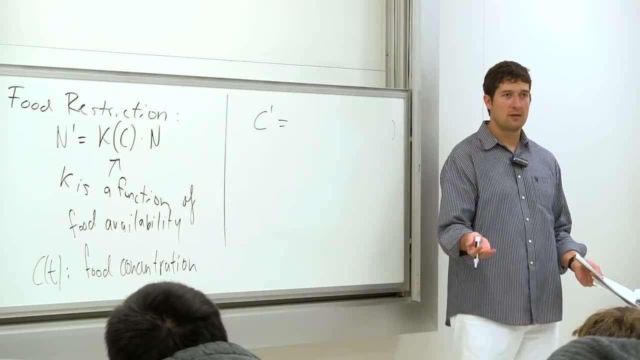 what do you think? so let's see: if there's no bacteria, then the food is. there's no bacteria, then the food is. there's no bacteria, then the food is constant. right, okay now. the more constant, right, okay now. the more constant, right okay now. the more bacteria there are, the faster the food is. 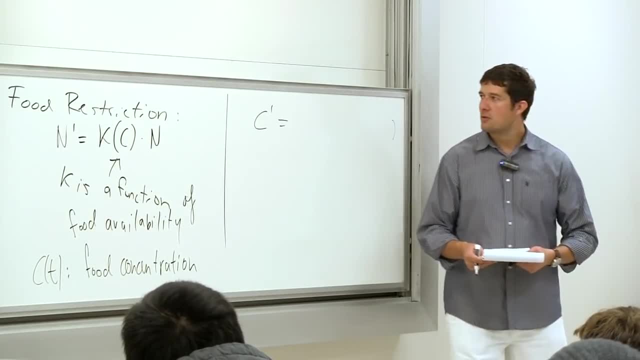 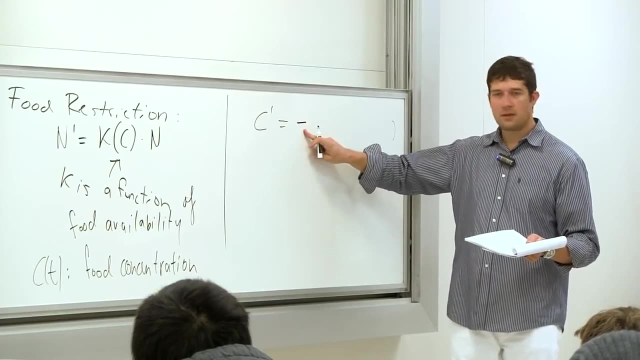 bacteria there are. the faster the food is bacteria there are, the faster the food is consumed, right, you would think right, consumed right, you would think right, consumed right. you would think right. so then, what decreasing exponential? so then, what decreasing exponential? so then, what decreasing exponential function you mean like minus C? 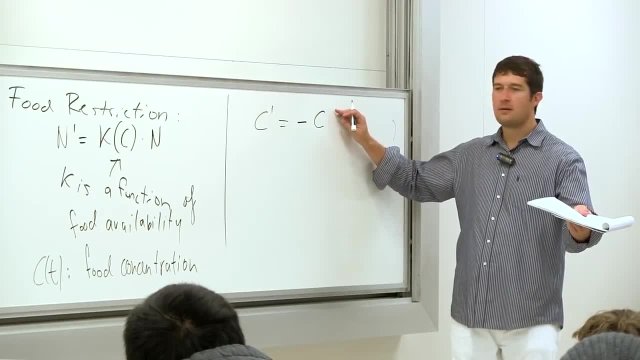 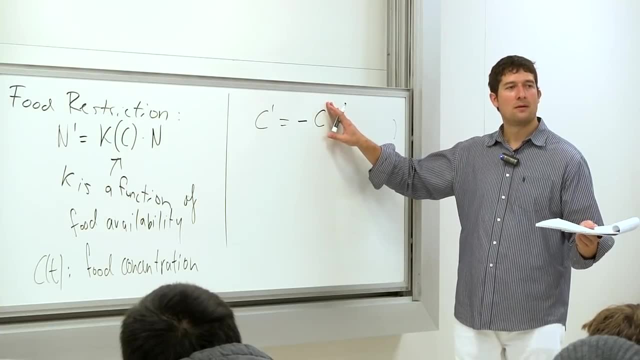 function, you mean like minus C function, you mean like minus C, well, well, well, but if you, if you write something like, but if you, if you write something like, but if you, if you write something like this, whether we do it as an exponential this, whether we do it as an exponential, 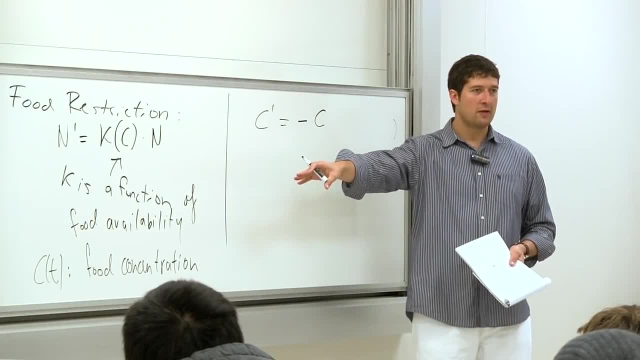 this: whether we do it as an exponential or not, it's not going to depend on the or not. it's not going to depend on the or not. it's not going to depend on the on the bacteria population right, if any. on the bacteria population right, if any. 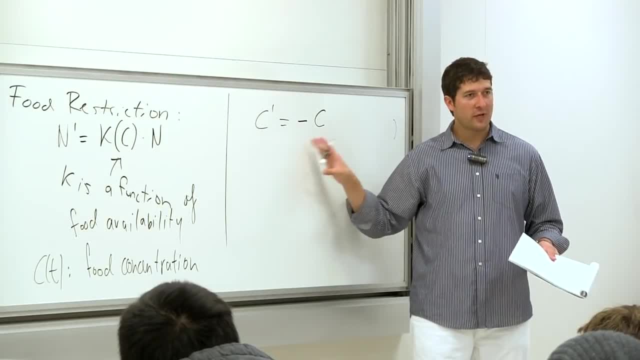 on the bacteria population right, if any zero right, then C C prime should be zero. right then C C prime should be zero. right then C C prime should be equal to 0. so there better be an N in equal to 0. so there better be an N in. 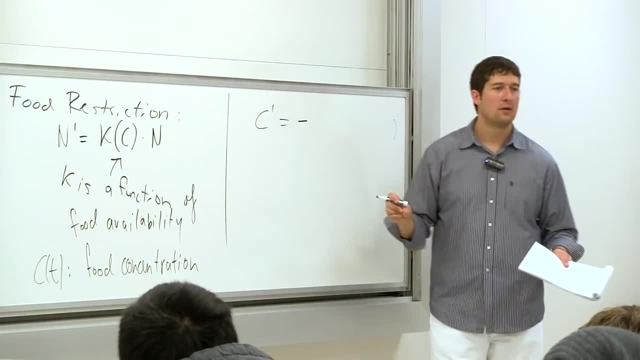 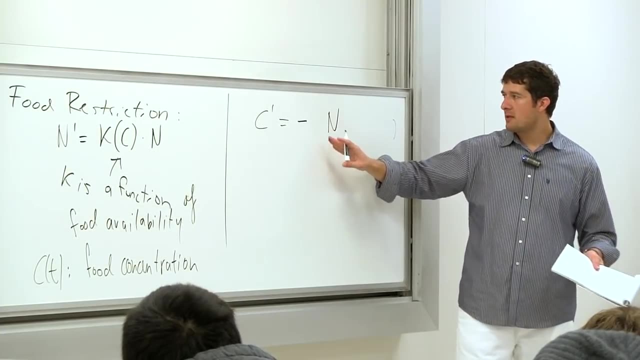 equal to 0, so there better be an N in here. okay. so then, what do you think here? okay, so then, what do you think here? okay, so then, what do you think? negative in, for example: right, okay, but negative in, for example: right okay, but negative in, for example: right, okay, but there's probably gonna have to be some. 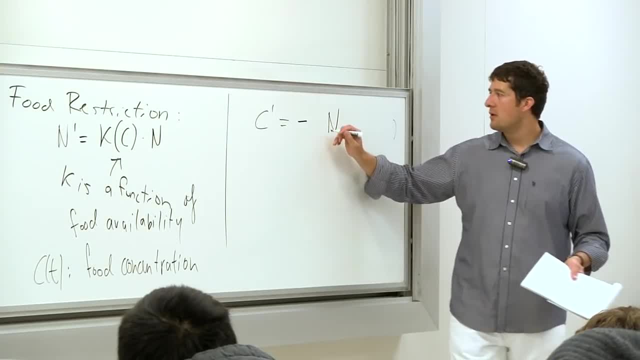 there's probably gonna have to be some. there's probably gonna have to be some constant in here. what do you think let's constant in here? what do you think let's constant in here? what do you think? let's write it like this: minus alpha times and. 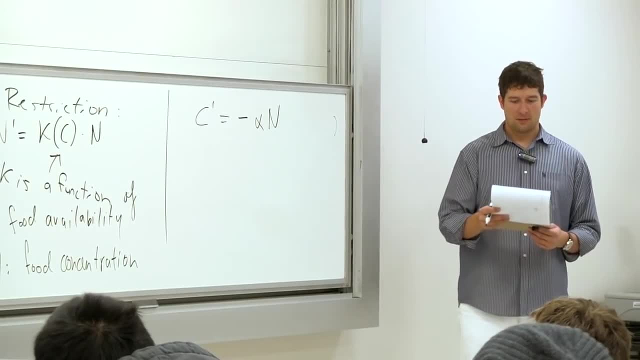 write it like this minus alpha times. and write it like this minus alpha times: and what does alpha mean? actually, no, no, I'm. what does alpha mean? actually, no, no, I'm. what does alpha mean? actually, no, no, I'm sorry. no, it's not, it's not really. and 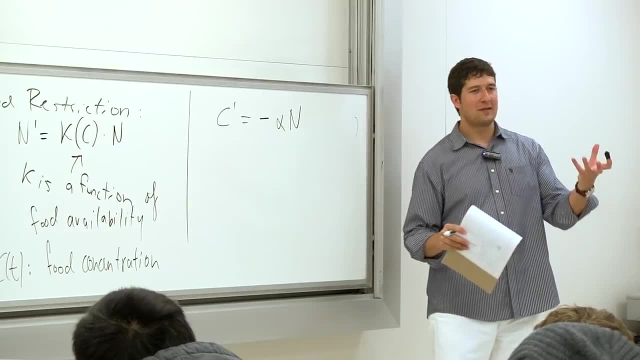 sorry, no, it's not, it's not really. and sorry, no, it's not, it's not really. and it's actually the. the rate of change of it's actually the. the rate of change of it's actually the. the rate of change of n. it's not. it's not the. the present. 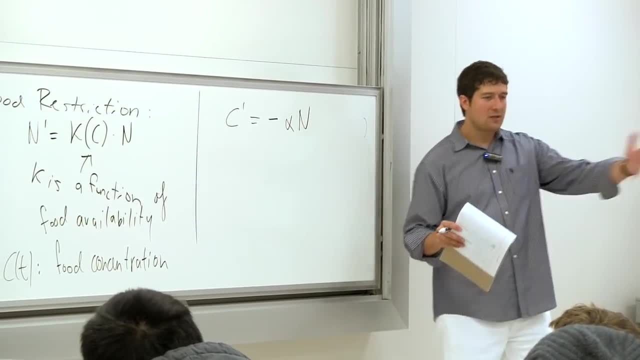 it's not. it's not the the present, it's not. it's not the- the present bacteria that consume the food, but it's bacteria that consume the food, but it's bacteria that consume the food, but it's actually the- the- the rate of growth of actually the. the- the rate of growth of. 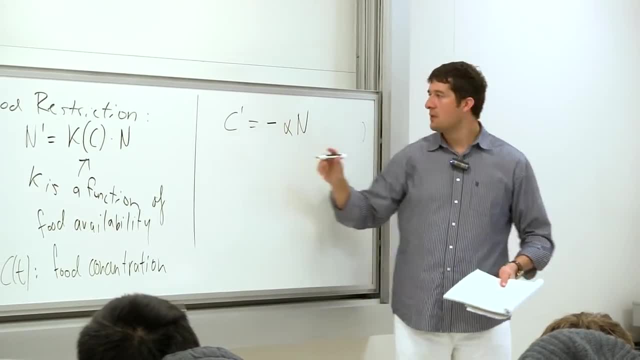 actually the, the, the rate of growth of the bacteria that are causing the, the bacteria that are causing the, the bacteria that are causing the consumption of food. let's do it like this consumption of food. let's do it like this consumption of food. let's do it like this. actually, you can also assume the other. 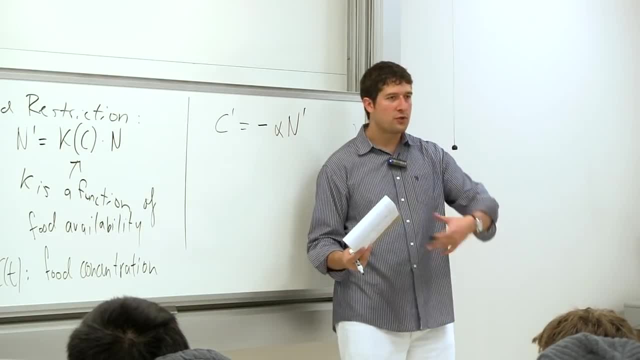 actually, you can also assume the other. actually, you can also assume the other one. you can also assume that if bacteria one, you can also assume that if bacteria one, you can also assume that if bacteria need food to just be there and survive, need food to just be there and survive. 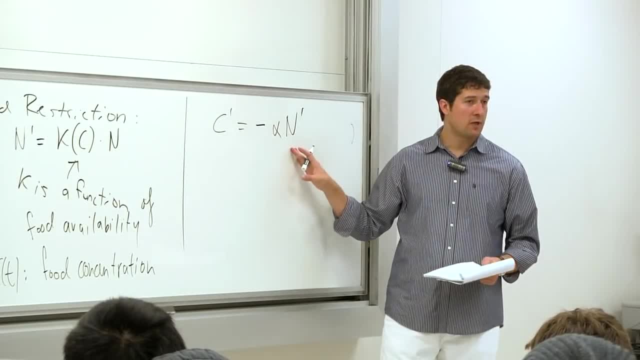 need food to just be there and survive. and you know, just hang around then. and you know, just hang around then. and you know, just hang around then. there's gonna be an N term in here, but there's gonna be an N term in here, but there's gonna be an N term in here. but let's suppose the bacteria only need 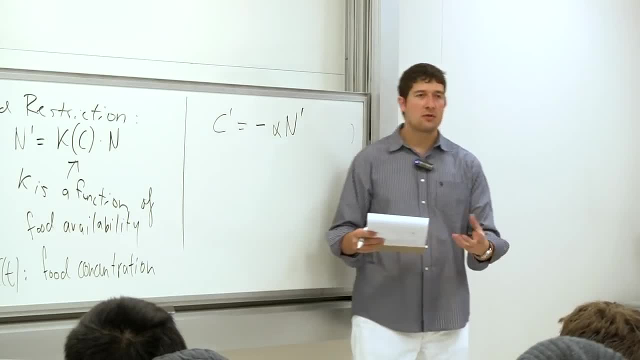 let's suppose the bacteria only need. let's suppose the bacteria only need food to the extent that they're growing food, to the extent that they're growing food, to the extent that they're growing right. so if there's and there's for right, so if there's and there's for 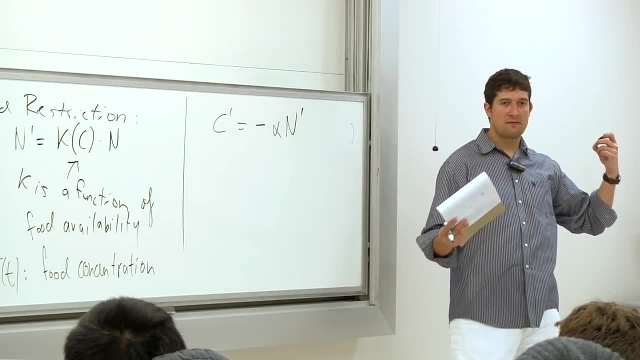 right. so if there's and there's, for example, five new bacteria, then there's example, five new bacteria, then there's example, five new bacteria, then there's gonna be a consumption of food, if gonna be a consumption of food, if gonna be a consumption of food, if there's ten new bacteria, there's gonna be. 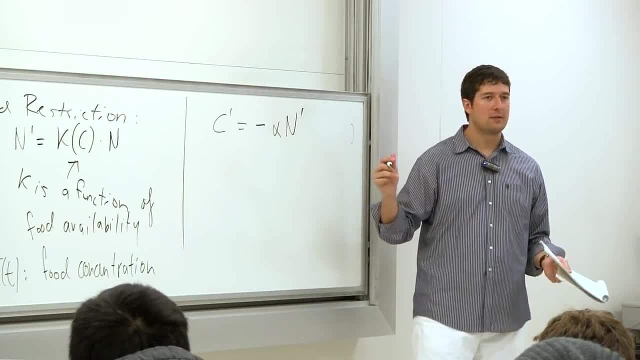 there's ten new bacteria. there's gonna be. there's gonna be ten new bacteria. there's gonna be twice as much consumption of food. twice as much consumption of food, twice as much consumption of food. okay, so then alpha will be what alpha is a. okay, so then alpha will be what alpha is a. 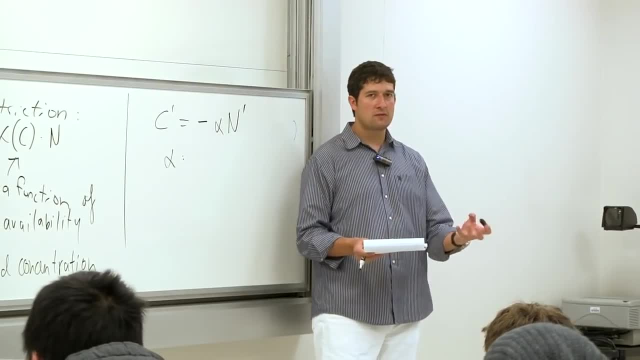 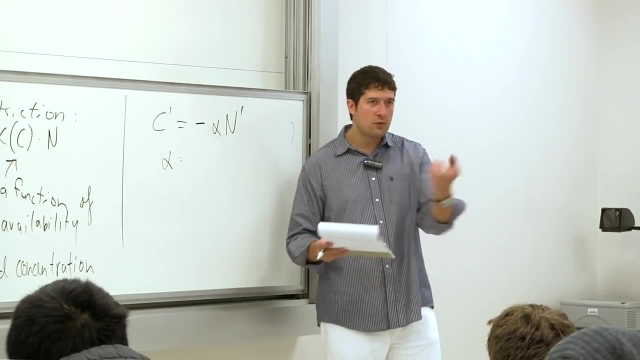 okay, so then alpha will be what alpha is? a constant that tells us how much food. a constant that tells us how much food. a constant that tells us how much food a new bacterium is consuming- right, the new bacterium is consuming. right, the new bacterium is consuming right? the larger alpha, the more food each. 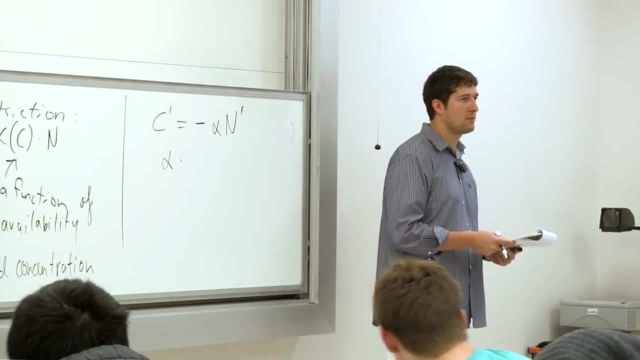 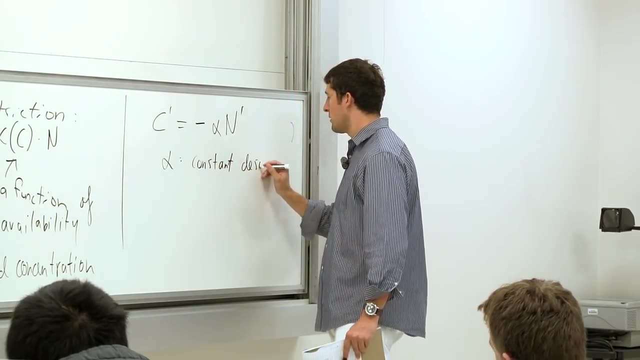 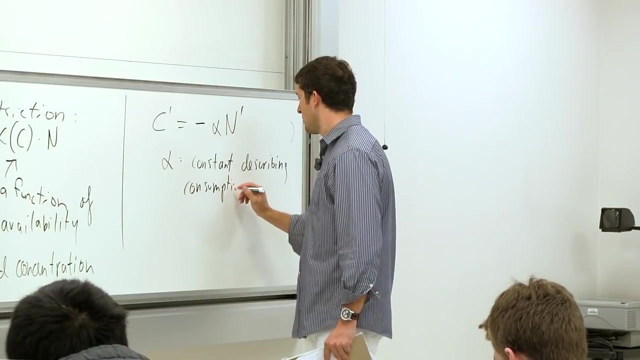 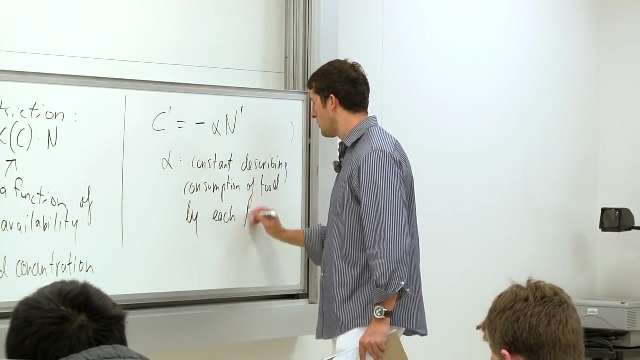 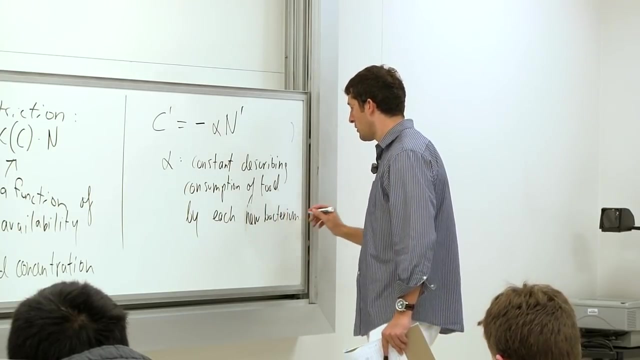 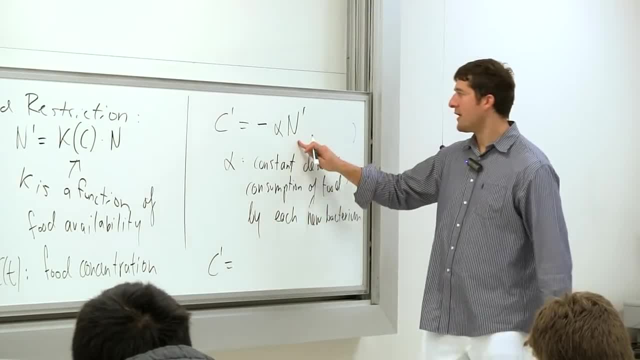 bacterium by its new bacterium- okay, but bacterium by its new bacterium- okay, but we know that C Prime- sorry. we know that. we know that C Prime- sorry. we know that. we know that C Prime- sorry. we know that M prime has that. M prime has that. 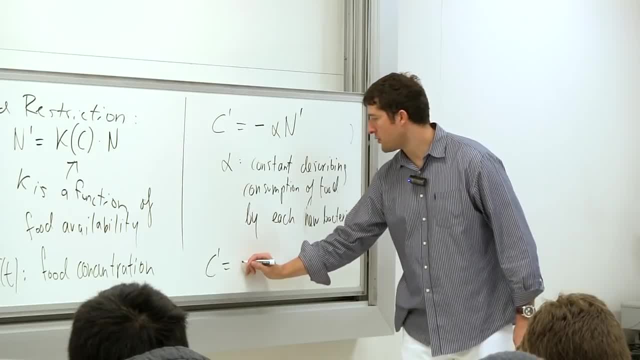 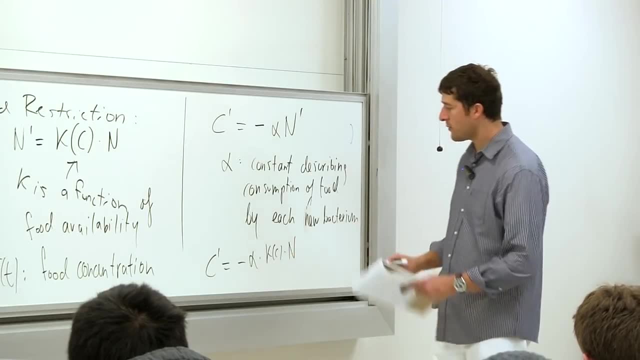 M prime has that formula over there. so then C Prime is formula over there. so then C Prime is formula over there. so then C Prime is equal to minus alpha times K of C times. equal to minus alpha times K of C times. equal to minus alpha times K of C times times n. 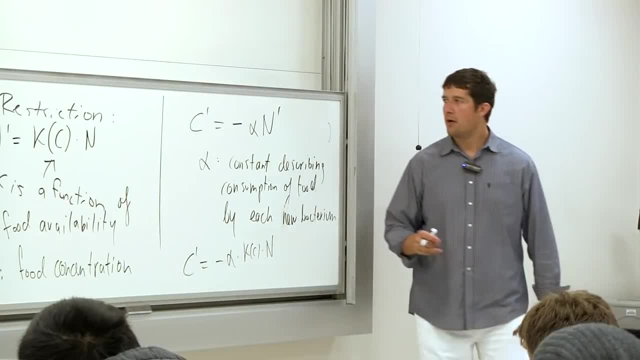 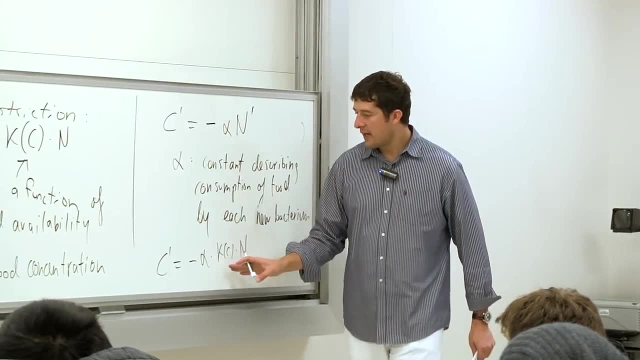 times n times n. okay, all right, now, let's make a new. okay, all right now, let's make a new. okay, all right, now, let's make a new assumption, just to be able to analyze assumption, just to be able to analyze assumption, just to be able to analyze this thing. and let's suppose that K is. 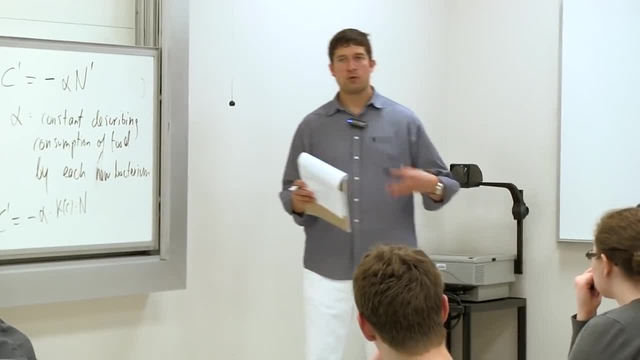 this thing, and let's suppose that K is this thing, and let's suppose that K is proportional to C. in other words, the proportional to C. in other words, the proportional to C. in other words, the more food the bacteria has, the happier. more food the bacteria has, the happier. 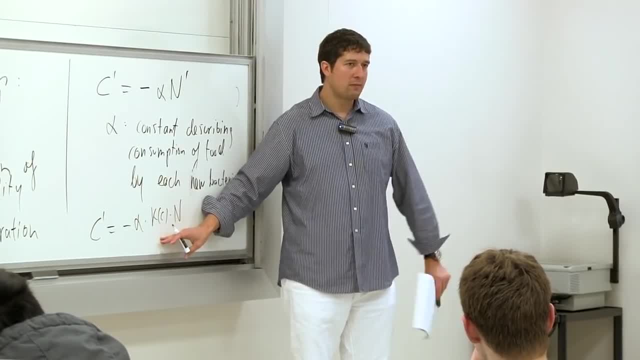 more food the bacteria has, the happier it is okay. we don't have to assume that it is okay. we don't have to assume that it is okay. we don't have to assume that we can make it. we can make another, we can make it, we can make another. 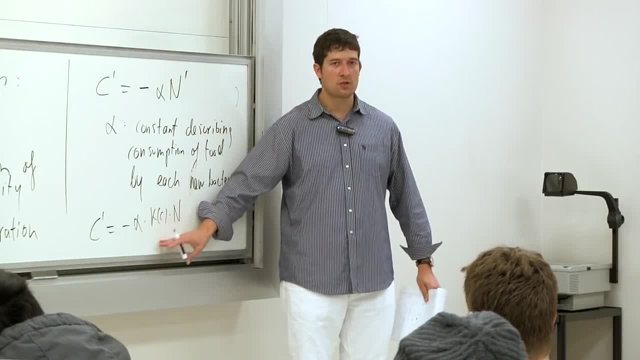 we can make it, we can make another assumption. it's just that to analyze the assumption. it's just that to analyze the assumption. it's just that to analyze the system is going to be easier if we make system is going to be easier if we make system is going to be easier if we make an assumption about the form of this. 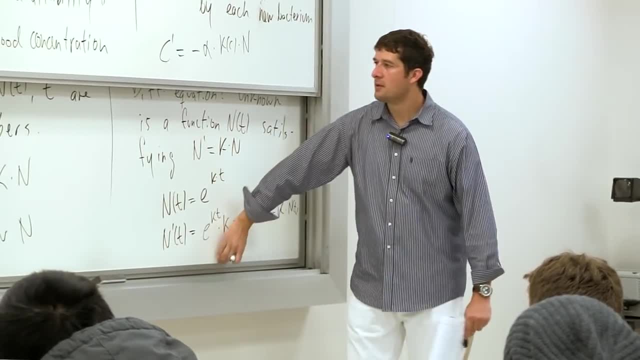 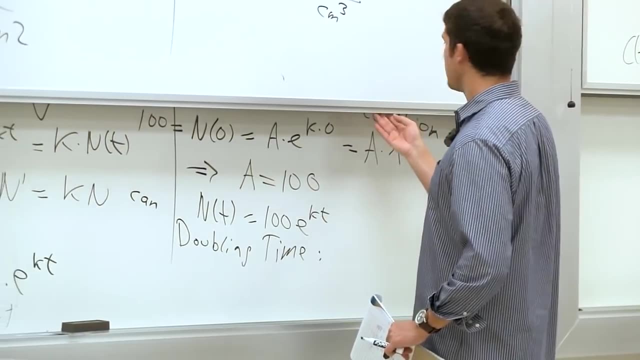 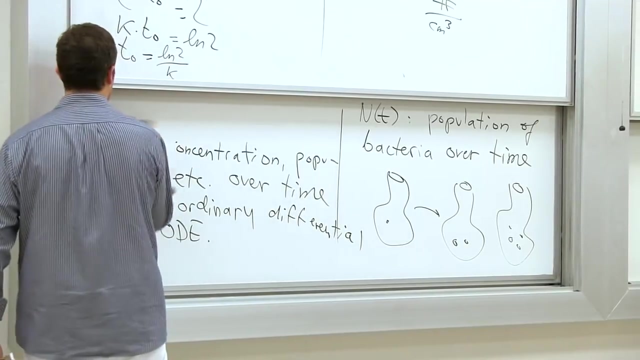 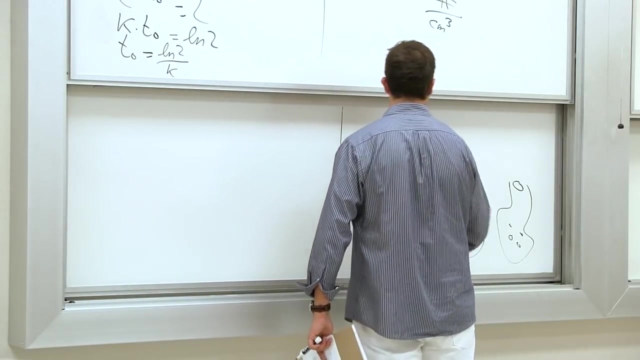 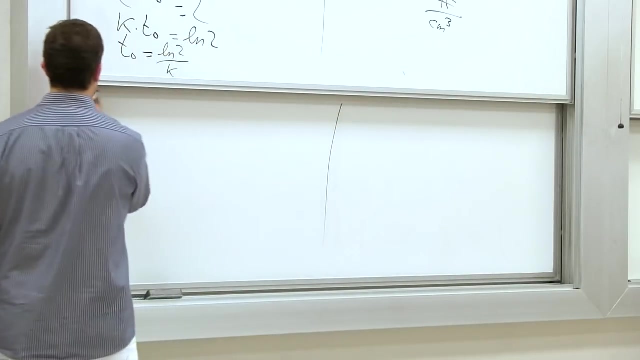 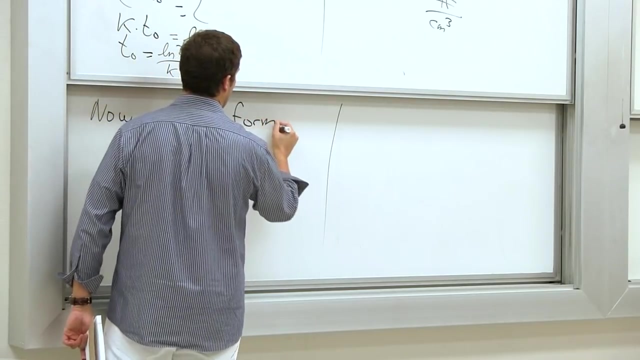 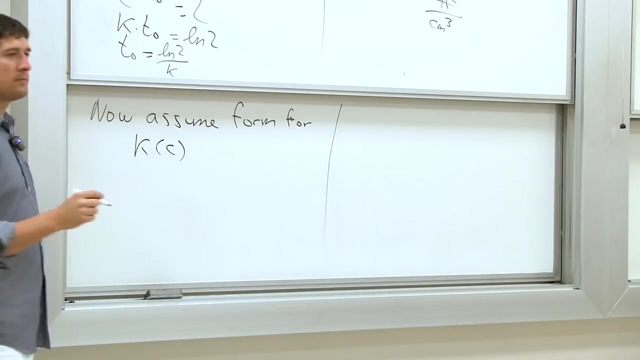 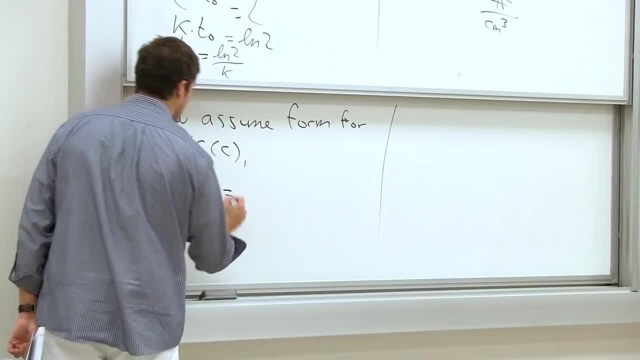 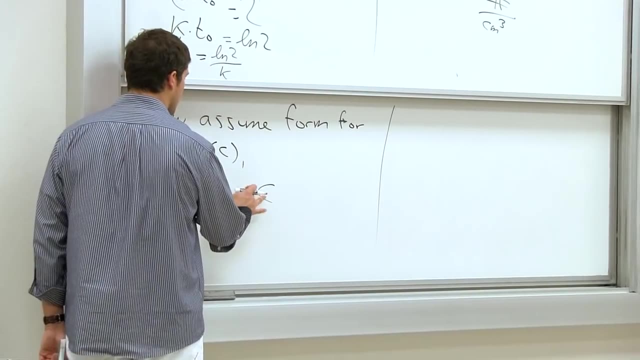 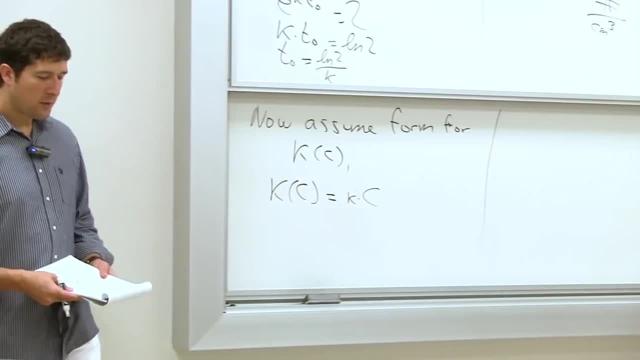 a constant times C. and, and here it's a a constant times C. and, and here it's a little bit awkward to write on the board. little bit awkward to write on the board. little bit awkward to write on the board. but I really should be, I really should. 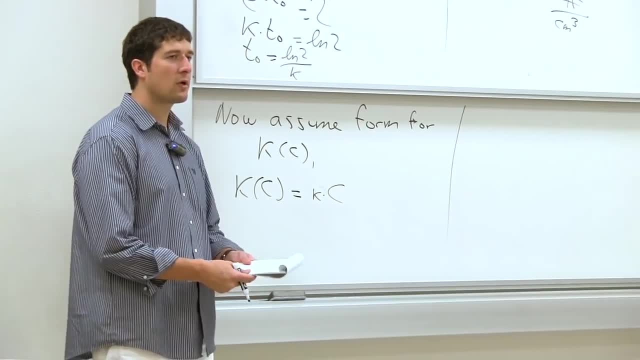 but I really should be, I really should, but I really should be. I really should follow the the notation of the book. so follow the the notation of the book. so follow the the notation of the book so that we can read the book and follow the that we can read the book and follow the. 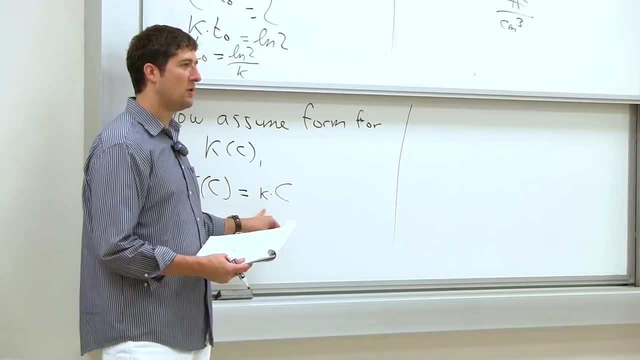 that we can read the book and follow the class at the same time and the book uses class at the same time, and the book uses class at the same time. and the book uses this small, smaller case K. it's more of this small, smaller case K. it's more of. 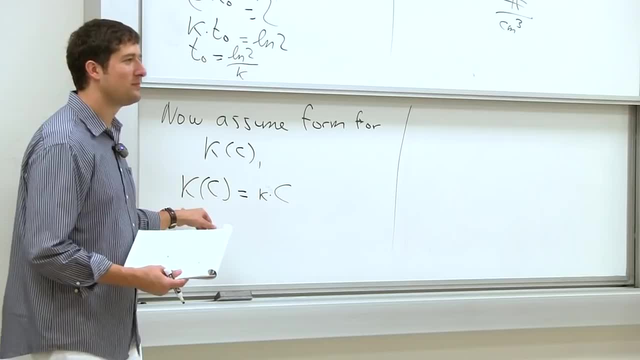 this small, smaller case K, it's more of a Kappa. actually this is a Kappa and this a Kappa. actually this is a Kappa and this a Kappa. actually this is a Kappa and this is a capital K. okay, and they look is a capital K, okay, and they look. 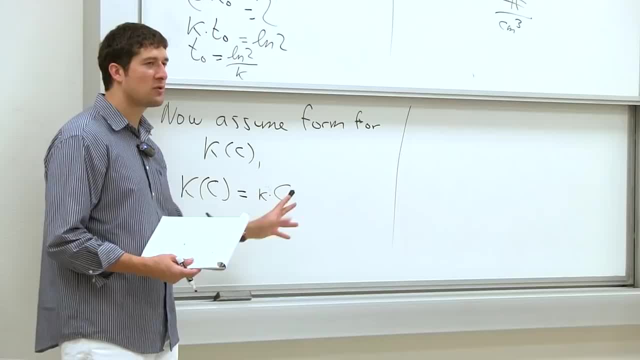 is a capital K okay, and they look almost the same. but I mean I'm not sure almost the same. but I mean I'm not sure, almost the same, but I mean I'm not sure if maybe I should use a different, if maybe I should use a different. 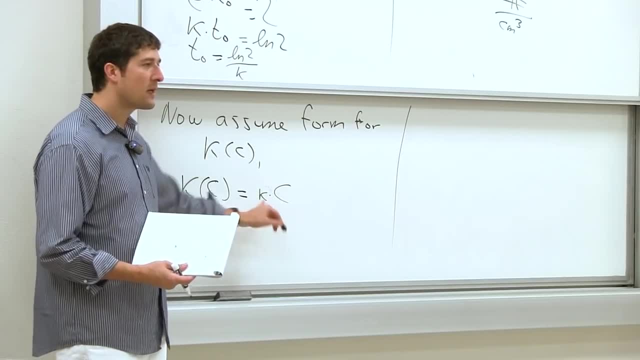 if maybe I should use a different constant for the board, but I think it constant for the board, but I think it constant for the board, but I think it should be fine. let's just remember this should be fine. let's just remember. this should be fine. let's just remember this is little K and this is large K. okay, I. is little K and this is large K. okay, I is little K and this is large K. okay, I think it should be fine. because we're think it should be fine, because we're think it should be fine, because we're gonna multiply by C, you can see the. 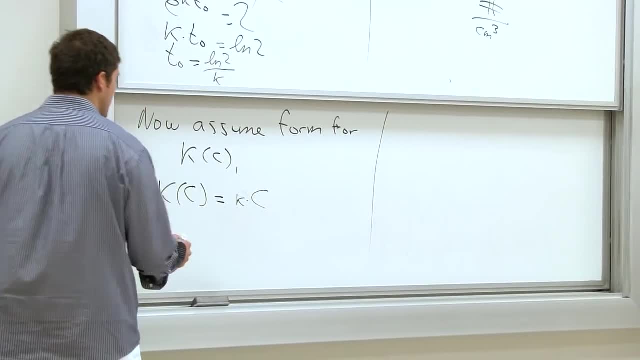 gonna multiply by C. you can see the gonna multiply by C. you can see the small K and the large C. so should be small K and the large C. so should be small K and the large C. so should be okay, all right. so now this: how do you? 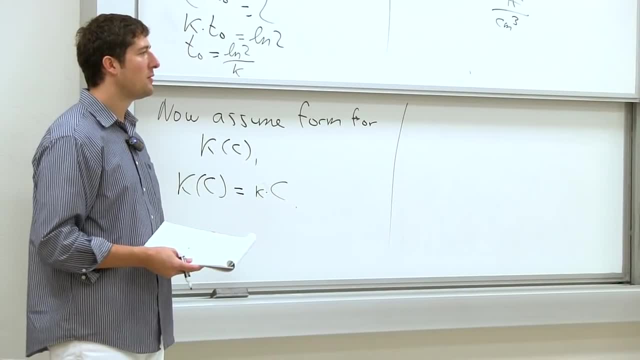 okay, all right. so now this. how do you? okay, all right. so now this. how do you? how would you describe this assumption? how would you describe this assumption? how would you describe this assumption? what, what, what are we assuming here? so? what, what, what are we assuming here? so? 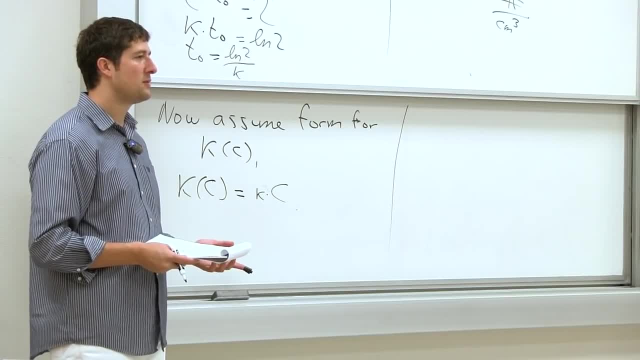 what, what, what are we assuming here? so, if there's no food, how fast to the? if there's no food, how fast to the? if there's no food, how fast to the tree I grow- they don't grow at all right. tree I grow, they don't grow at all right. tree I grow. they don't grow at all. right, okay, if there's a lot of food, then okay. if there's a lot of food, then okay. if there's a lot of food, then bacteria grow very, very fast right now. bacteria grow very, very fast right now. 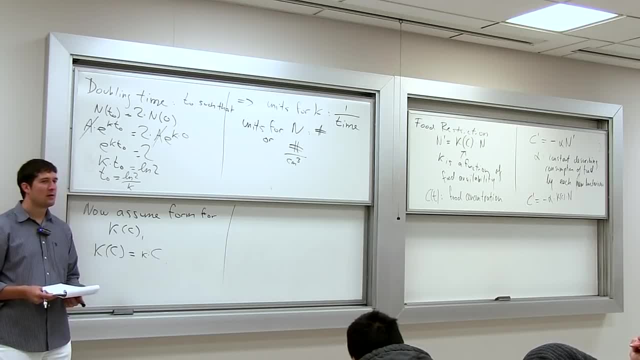 bacteria grow very, very fast right now. what do you think? is this a reasonable? what do you think is this a reasonable? what do you think is this a reasonable assumption to make, or does it have a assumption to make? or does it have a assumption to make or does it have a problem? what if there's like a thousand? 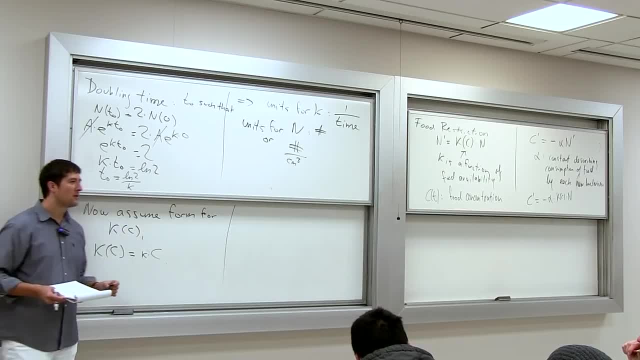 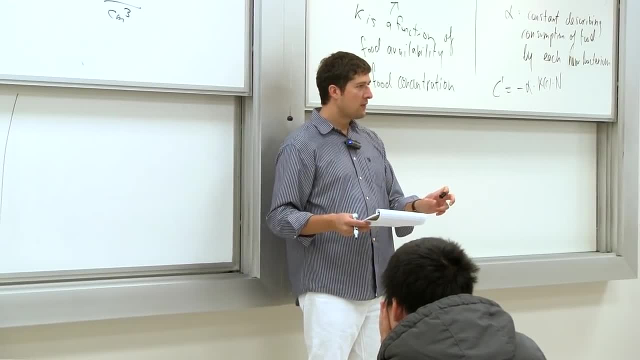 exactly, exactly, if you remember, K is the proportionality rate for the growth of the proportionality rate for the growth of the proportionality rate for the growth of bacteria: right the larger K, not little bacteria. right the larger K, not little bacteria. right the larger K, not little Kappa, but large K. right the larger K, the. 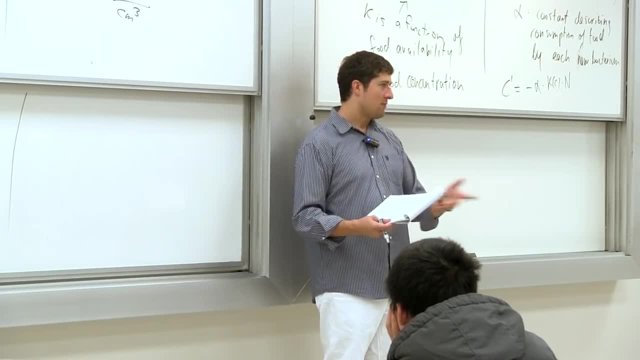 Kappa, but large K right the larger K the Kappa, but large K right the larger K, the faster they grow. but bacteria, I mean we faster they grow, but bacteria. I mean we faster they grow, but bacteria. I mean we know this about bacteria. if you give 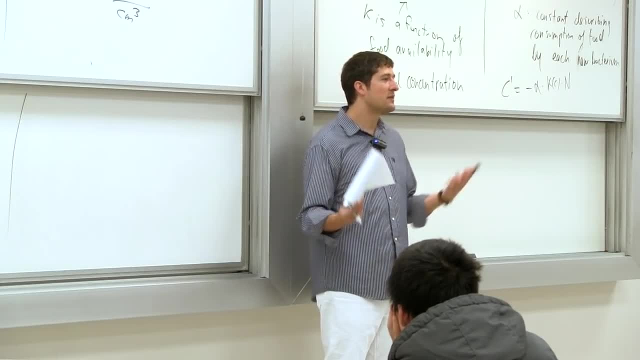 know this about bacteria: if you give know this about bacteria: if you give them as much food as they want- at some them as much food as they want, at some them as much food as they want- at some point they're not gonna grow faster than point. they're not gonna grow faster than. 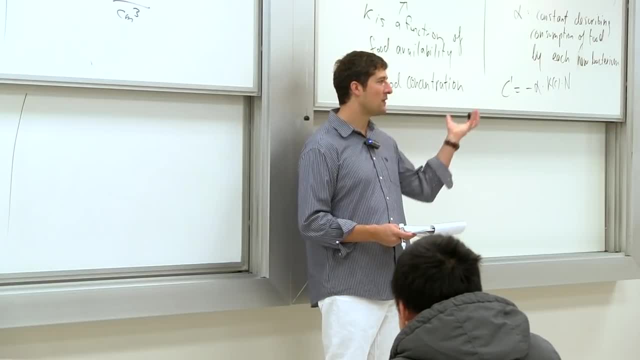 point. they're not gonna grow faster than proteins and amino acids and whatnot- proteins and amino acids and whatnot- proteins and amino acids and whatnot- and they need to, then you also need other. and they need to. then you also need other. and they need to. then you also need other sources from the environment. they need. 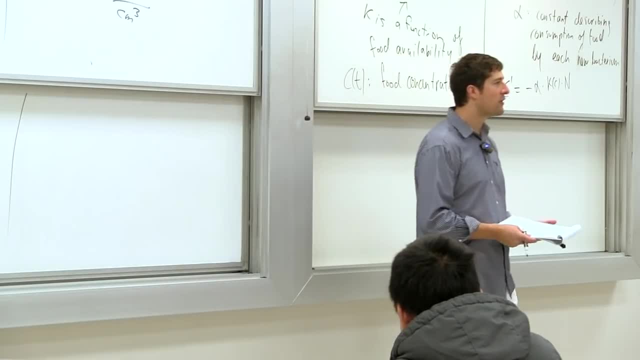 sources from the environment. they need sources from the environment. they need, they really need more time. you know they, they really need more time. you know they, they really need more time. you know they cannot grow arbitrarily fast. so really cannot grow arbitrarily fast. so really cannot grow arbitrarily fast. so really, K is what we call a saturating function. 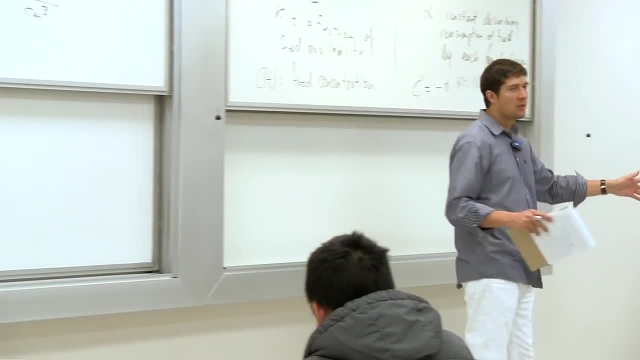 K is what we call a saturating function. K is what we call a saturating function. in other words, if C is really really. in other words, if C is really really. in other words, if C is really, really, really large. case should not be really large, case should not be. 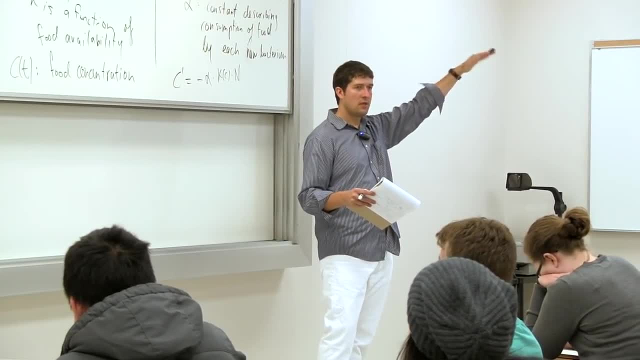 really large case should not be arbitrarily large but should reach some arbitrarily large, but should reach some arbitrarily large but should reach some kind of saturation and not grow beyond kind of saturation and not grow beyond kind of saturation and not grow beyond that right but for the purposes of the 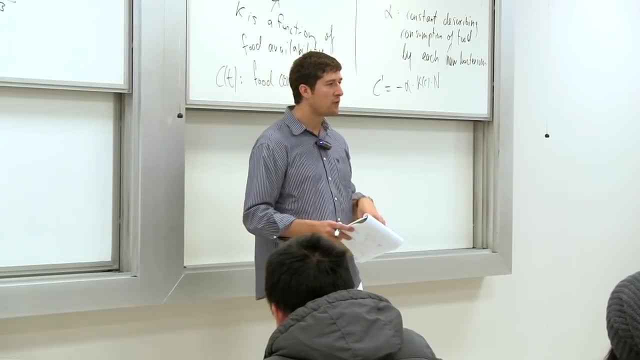 that right, but for the purposes of the that right, but for the purposes of the analysis. I believe we're going to analysis. I believe we're going to analysis. I believe we're going to actually solve the system, not not today. actually solve the system, not not today. 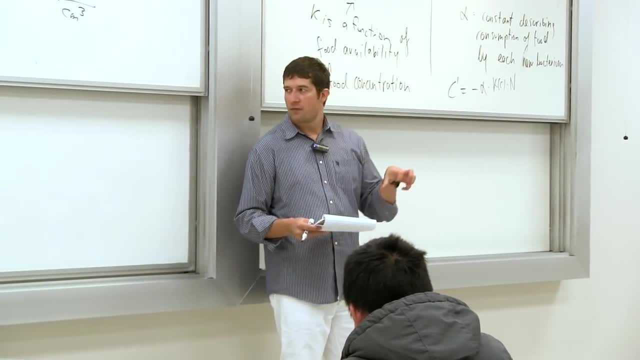 actually solve the system, not not today, but later in the few lectures, or maybe, but later in the few lectures, or maybe, but later in the few lectures, or maybe even on Wednesday for the purpose of even on Wednesday. for the purpose of even on Wednesday, for the purpose of this analysis, we're going to make a 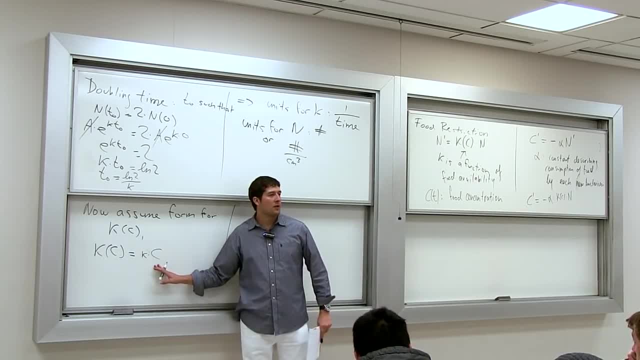 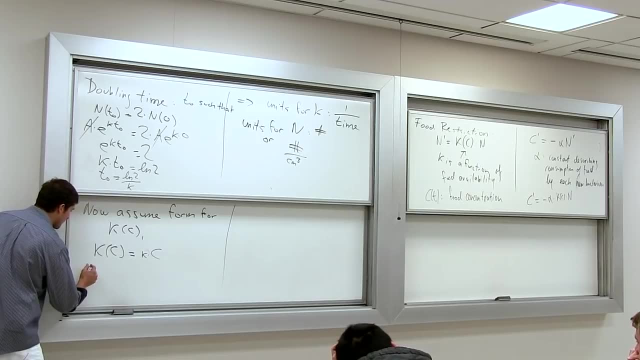 this analysis, we're going to make a. this analysis, we're going to make a simple assumption: that the more food. simple assumption that the more food. simple assumption that the more food there is available, the faster the there is available. the faster the there is available, the faster the bacteria grow. okay, so all right. so now, 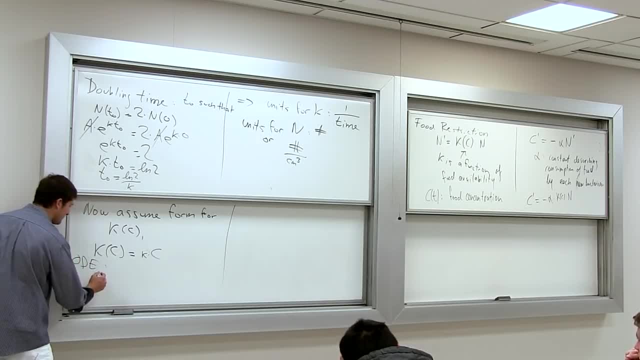 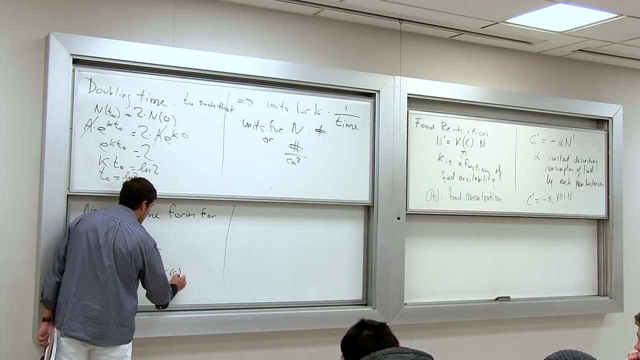 bacteria grow okay, so all right. so now bacteria grow okay, so all right. so now the ODE now looks like this: n prime of the ODE now looks like this: n prime of the ODE now looks like this: n prime of T is equal to K of C times n. 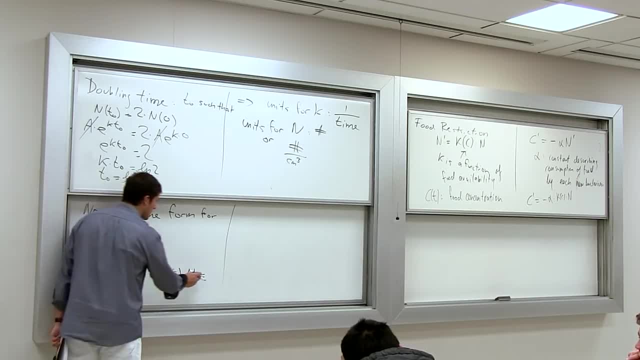 T is equal to K of C times n. T is equal to K of C times n, and if you remember- now we're using this, and if you remember- now we're using this, and if you remember- now we're using this formula- that it is little K times C. 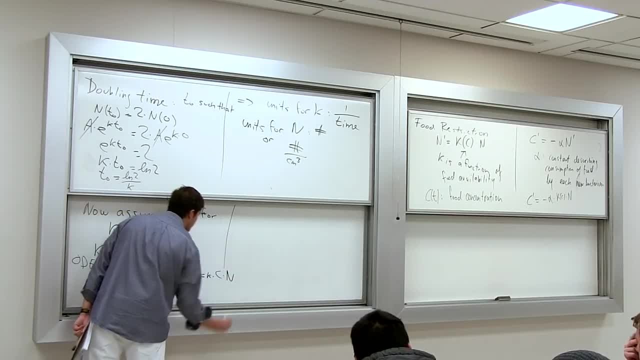 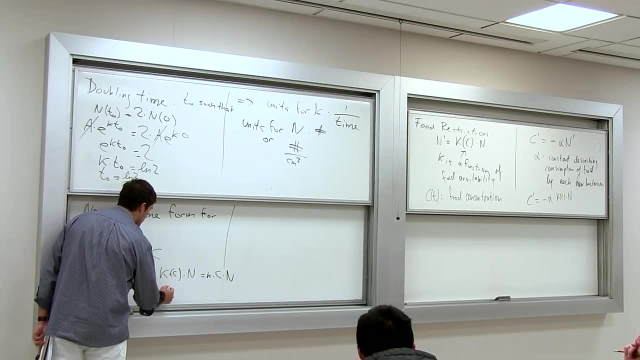 formula that it is little K times C. formula that it is little K times C. sorry this, Kappa Kappa times C times n. sorry this Kappa Kappa times C times n. sorry this Kappa Kappa times C times n. okay, and C prime of T is equal to minus. 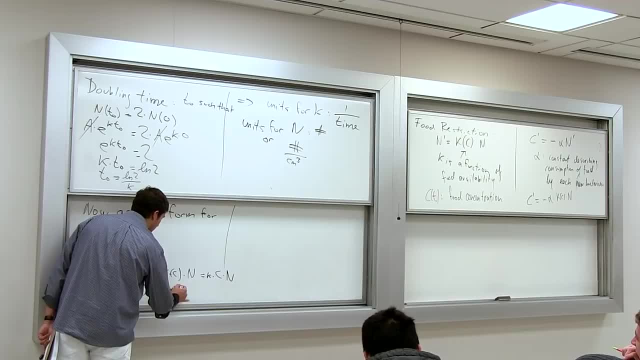 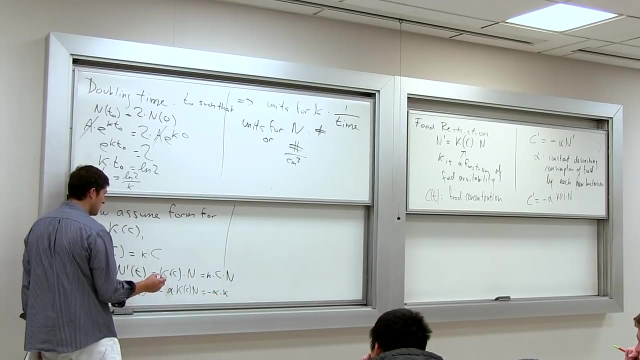 okay, and C prime of T is equal to minus. okay, and C prime of T is equal to minus. alpha times: alpha times: alpha times K of C- n is equal to minus. alpha times K of C? n is equal to minus. alpha times K of C? n is equal to minus. alpha times: Kappa times: C times n. all right now. 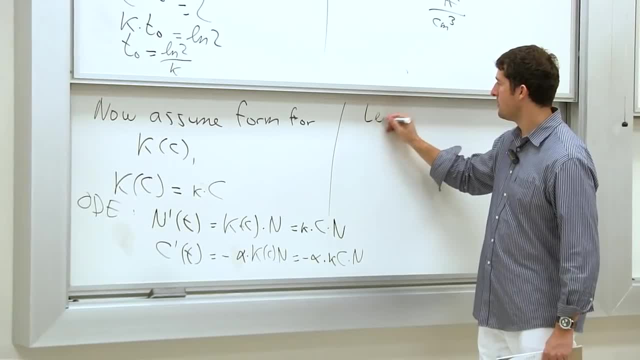 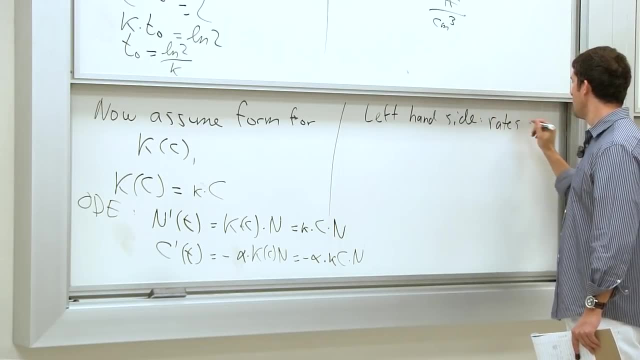 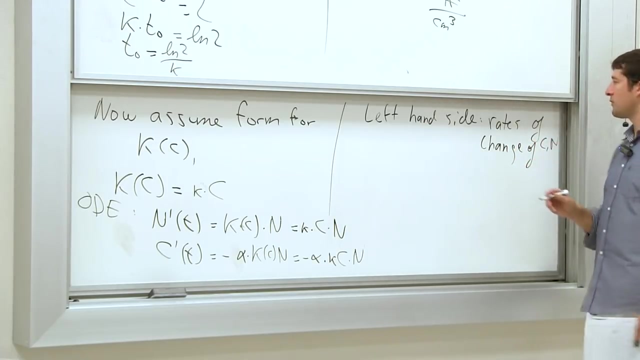 Kappa times C times n. all right now. Kappa times: C times n. all right now. notice that on the left-hand side are. notice that on the left-hand side are. notice that on the left-hand side are the rates of change, the rates of change, the rates of change for the two variables of the system C and. 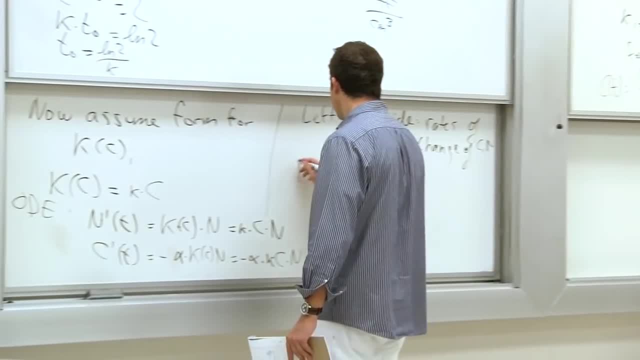 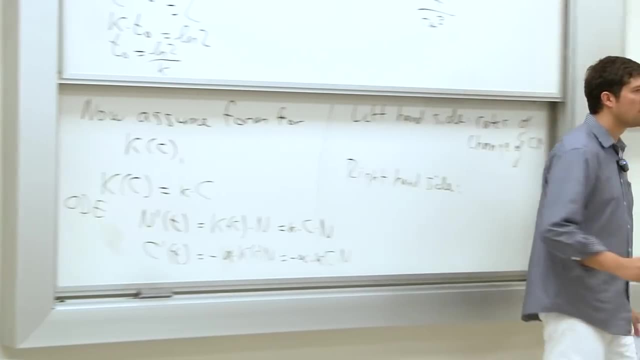 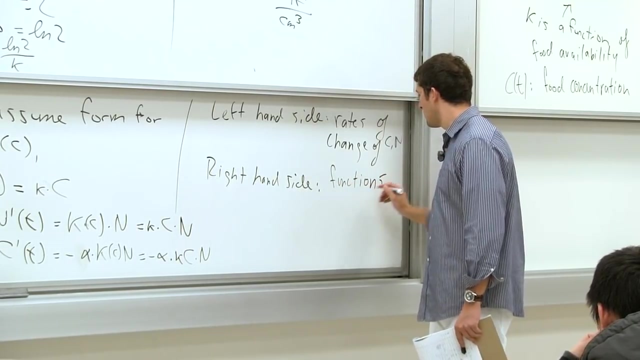 for the two variables of the system C and for the two variables of the system C and n. okay, and on the right-hand side we n okay. and on the right-hand side we n okay. and on the right-hand side we have functions of CNN. okay, what this? 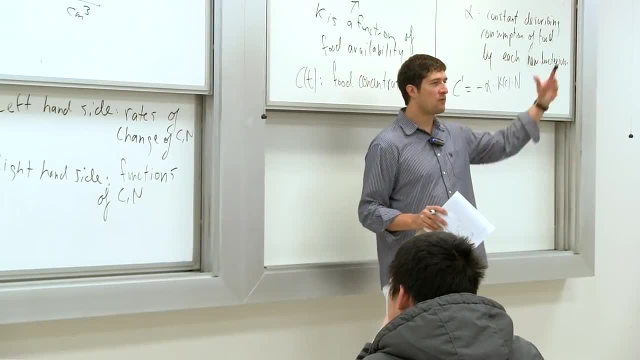 have functions of CNN. okay, what this have functions of CNN: okay, what this means is that if we know the constant means is that if we know the constant means is that if we know the constant ration of food and if we know the ration of food and if we know the 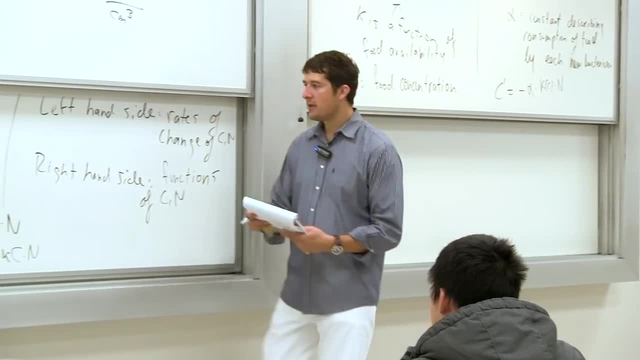 ration of food and if we know the population of n at any given time, then population of n at any given time, then population of n at any given time, then we can calculate the rate of change of. we can calculate the rate of change of. we can calculate the rate of change of the food and the population. that is the. 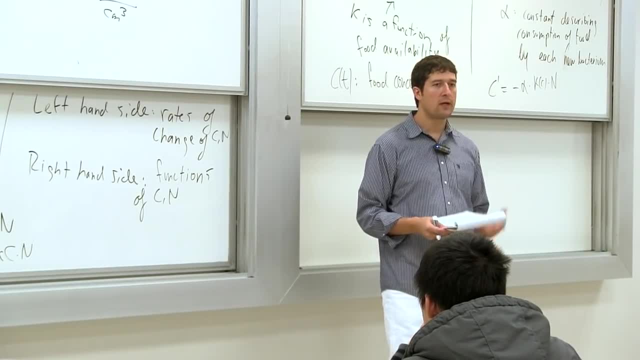 the food and the population. that is the. the food and the population. that is the key idea of dynamical systems. I said key idea of dynamical systems. I said key idea of dynamical systems. I said that's the basic situation for a. that's the basic situation for a. 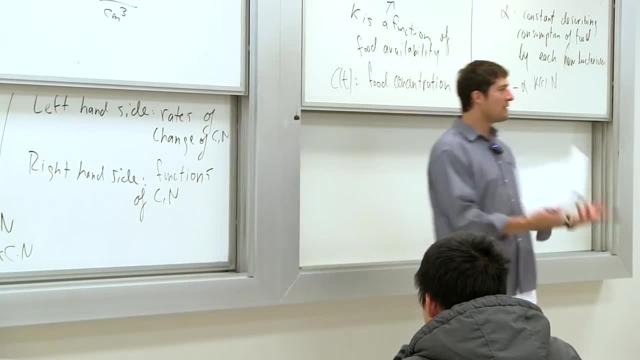 that's the basic situation for a continuous time dynamical system. is that continuous time dynamical system? is that continuous time dynamical system is that, if you know the state- in this case, food, if you know the state- in this case food, if you know the state- in this case food and population, you know the rate of. 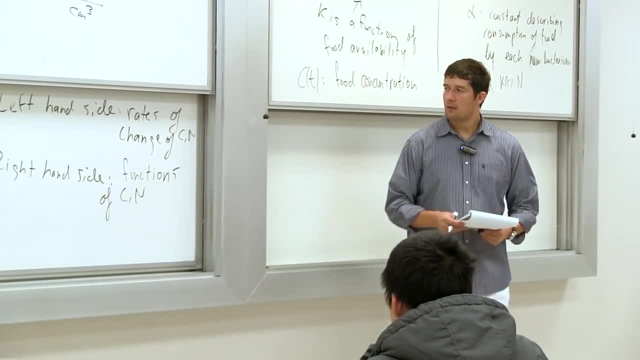 and population. you know the rate of, and population. you know the rate of change. okay, that's it. so this is an change. okay, that's it. so this is an change. okay, that's it. so this is an example of a dynamical system in this. example of a dynamical system in this. 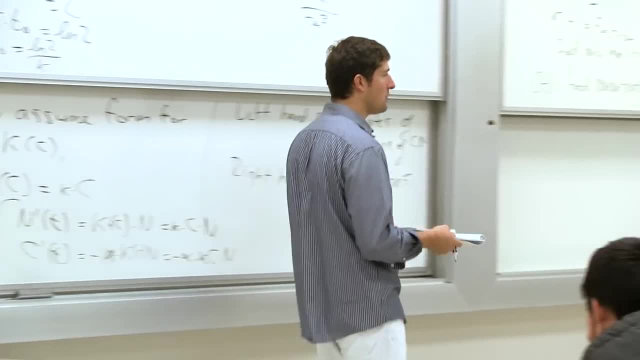 example of a dynamical system, in this case, a coupled system of two different case, a coupled system of two different case, a coupled system of two different equations and mathematically, now we can equations and mathematically, now we can equations, and mathematically, now we can use, you know, mathematical tools to 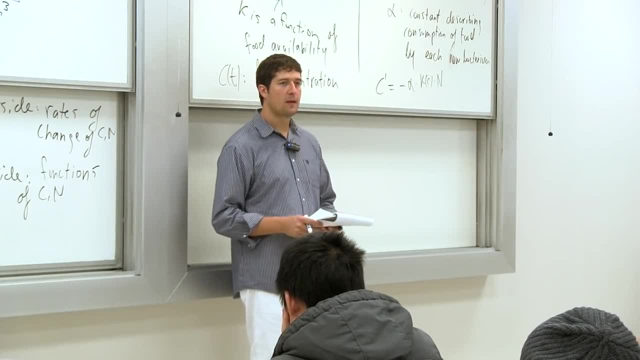 use you know mathematical tools to use you know mathematical tools to figure out how this thing behaves over. figure out how this thing behaves over. figure out how this thing behaves over time. all right, so you guys have any time. all right, so you guys have any time. all right, so you guys have any questions? 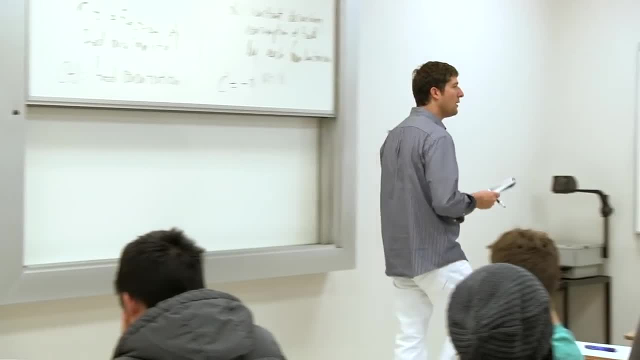 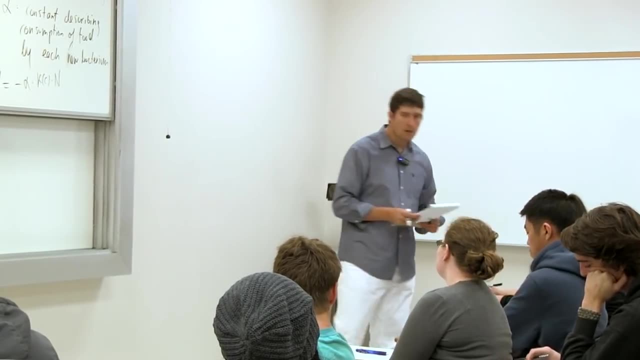 questions questions. yes, sir, okay, that's a very good question. when we? okay, that's a very good question. when we? okay, that's a very good question. when we make, when we are working on a make, when we are working on a make, when we are working on a mathematical model, how do we know when? 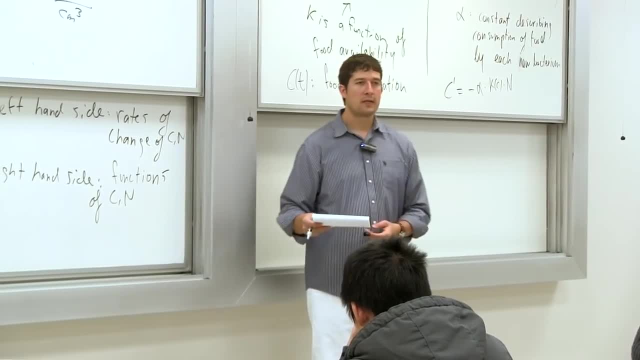 mathematical model. how do we know when? mathematical model. how do we know when to make assumptions and when these to make assumptions and when these to make assumptions and when these assumptions are reasonable, okay, and it assumptions are reasonable, okay, and it assumptions are reasonable, okay, and it really is a bit of an art. for example, 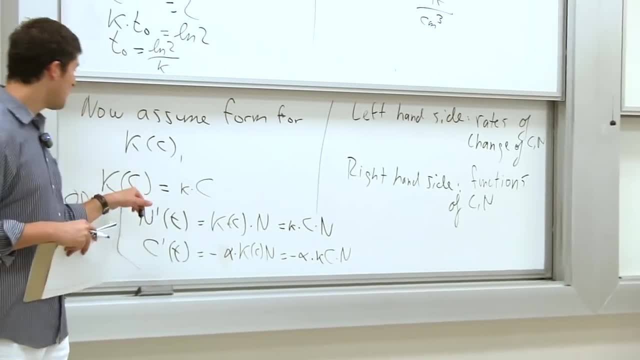 really is a bit of an art, for example, really is a bit of an art. for example: right here, we made a very well, we made right here, we made a very well, we made right here, we made a very well. we made an assumption about this function. we. 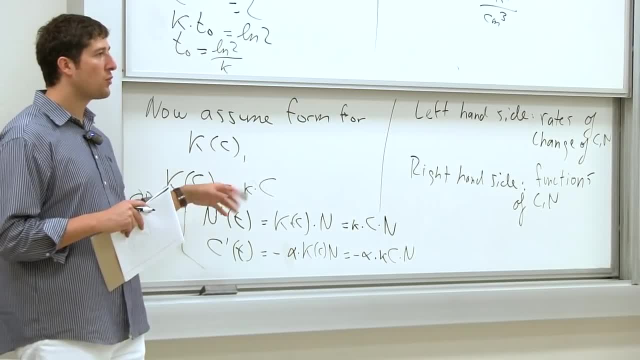 an assumption about this function. we an assumption about this function. we assume that it depends on the amount of. assume that it depends on the amount of. assume that it depends on the amount of food. that's because we wanted to we food. that's because we wanted to we. 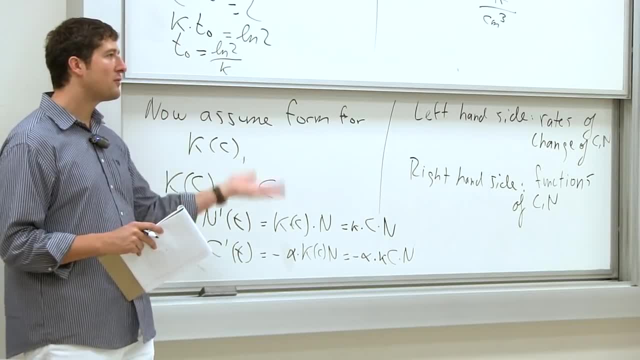 food. that's because we wanted to. we wanted to throw in food into the system, wanted to throw in food into the system, wanted to throw in food into the system. we wanted to say: you know the amount of. we wanted to say: you know the amount of. we wanted to say: you know the amount of sugar. really makes a difference. let's 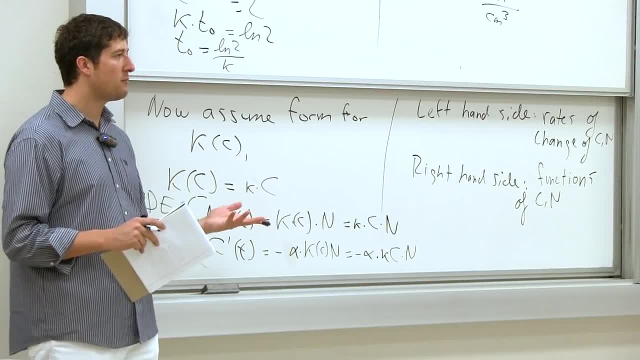 sugar really makes a difference. let's sugar really makes a difference. let's just let's throw sugar into the system. just let's throw sugar into the system. just let's throw sugar into the system and see how it how it behaves for how, and see how it how it behaves for how. 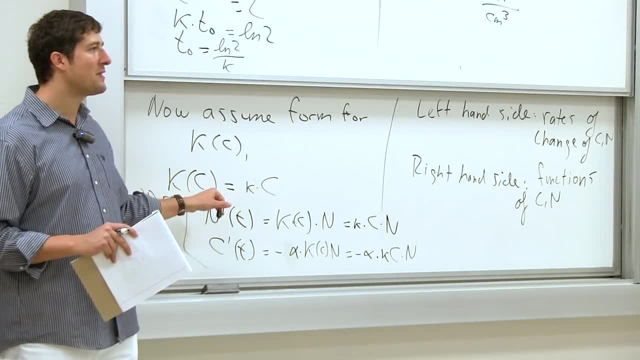 and see how it how it behaves, for how the whole thing behaves with sugar and the whole thing behaves with sugar and the whole thing behaves with sugar. and the way to include sugar into the system, the way to include sugar into the system, the way to include sugar into the system in this case is, let's say that the 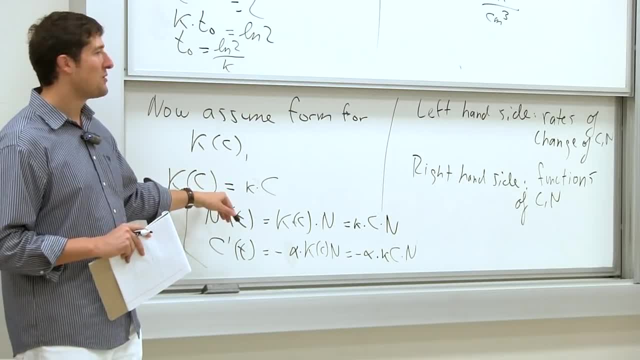 in this case is: let's say that the in this case is: let's say that the bacteria are happier the more food they bacteria are happier. the more food they bacteria are happier, the more food they have right. so that's how you made this. have right. so that's how you made this. 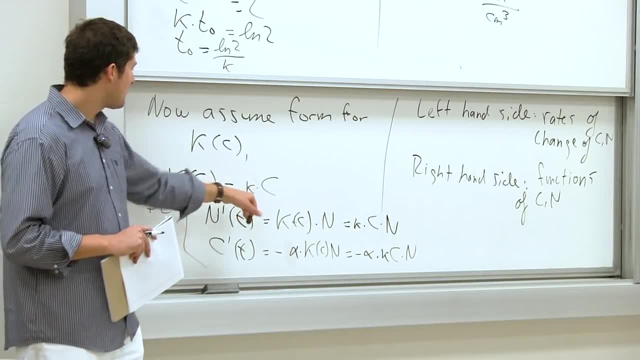 have right. so that's how you made this assumption about K being a function of C, assumption about K being a function of C, assumption about K being a function of C, then you have to figure out what kind. then you have to figure out what kind. then you have to figure out what kind of function of C, depending on what. 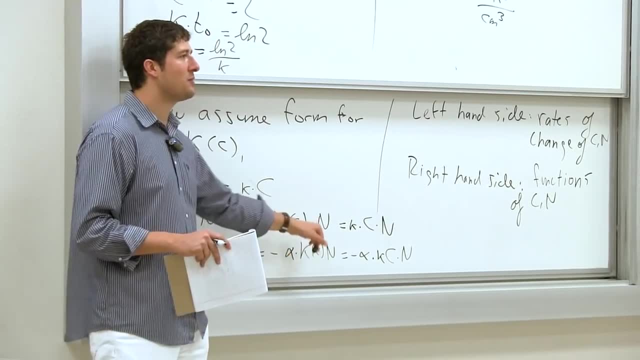 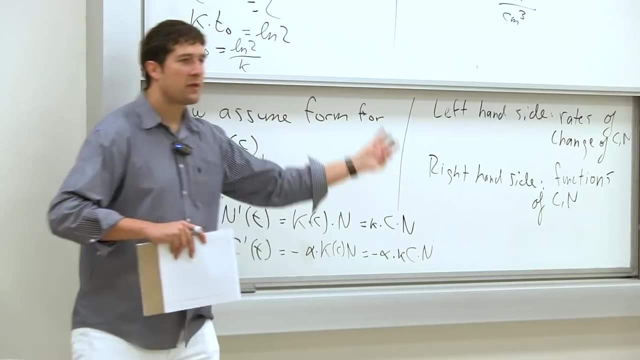 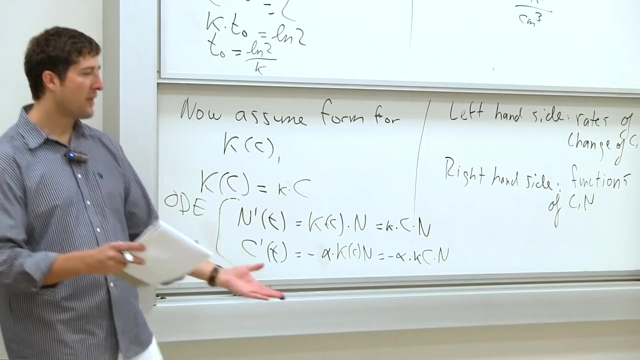 of function of C. depending on what of function of C? depending on what function of C you choose. you're gonna the function of C, you choose, you're gonna the function of C you choose, you're gonna problem. the modelers art is on the one problem. the modelers art is on the one. 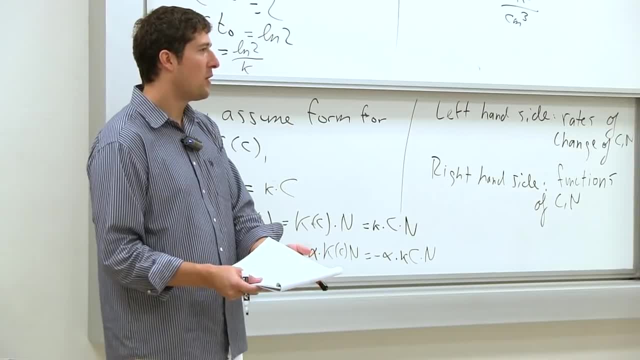 problem: the modelers art is on the one hand side. you want to make us, you want hand side. you want to make us, you want hand side. you want to make us. you want to make. be as precise as possible on the. to make be as precise as possible on the. 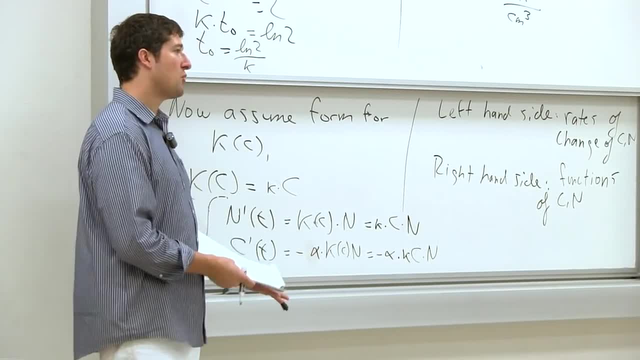 to make be as precise as possible. on the other hand, if you make it too messy, and other hand if you make it too messy, and other hand, if you make it too messy and too precise, you're not gonna be able to, too precise, you're not gonna be able to. 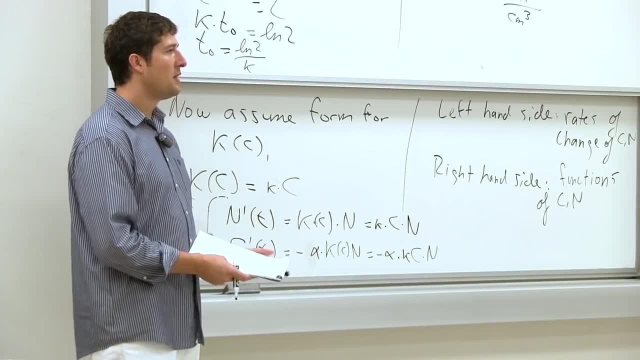 too precise, you're not gonna be able to analyze it because it's gonna be too analyze it because it's gonna be too analyze it because it's gonna be too difficult to solve mathematically first. difficult to solve mathematically first, First of all. second, you have more and more parameters. 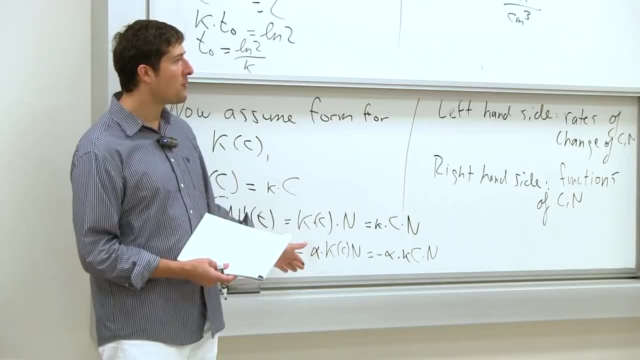 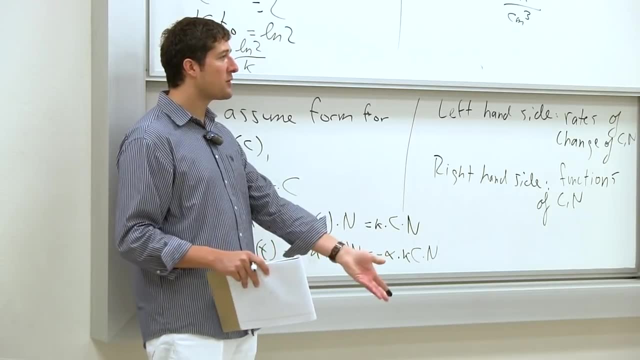 These parameters are going to influence the system. Depending on the value of the parameter, you're going to get one behavior or a different behavior and bottom line is we don't really know those parameters. You can talk with a biologist to figure out the parameter values and sometimes you're 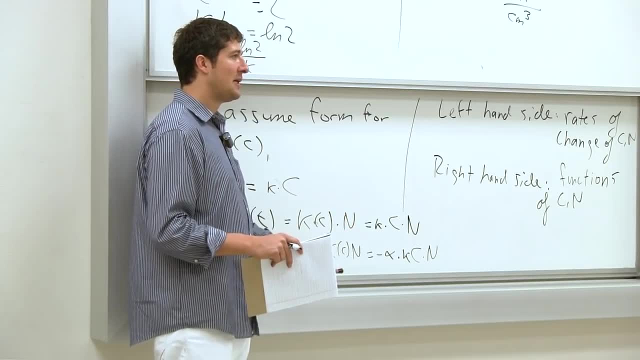 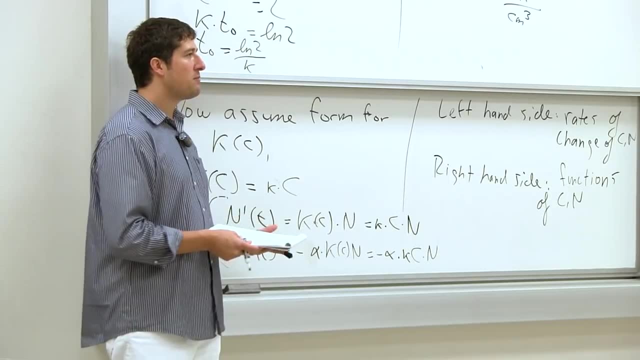 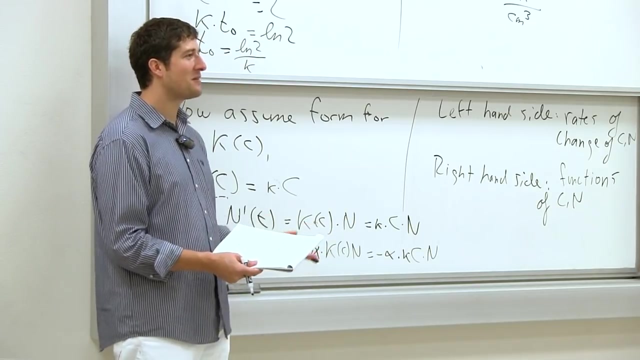 going to be able to derive those parameter values from experimental data. But the fewer parameters you have, the better off you are. Somebody also said about modeling that if they're given enough parameters- like a hundred parameters- they can feed an elephant. They can feed anything you give them, they can feed. 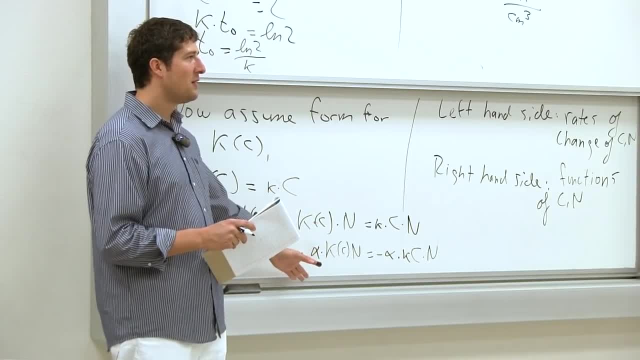 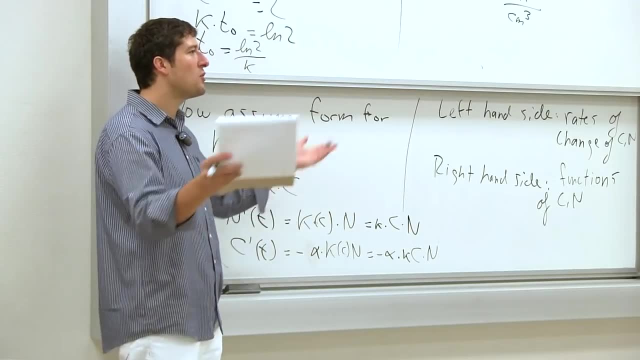 This is this idea that you can cheat with parameters. The more parameters you throw in, the more chances you have to feed things however you want, and then you can choose parameters to do whatever you want to do, but you're still not doing anything particularly useful, necessarily. 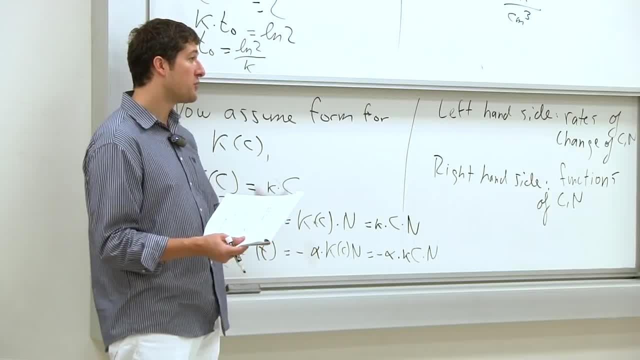 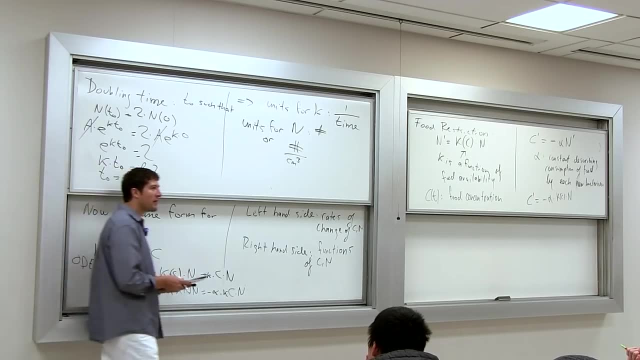 We want to keep it as simple as possible so that we can analyze it And we're not cheating with parameters, But, on the other hand, we want to include the interesting biology And in terms of mathematical biology, which is different from other types of modeling. 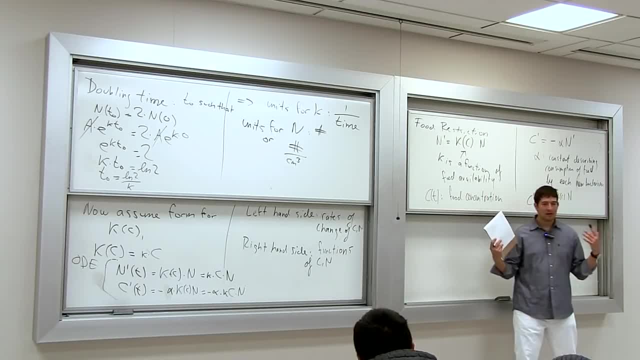 if you're modeling physics or if you're modeling engineering problems, if you're modeling the flow of air through an airplane or if you're modeling how a ball is thrown. you can always make simplifying assumptions and you can find an environment where the assumptions 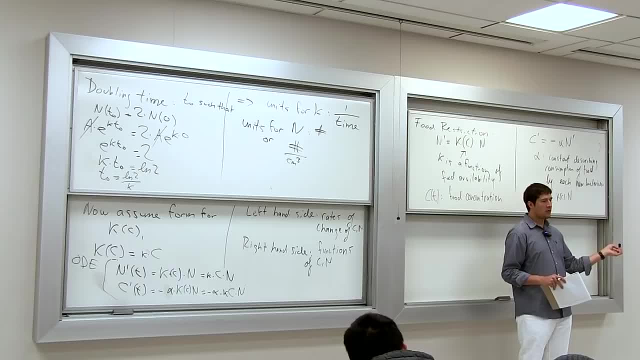 are broadly satisfied. For example, if you don't want to use, If you want to throw a ball and you don't want to take into account friction with the air, you can throw the ball in vacuum. I mean, it's hard right. 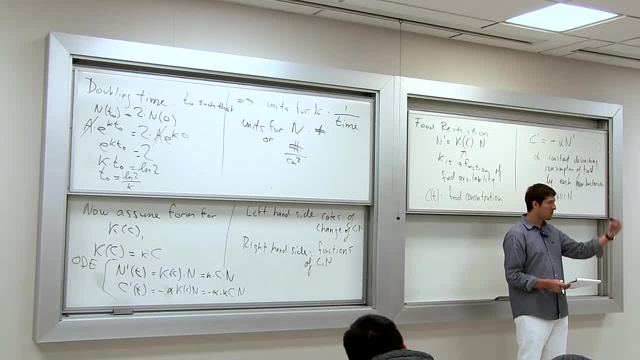 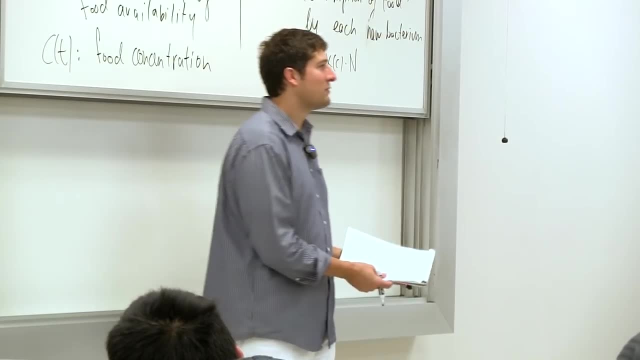 But you can. You can do that And you can verify this assumption of what happens if you throw the ball in vacuum. Does it really satisfy with what you want? But you cannot just assume that a bacterium doesn't need sugar, right? 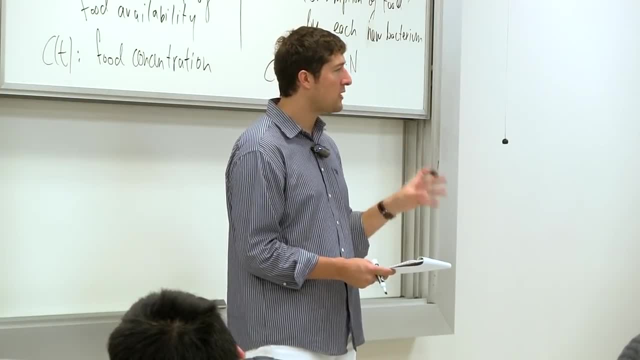 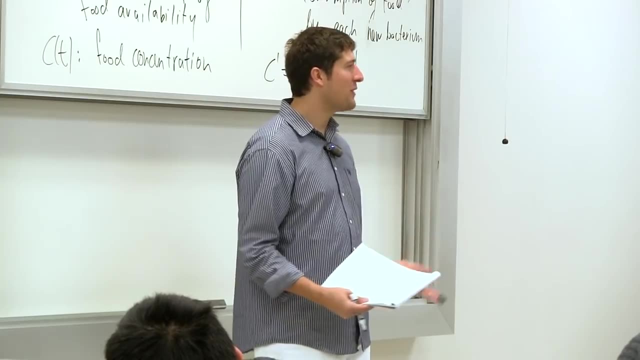 You cannot change Nowadays. sometimes you can, but generally you cannot change the biological system to satisfy your simplifying assumption, right? So the problem with biology is that it's very, very messy and you have to deal with that messiness, if you will, right. 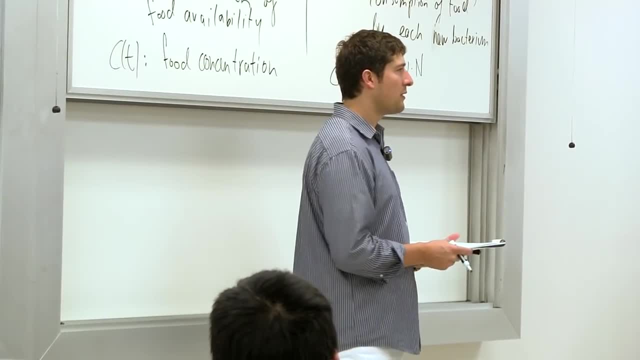 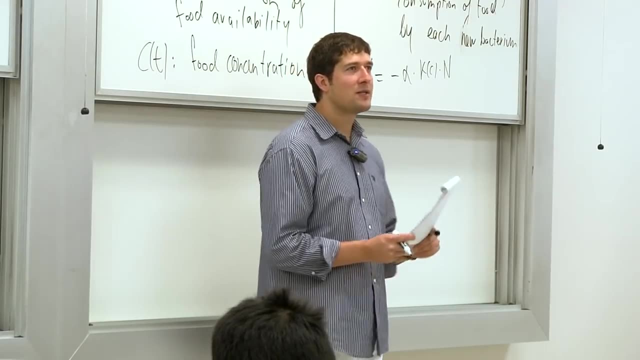 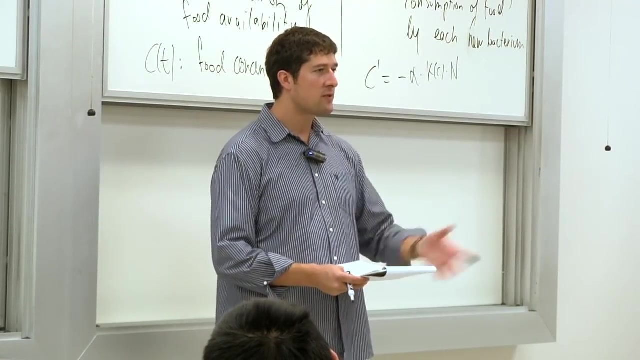 So that's why modeling in biology is a little bit different from other types of modeling. Any other questions? All right, so we're running out of time. So next time we're going to continue with this system, We're going to solve it and we're going to make it a little bit more complicated, and